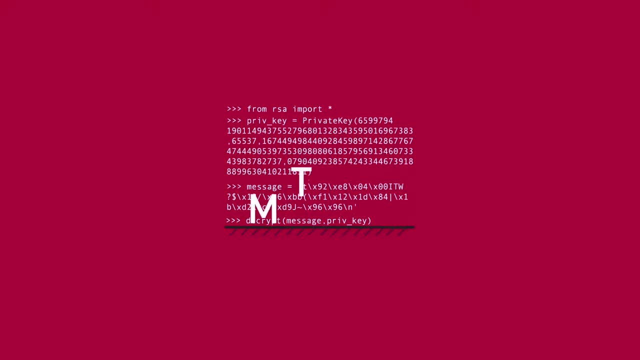 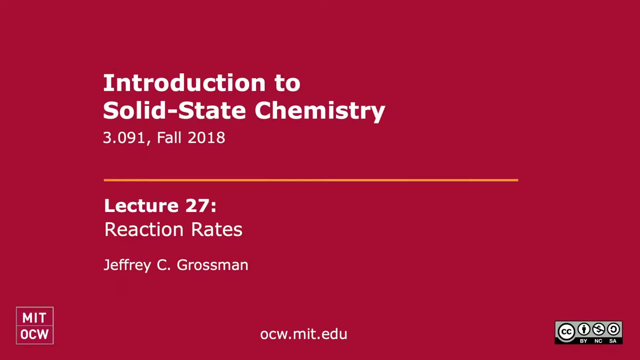 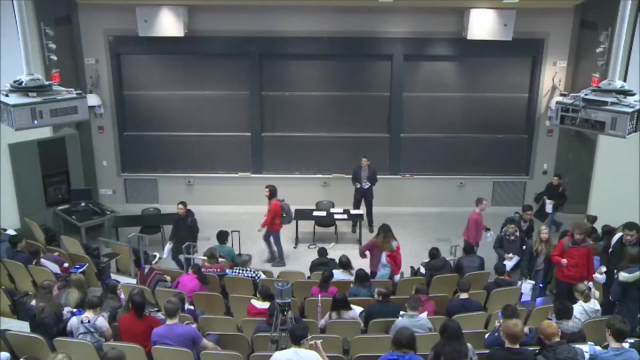 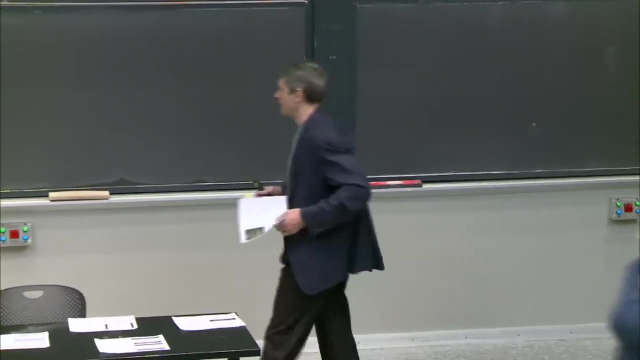 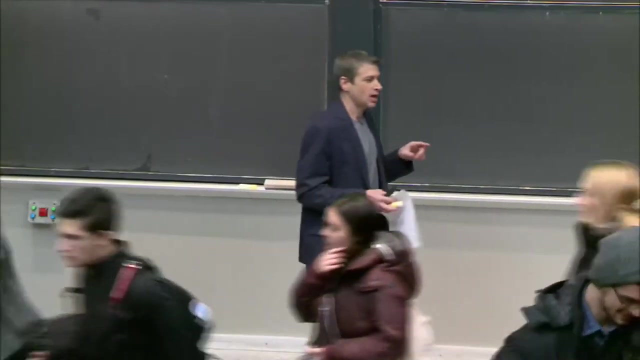 How's everyone doing? It's a goody bag. It's thank you for that. It's a goody bag day. It's a good day Related to the goody bags, you know, once again, hello. Once again, I want to get. 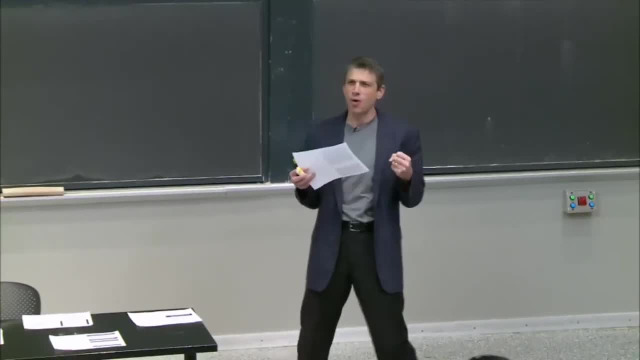 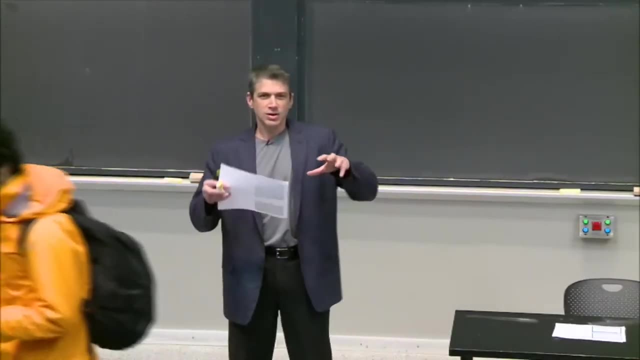 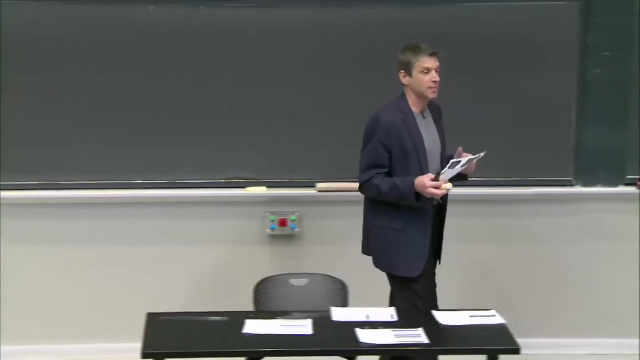 these out for you because you got to have them on a Friday night. There's no real better way to think about spending your time on a Friday night than opening up a brand new goody bag. The topic of the goody bag is related to reactions, which is the topic we're starting today, but it's really 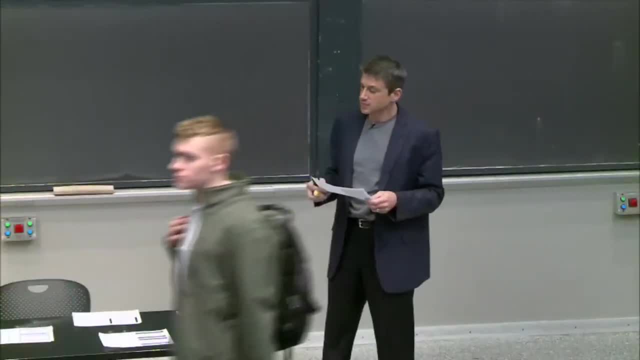 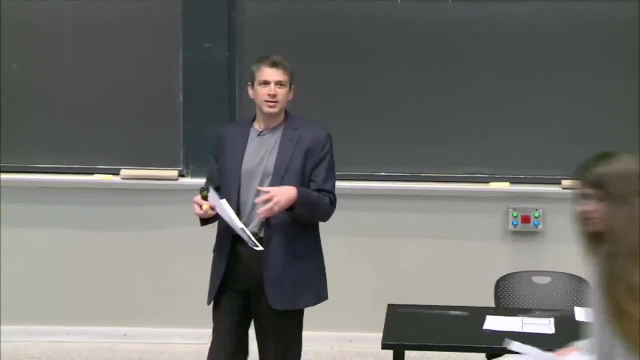 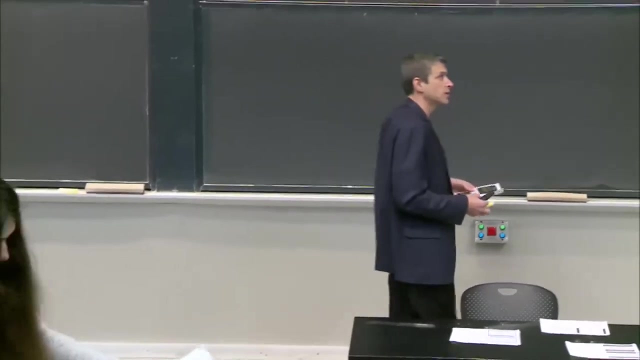 also related to acids and bases, which is something we'll talk about on Monday. So I'm giving you the goody bag today, but I'll talk about the goody bag and contextualize it in the lecture on Monday. But, as I said, today what we're going to do is we're going to start a new topic that we'll be 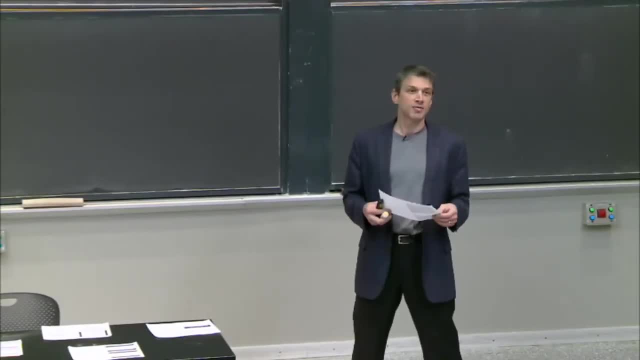 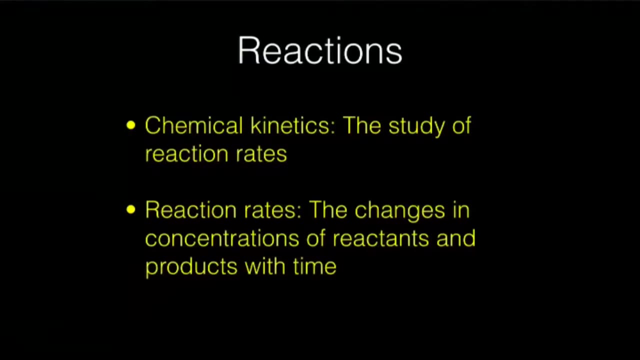 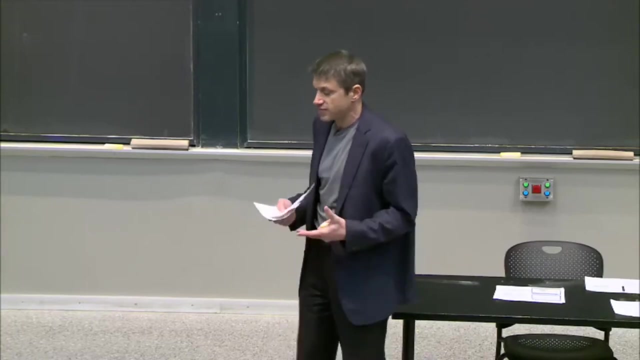 talking about for the next couple of weeks, and that is the topic of reactions. Okay, now this falls under the domain of something called chemical kinetics, which is the study of reaction rates. Kinetic: move right. So what's moving? Concentration: right, The stuff that you started. 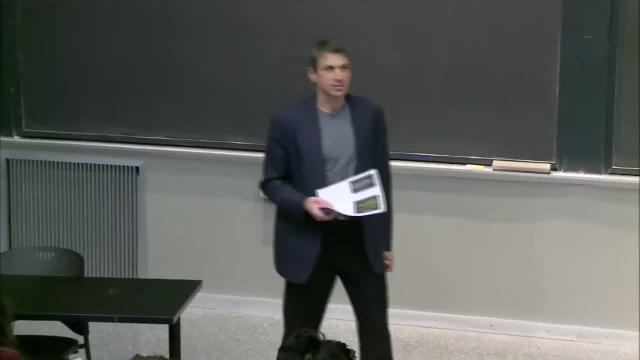 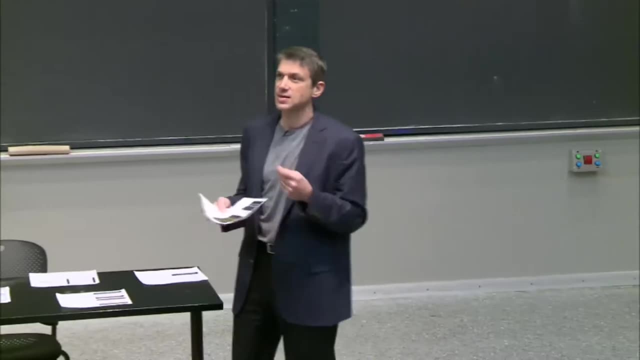 with is doing something and winding up different. That's a reaction. okay, Now, we've already written lots of reactions in this class, but today we're going to talk about the rates, And the rate in particular is the change in concentration of the reactants and products with. 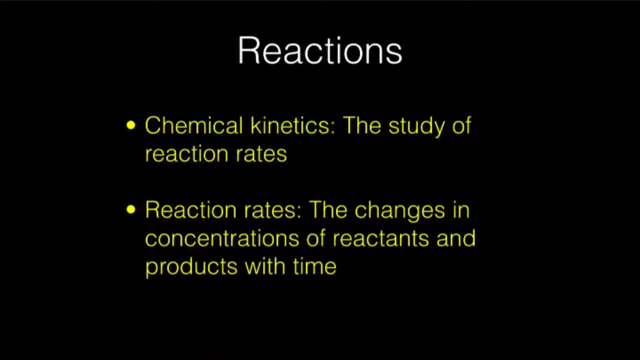 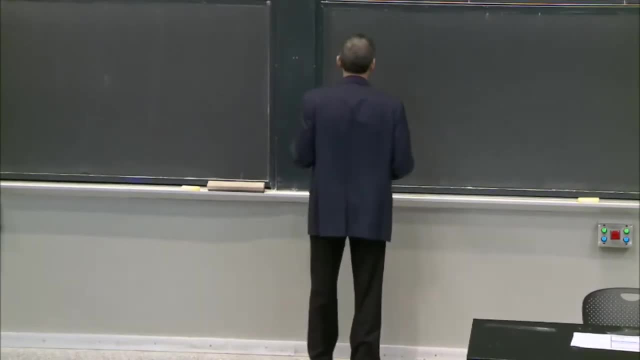 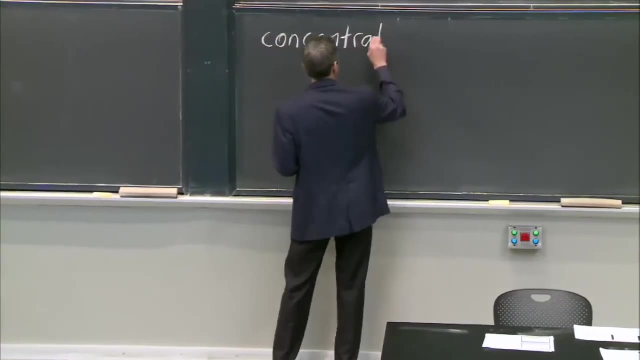 time. So there's a couple of terms that we got to know because we're going to be working with them, and so I'm going to start by writing those down. Okay, so the first thing is the thing that we're going to talk about changing, which is the concentration. Okay, so the concentration is equal to. 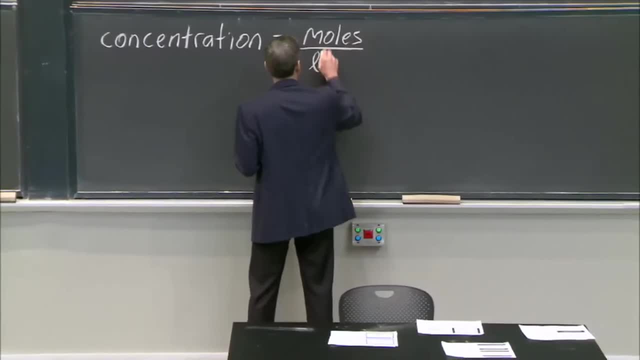 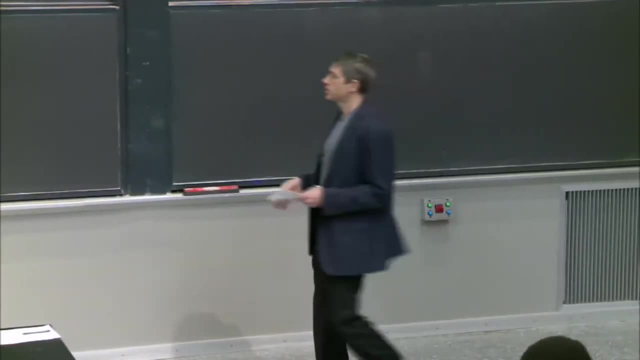 the moles per liter. I mean there are lots of ways to write concentration, This is the way we're going to write it- Moles of a substance per liter. Well, that has a name for it. That's called the molarity. 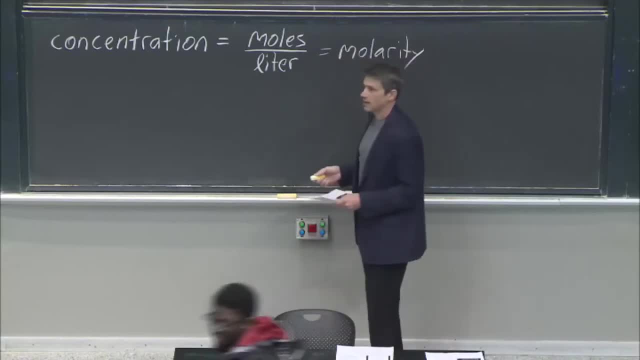 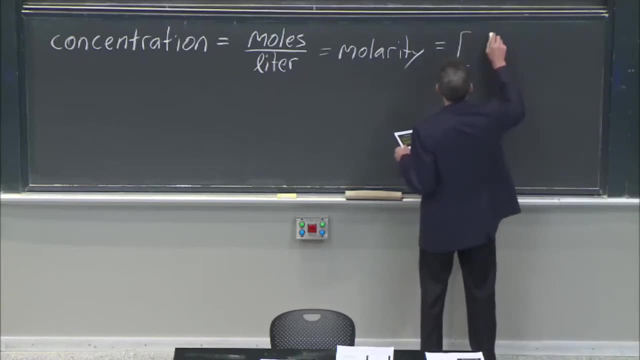 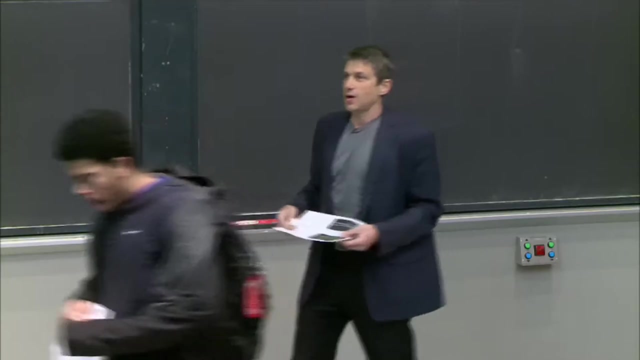 What's molarity? It's moles per liter, And oh, and then we can also write it in shorthand, which I'll be doing, as simply some substance in brackets. If I say that I have some substance A and I say: and now I say oh, 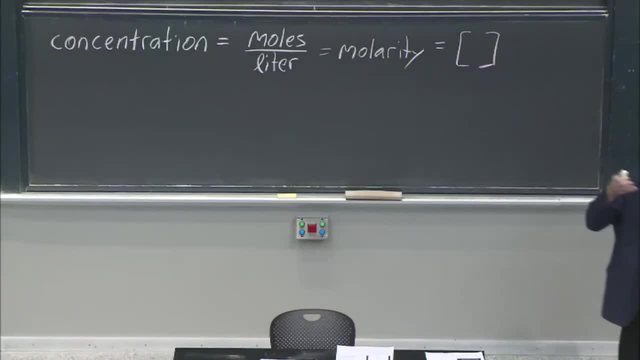 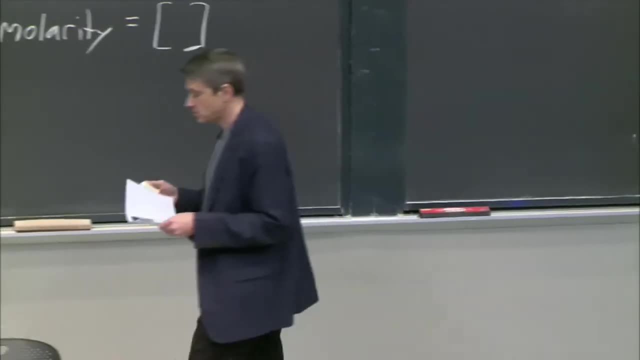 look, I'm writing brackets around it. then what I mean is the concentration of A. That's what that means, which is the moles per liter of A Good, so that's concentration. What else? Well, there's the rate. 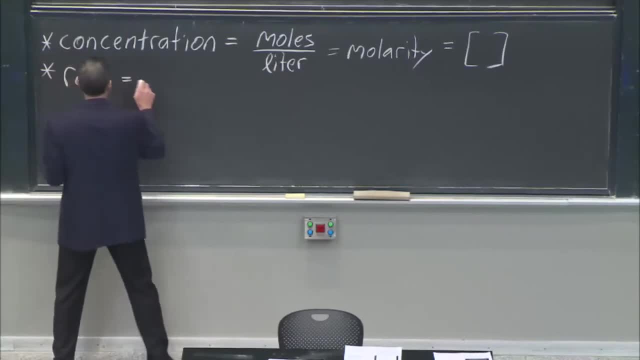 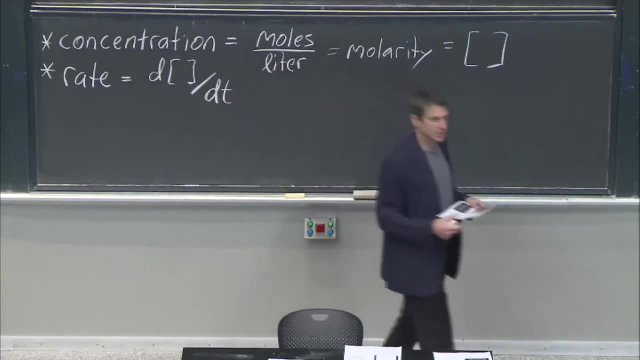 There's the rate, And the rate is, as you might guess, the change in the concentration with time. That's the rate that we're going to be talking about a lot today. the reaction rate: There's a change in the concentration with time. 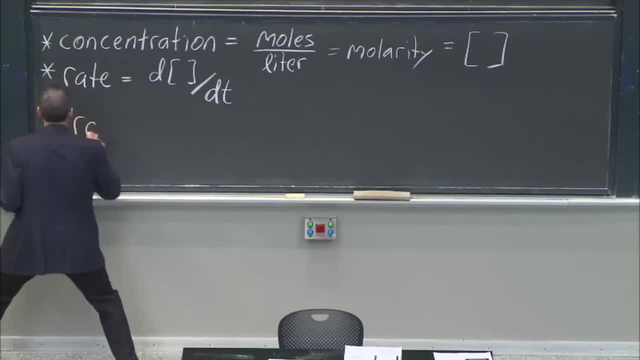 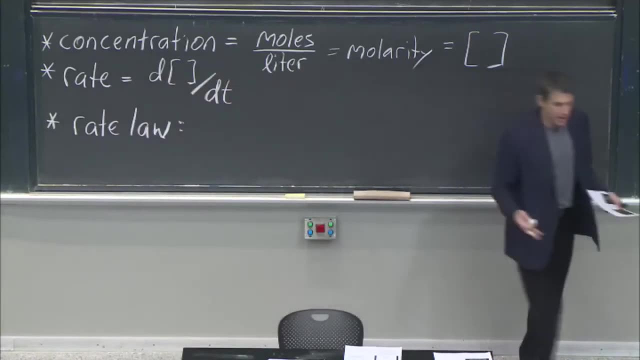 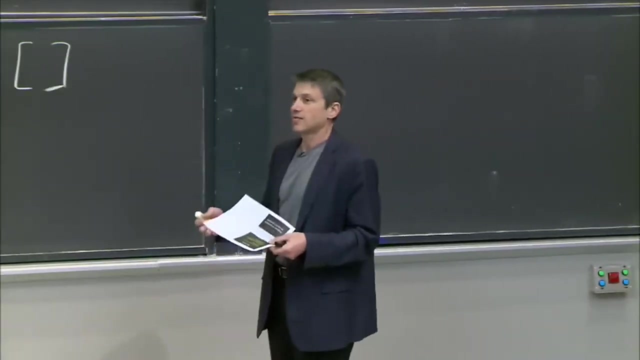 What else do we got? Well, we have, then, a law, Because see, here's the thing, The rate is just the rate, It's the change with something with time. It's like the change in distance with time would be like velocity. 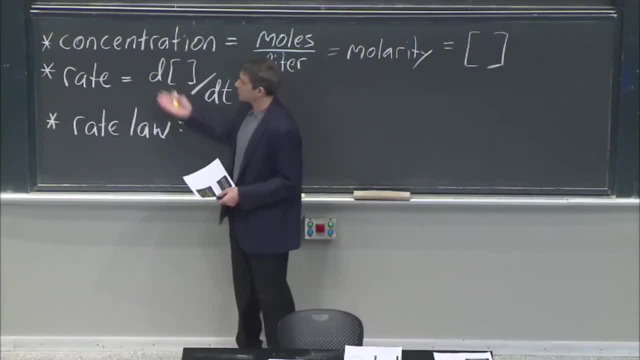 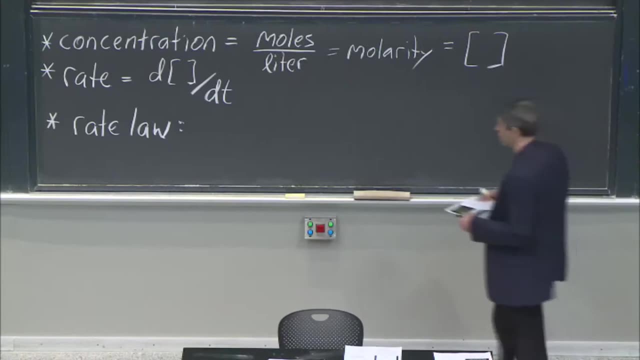 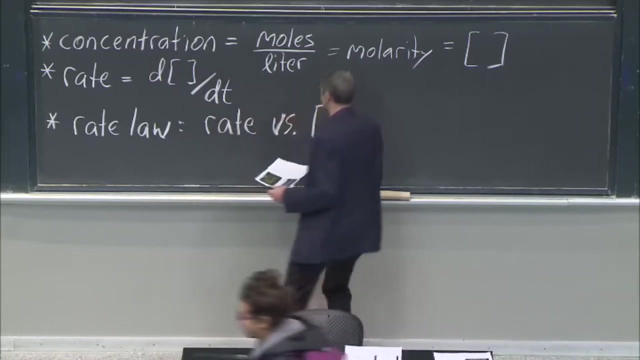 But what if I wanted to say: well, could you tell me what the rate is, as some function, As some function, That's good, That's called a rate law, That's called a rate law, And it will give me a rate versus concentration. 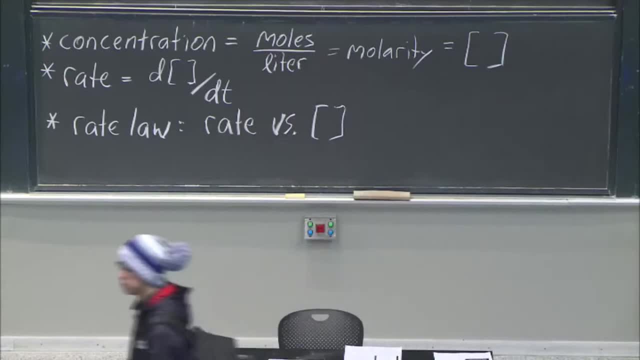 That's what I want out of a rate law. And then, well, I could integrate that. I could integrate that because the rate itself is a derivative with time. It's a change in time. So if I integrate it, well then I've. 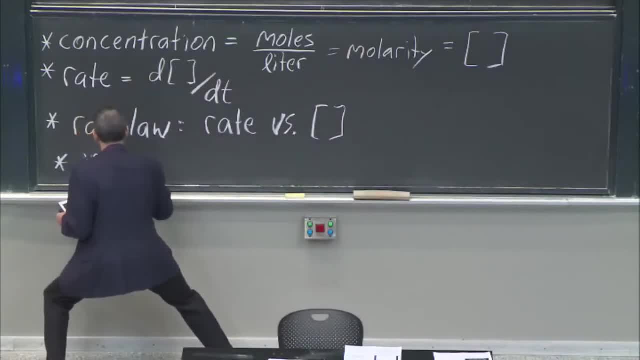 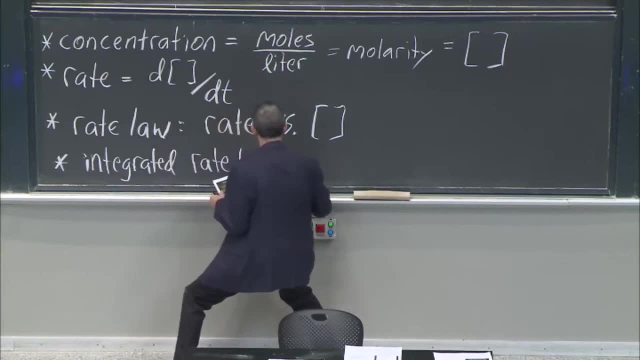 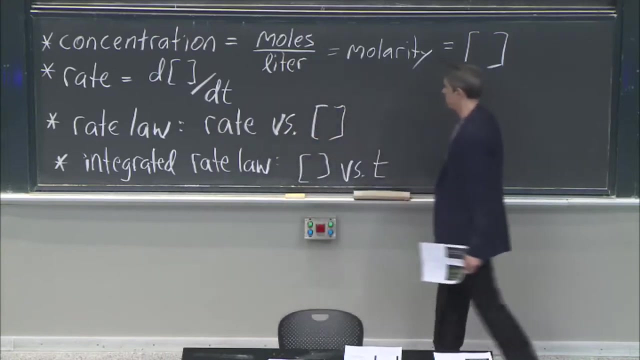 got something called the integrated rate law- Integrated rate, Integrated rate law- And what's that going to give me? It's going to give me the concentration versus time, Because the rate law is a rate versus concentration And the integrated rate law is the concentration versus time. 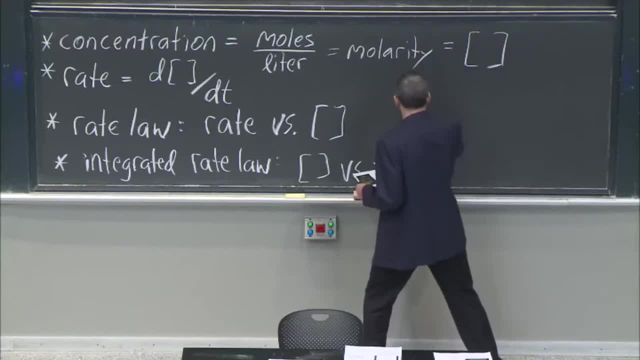 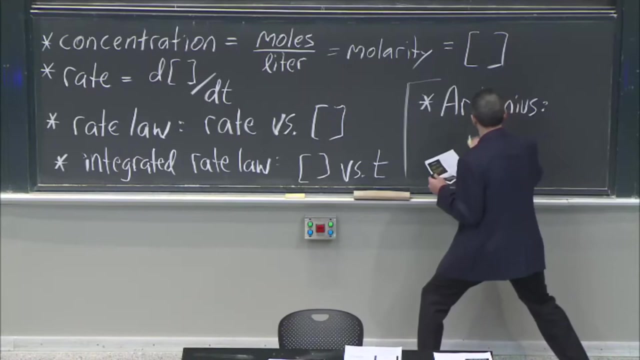 And then we've got Arrhenius. Let's put it all on the same board. So I'll do one more here, which is the Arrhenius dependence. It's going to give me the concentration for reactions And, as you might guess, this is going. 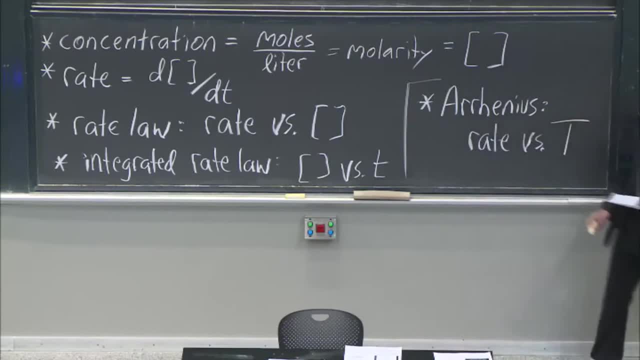 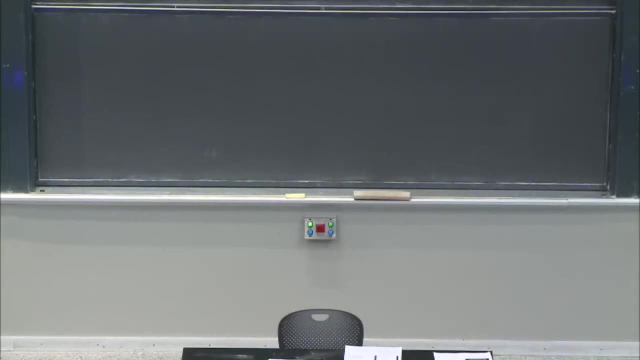 to give me rate versus temperature. These are the things we're going to be talking about. All these things we're going to talk about today in the context of reactions. I wanted to get them all down on the board so you can see them and think about them, and feel them. 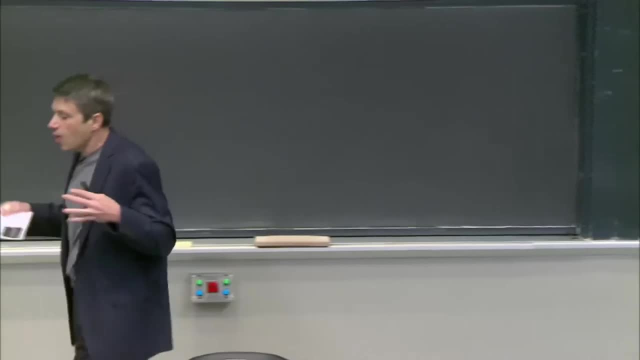 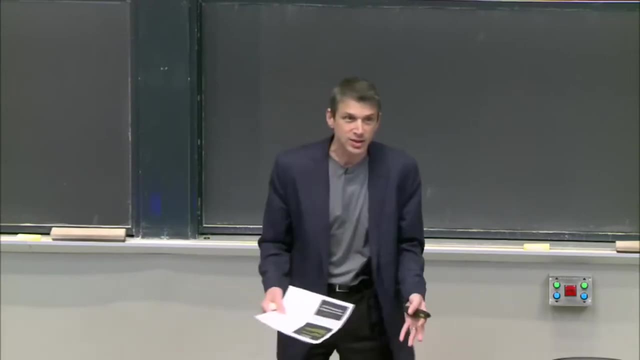 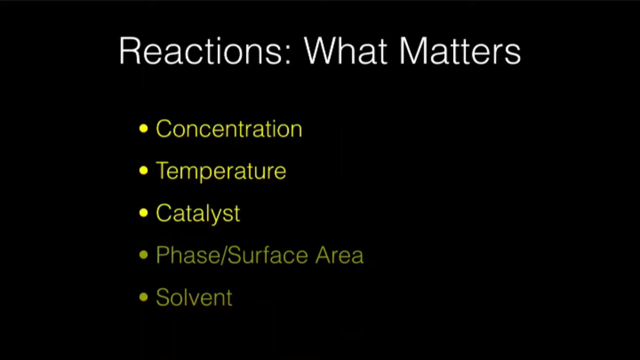 forward. So there are a whole bunch of things that impact the reaction, the rate of a reaction. What is it that matters? Well, concentration, How much do you have? That's the brackets thingy. Temperature catalysts, the surface and the structure. 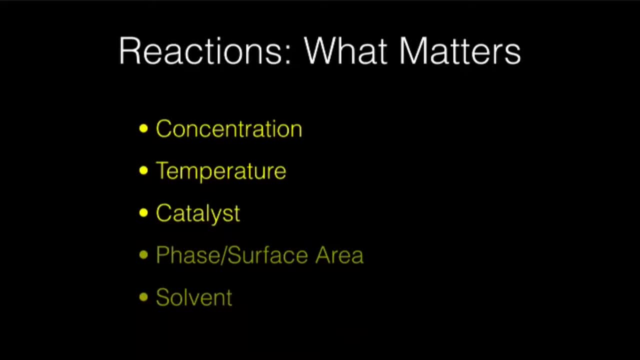 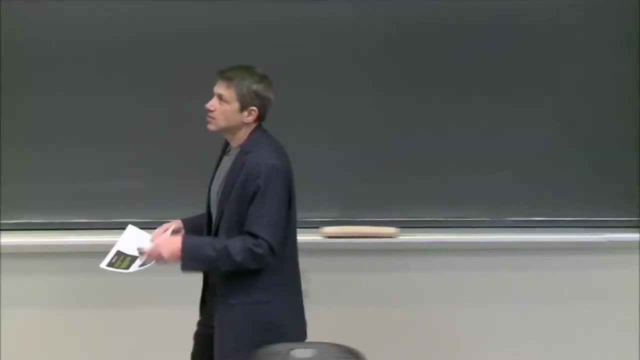 that you're doing, the reaction on the solvent that it's in. All of these things impact how the reaction happens And you see, I'm going to grayed out and made a little darker those bottom two because I'm not going to talk about those two. 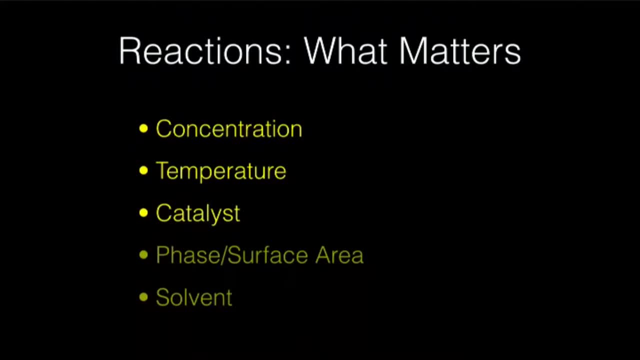 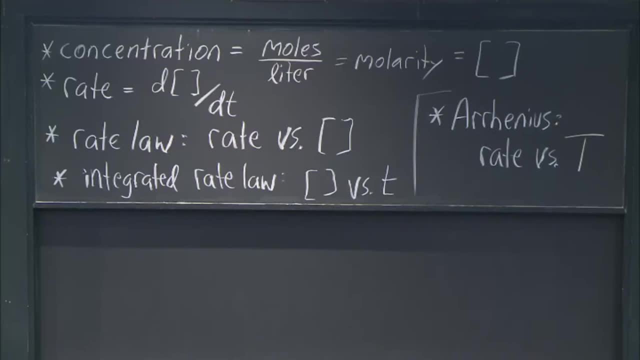 But I will talk about each of those other items today. That's our goal. How do those items play into these dependencies? That's our goal is to figure that out. So we're going to start with concentration And we're going to talk about how concentration plays. 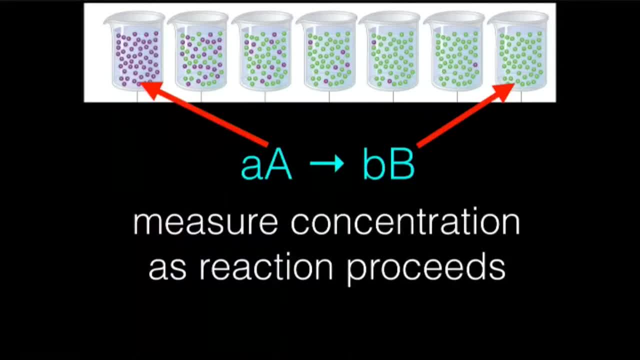 a role in reaction rates, And we're going to start with something very simple. I have something called A- Oh it's purple, And it turns into something called B- It's green. There you go, There's a reaction. OK. 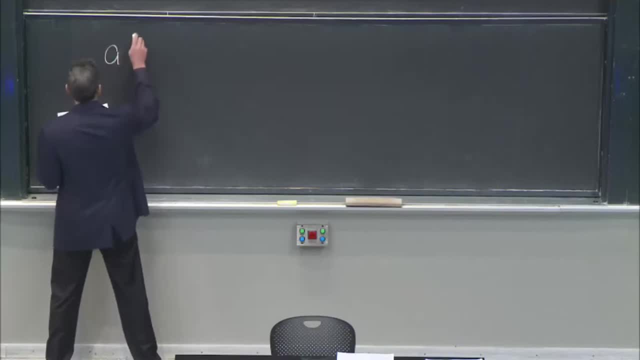 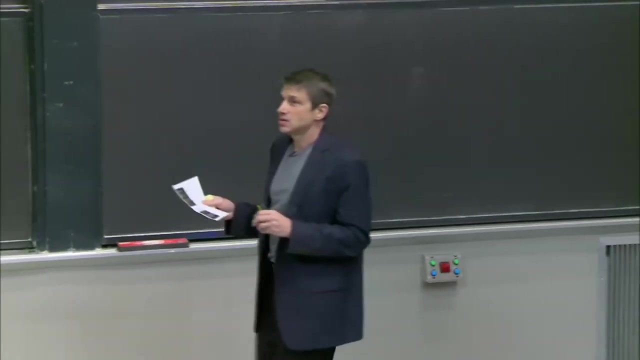 So let's start now. OK, So A A goes to B, B. Now the very first thing that I can think about in this is that nothing is lost. Nothing is lost, So I'm going to assume that nothing disappeared from my container. 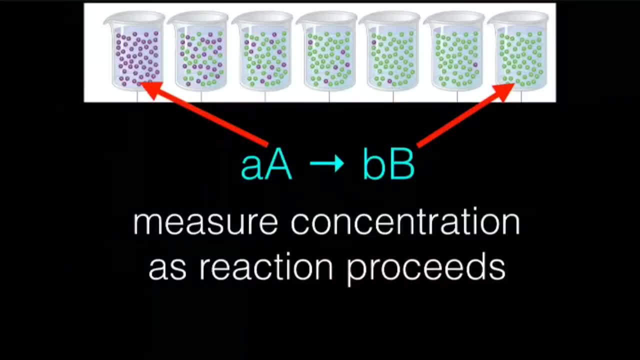 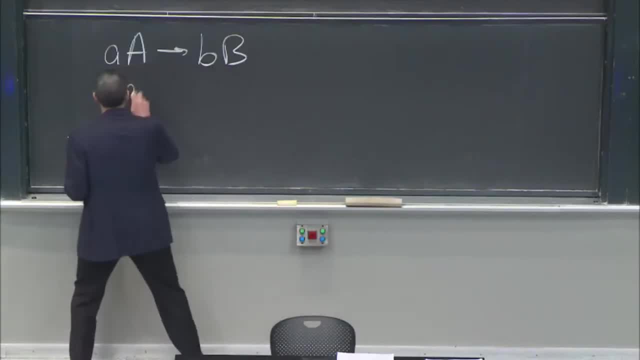 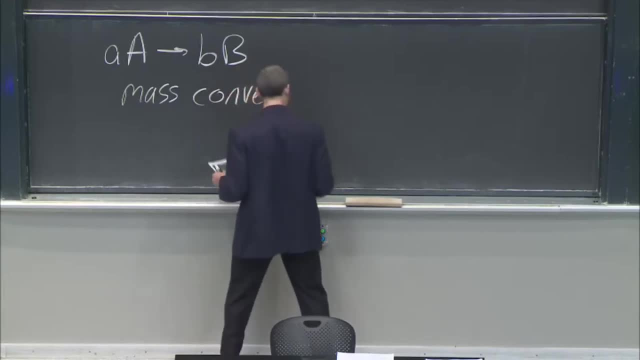 You see that The container, The container is there. So I haven't lost any mass. I haven't lost any mass. Well, mass conservation is a big deal, right? So mass conservation by taking this very simple case, mass conser, oh really. 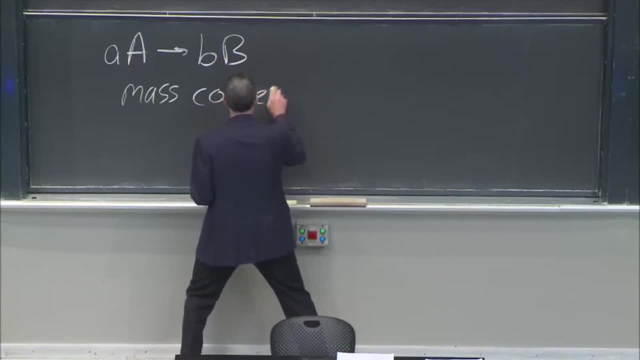 We could have a mass conversation too. That's OK. That's kind of what we're doing, But let's write it as conservation. This means that if I take away A Now, I must add B with the same amount and not lose anything. 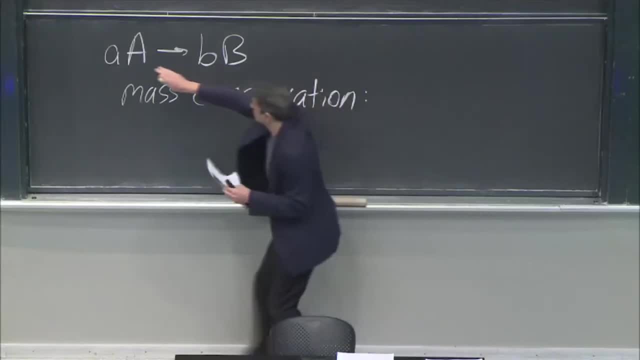 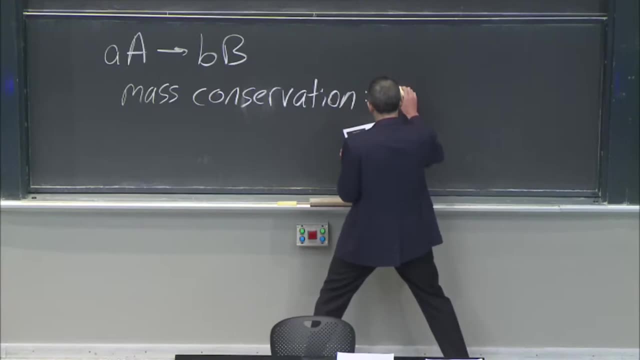 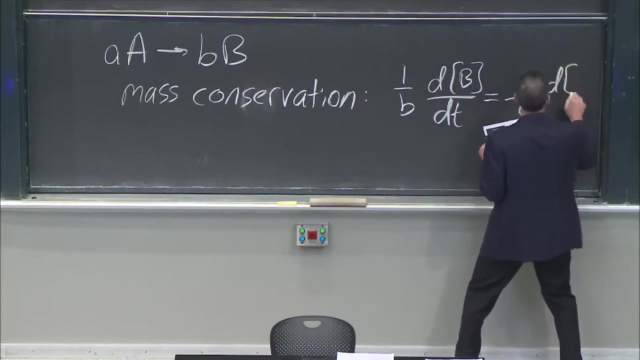 And if you look at that in terms of these coefficients- remember these are stoichiometric coefficients as part of the reaction- Then what that means is that 1 over B times the change in the concentration of B with time must equal minus 1 over A times the change. 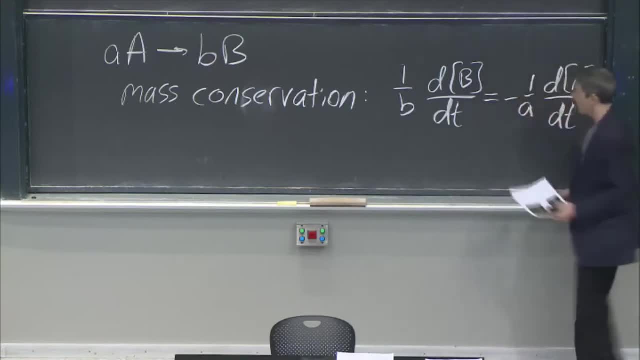 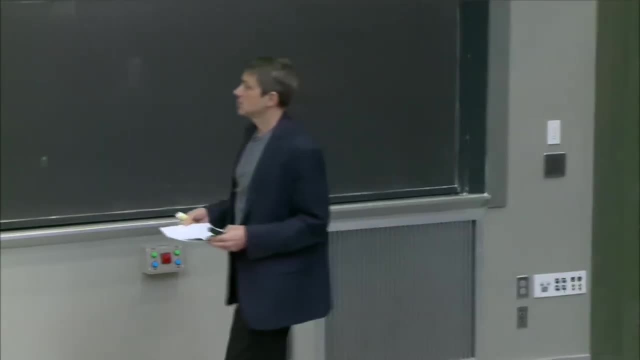 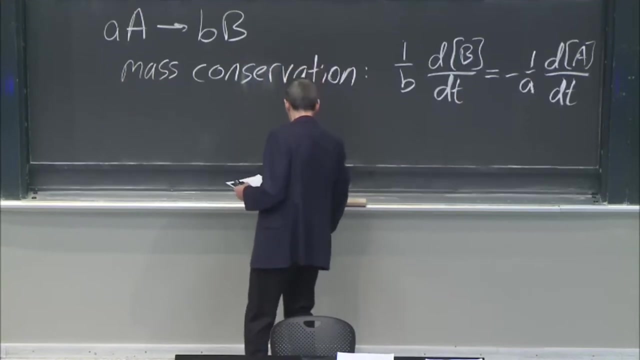 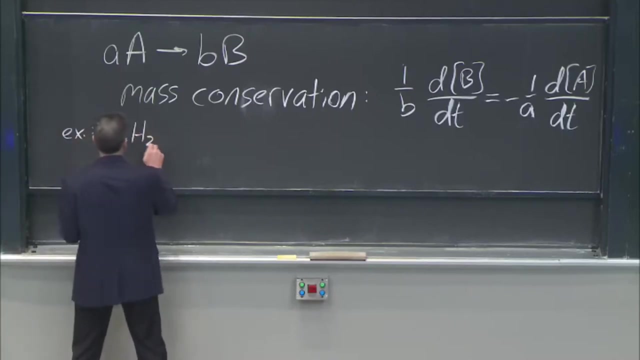 in concentration of A with time. That is mass conservation, just written as changes in concentration. Now you can see it. Look, imagine that this is 1, just as an example. OK, 1H2 goes to 2H, right? 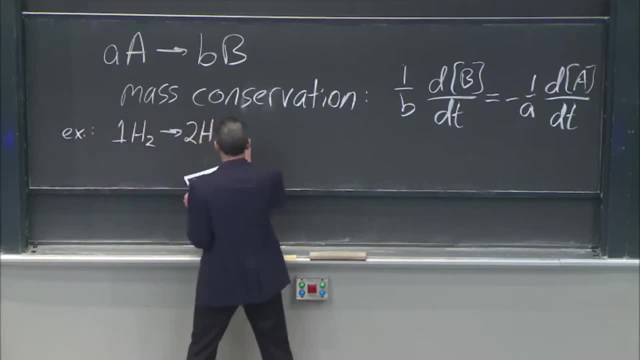 I'm not going to lose anything. Those are my stoichiometric Well. OK, this would tell you that the rate of this, if I don't lose anything, would be 1: half the change in H, the concentration of H with time. 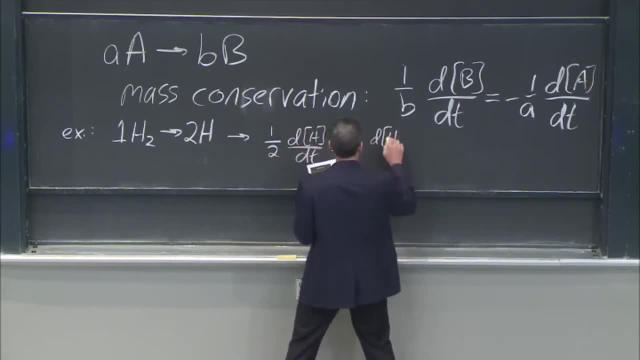 equals minus the change in concentration of H2.. That's just exactly what I wrote, but with an example I didn't lose anything, right? So the rate of change of this must be twice the rate of change of that. Right Stoichiometric coefficients come in. 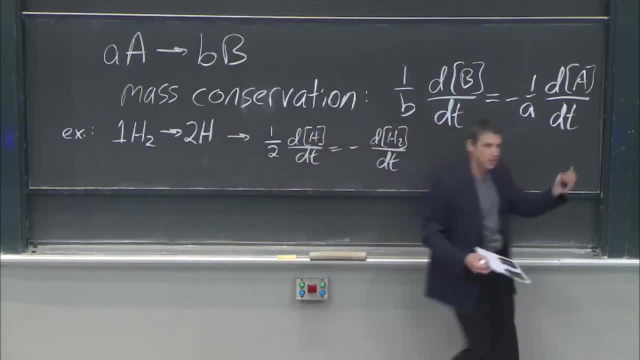 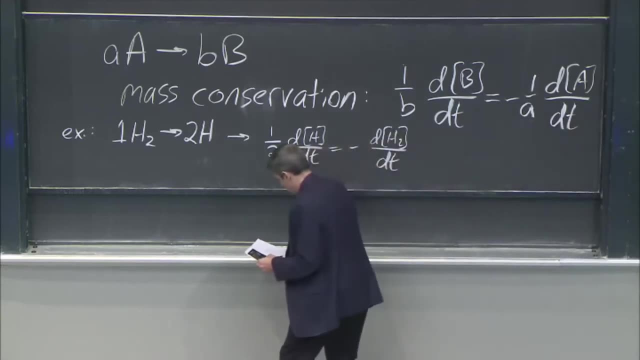 And they make sure, when I write it this way, they make sure I don't lose anything. That's why you've got to have these there Now. there's a couple other things about this, right, There's a couple other things about this. 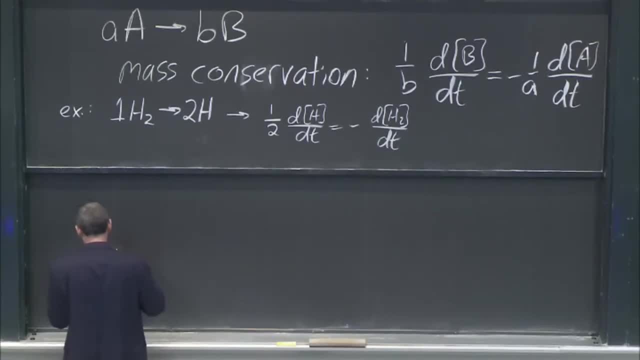 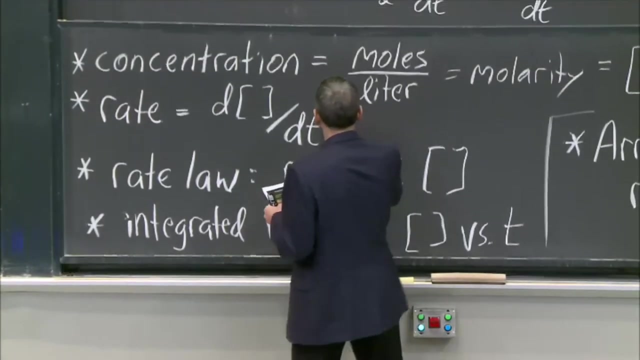 One is that you'll notice that the rate is always positive. Maybe we should write that up on the top board because it's a convention, But we like positive numbers when we talk about rates. So the rate is always positive. OK, always positive. 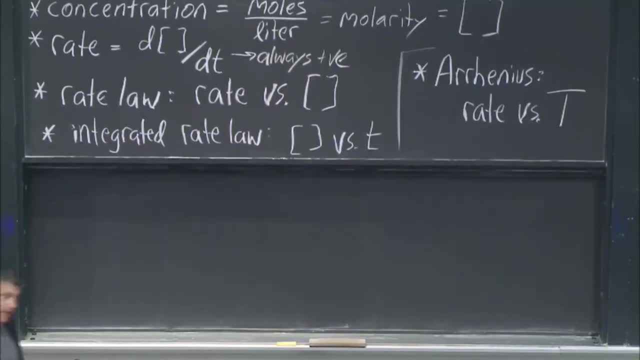 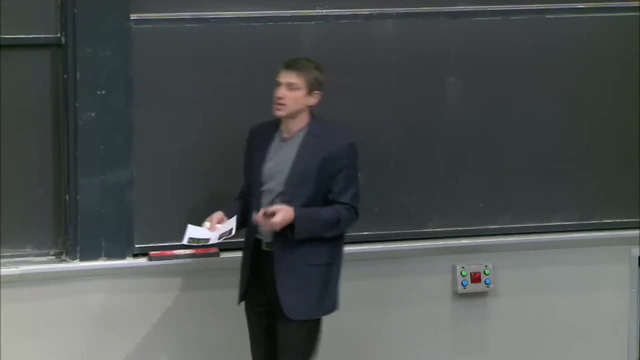 So when we're thinking about a reaction where something's getting consumed, we're going to write it as the negative of the change in that concentration, because that's a negative, And then we're going to write it as a positive of the change in concentration of things being formed. 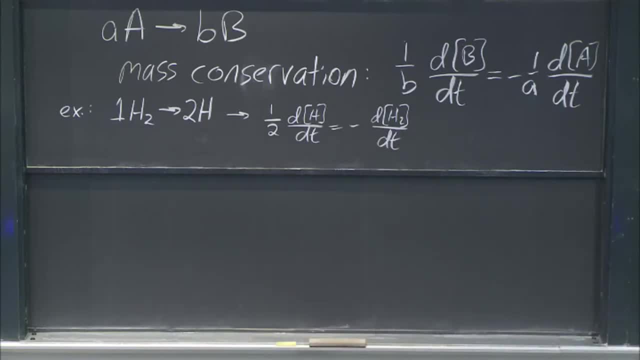 OK, So the rate is written, It's written as positive. Well, there's another thing, which is we can go more general. So let's just think about this: If we go more general, more general, then let's have more than just A to B. 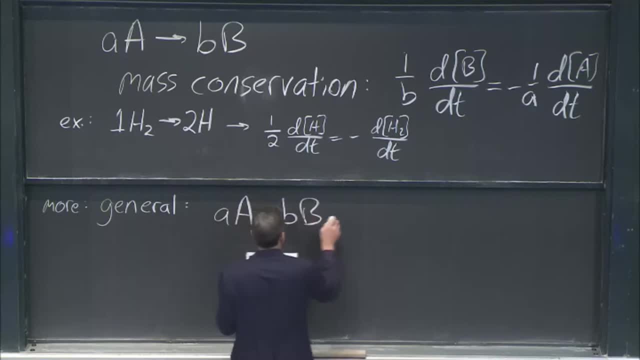 Let's have A, A plus B, B goes to C, C plus D, D. So now I've got four things, two products, two reactants. All right, OK, A and B are the reactants, C and D are the products. 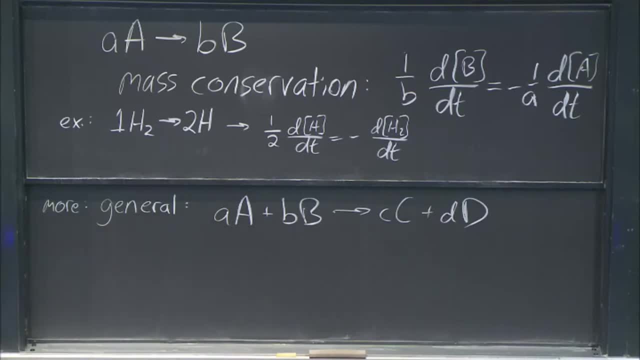 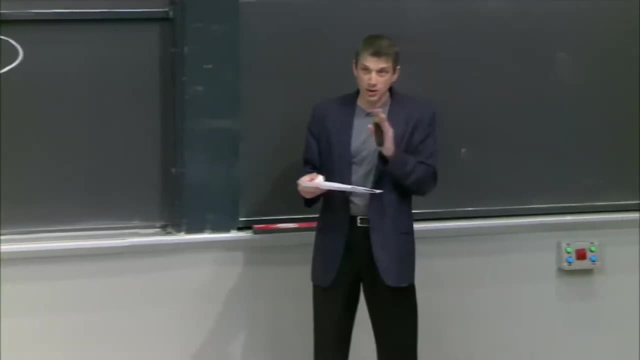 And they've all got their coefficients, And so you could look at the change in any one of these and know the rate. You could look at the change in any one of these and know the rate. So if I look at this, then the rate 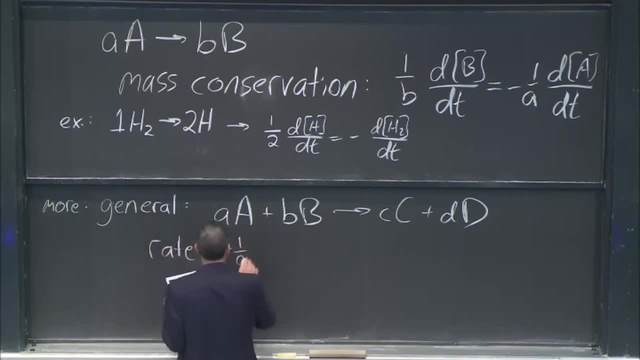 would be equal to minus 1 over A right convention. OK, it's a positive value. That's got to be equal to minus 1 over B times the change in B With time, and it must be equal to plus 1 over C times. 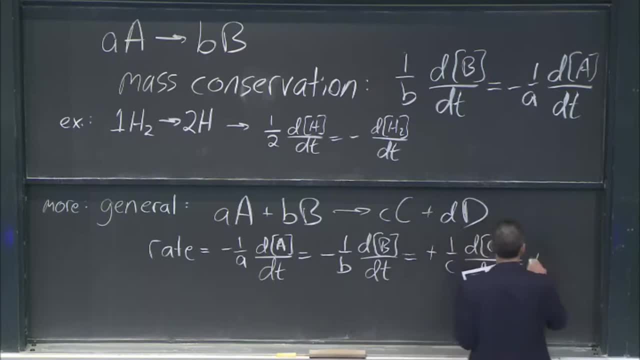 the change in C with time, And that also must be equal to plus 1 over D. right times the change in the concentration at D change DT Right. So I can look at the way any one of these things is disappearing or forming. 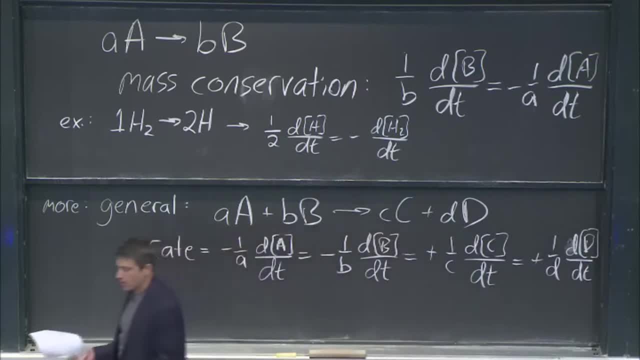 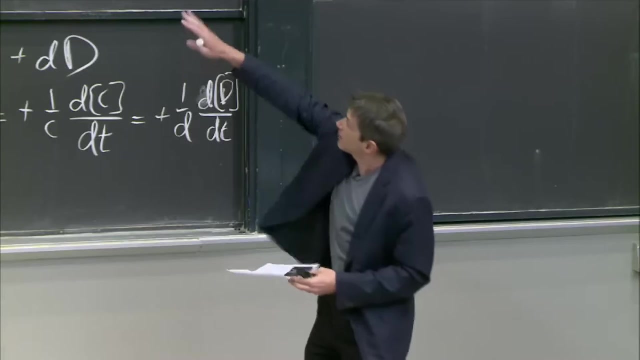 And because those stoichiometric coefficients are there, I know, I know what the rate of that reaction is. Again, this is basically a statement of mass conservation, But there's more, Because this is just a definition of rate: Rate is changing concentration. 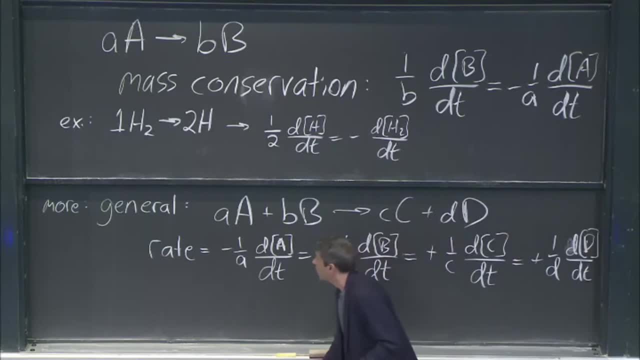 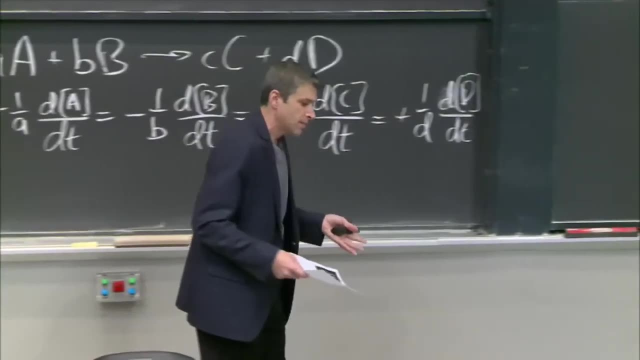 And it's always positive Done. But I want a law. I want to know, not just OK, yeah, I see how you change with time, so that's a rate- But I want to know a law that if I gave you, 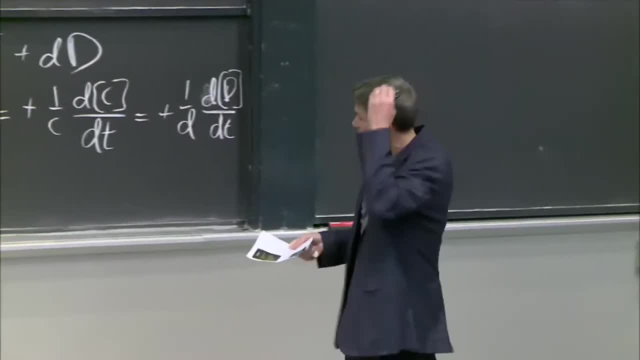 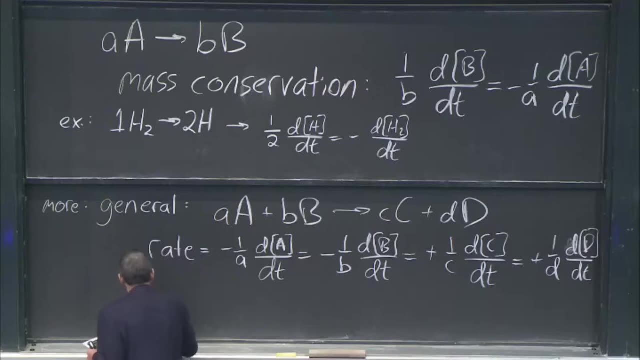 any concentration. if I gave you any set of concentrations, what would the rate be? What would the rate be? Could I come up with a function? And so we write down the rate as depending on the concentrations. Now you can do this with the products or reactions. 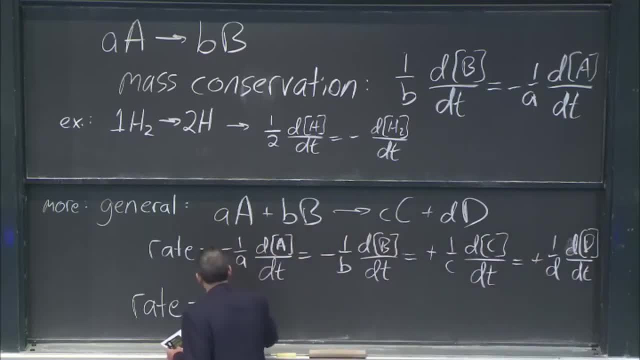 We're going to do this with the reactants, And so you would have that. it depends on the concentrations of A and B raised to some power With some coefficients. So k times the concentration of A to the m, times the concentration of B to the n. 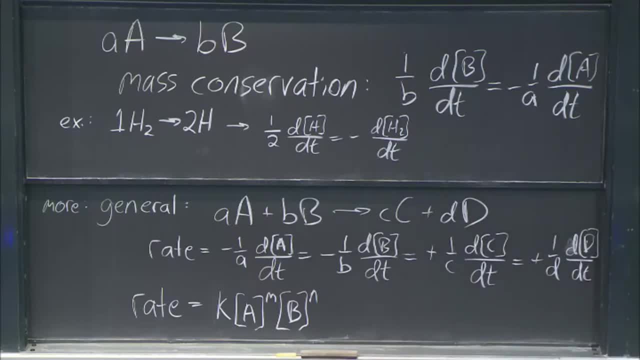 So we're raising these Now we don't know what these are, But what we're saying is that there's got to be a way. if I just know, maybe, if I do some experiments or something, maybe I could come up with a general function that 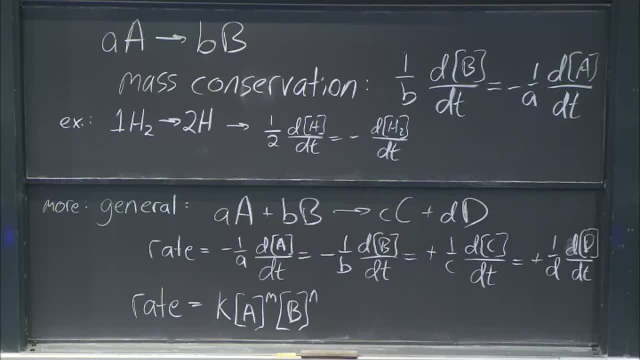 depends on just the concentrations, wherever they are, of A and B, And they're going to be raised to some power And some exponent that I don't know yet And they're going to have some constant. That's a rate law. 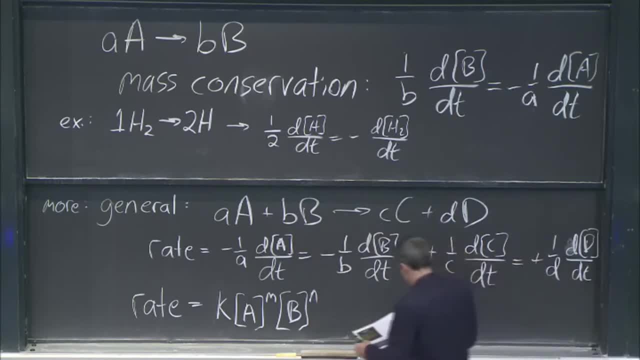 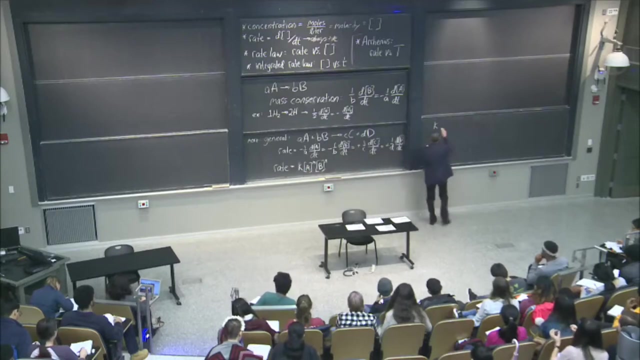 That's a rate law, And so now, OK, now the thing is that the rate law let's go over to here. So the k is, as you can imagine, going to be very important here. That's called a rate constant. 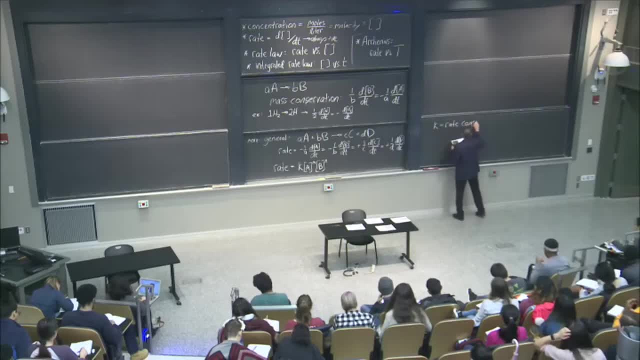 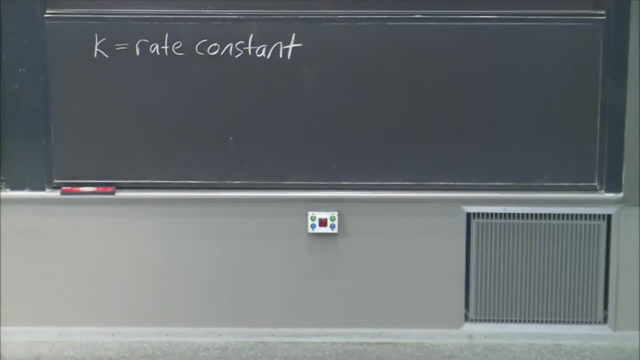 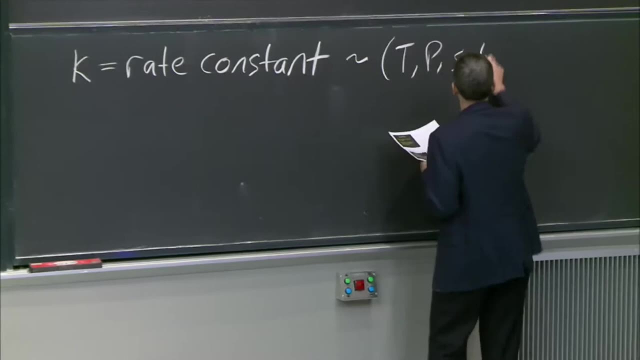 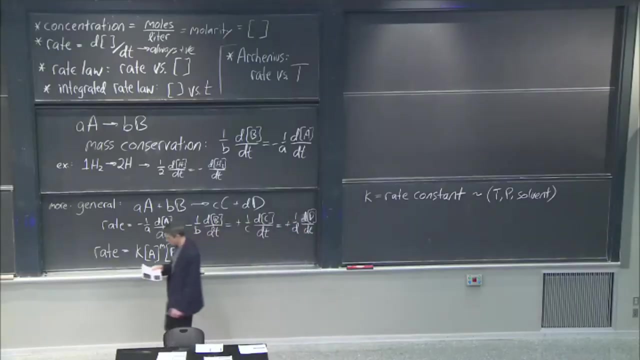 k is equal to a rate constant, OK, And this is going to depend on conditions like temperature pressure solvent. So it's going to depend on things like temperature pressure solvent et cetera, And we'll see how you get k. 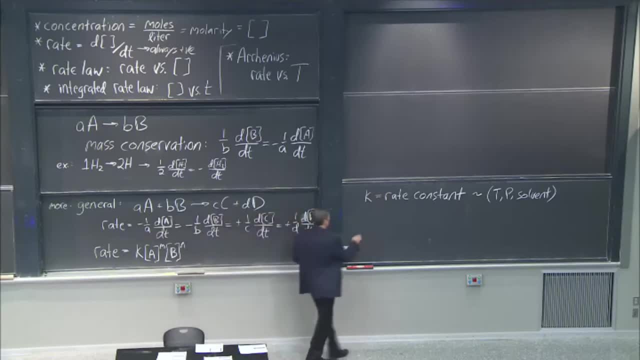 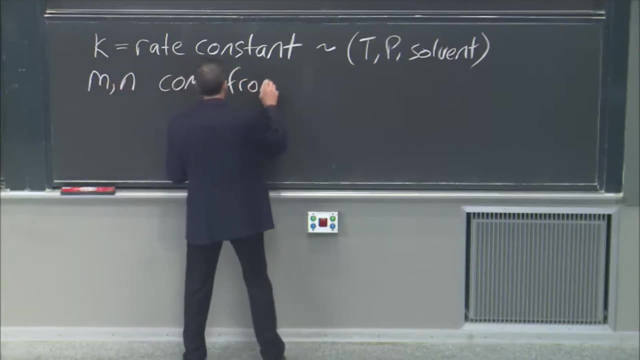 But m and n cannot come, And this is very important. m and n, and k for that matter, must come gazuntite from experiments. They're determined experimentally, Determined experiment experiments. OK, So you can't. this is a mistake that is often made. 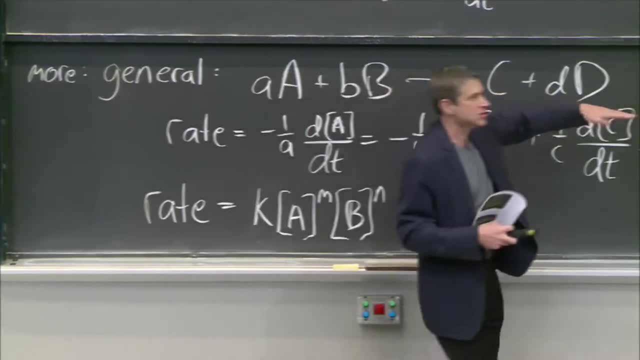 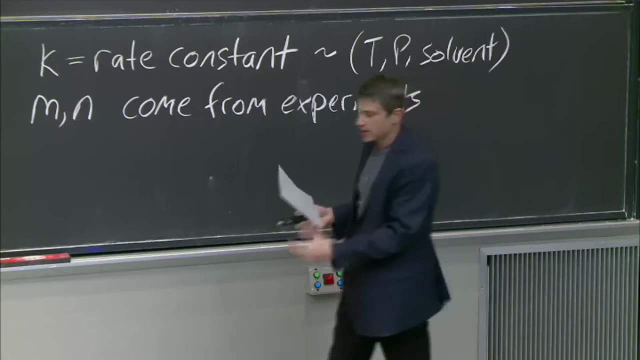 m and n must somehow be related to these coefficients. No, m and n is something else. I've created a function that the rate depends on, the rate of this reaction depends on. I've put these out there. I've put exponents in there. 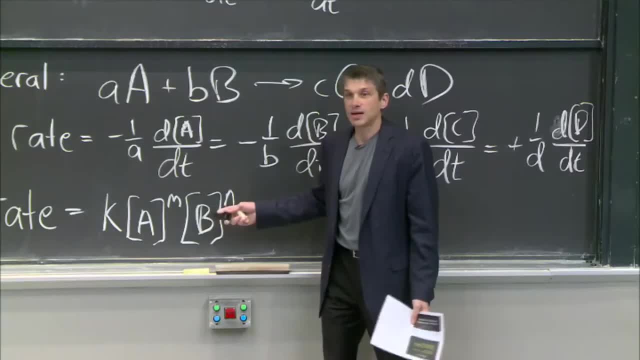 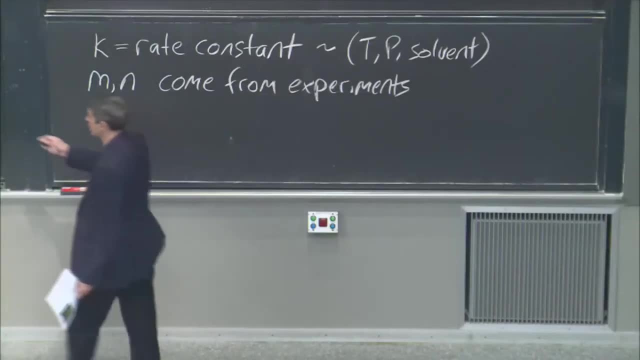 And I'm looking for the dependence on m and n. And the only way to do that, to know that, is to do experiments. You can't just get that from the way the reaction is written. You can get mass conservation and the relationship. 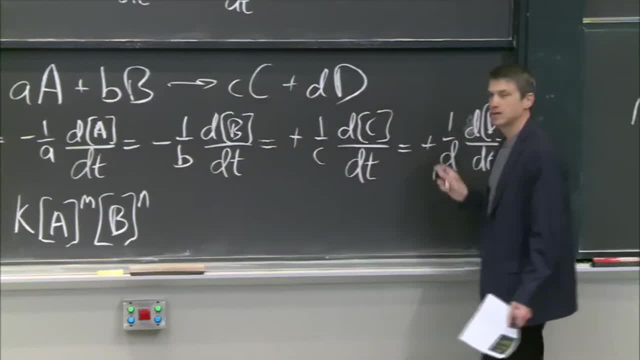 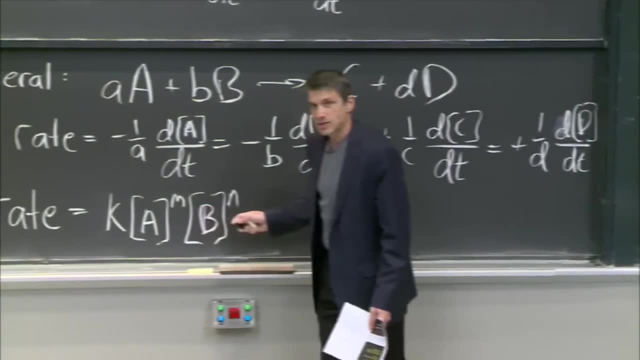 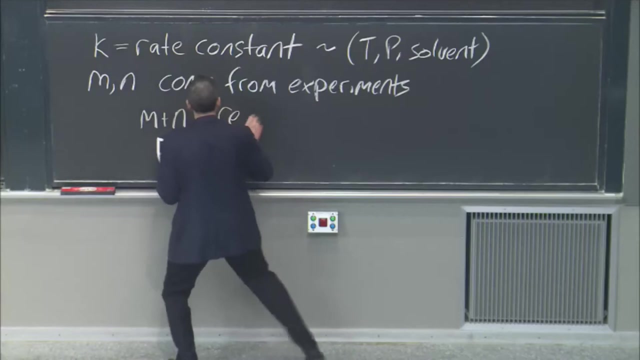 between rate rate, rate rate, Those are all the same. But you can't get the rate law unless you do some measurements Now. then when you do, then you're going to get the order of the reaction. So this is the reaction order. 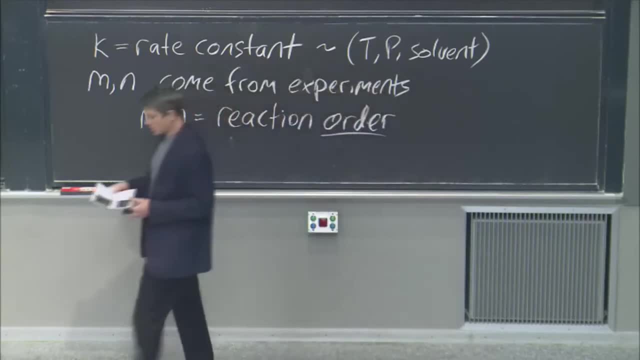 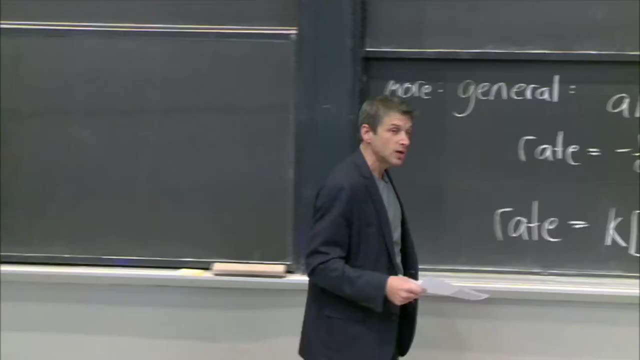 And that's an important, that's an important property. And there's one more thing I'll say, And then what we're going to do, I'm setting the stage here And then we're going to do examples. OK, so don't worry. 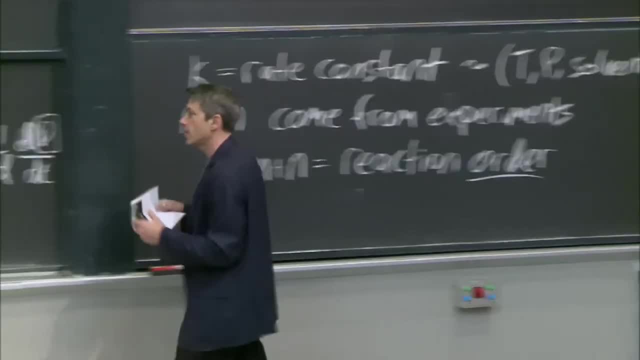 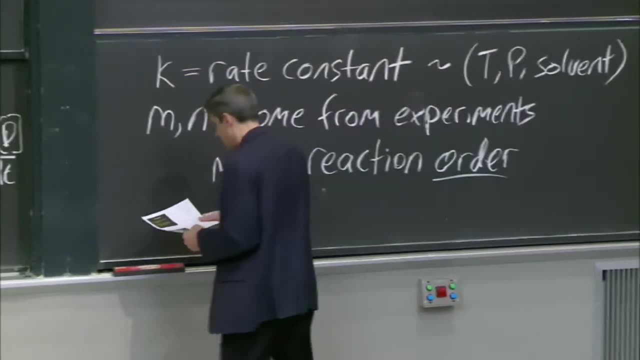 We're going to go through different examples. that I think will help kind of crystallize these concepts. But the last thing I want to say in terms of setting the stage is that the rate, the units of rate, if you look at how I've defined the units of rate, 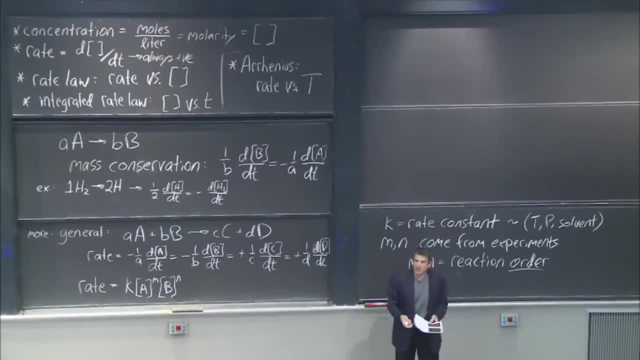 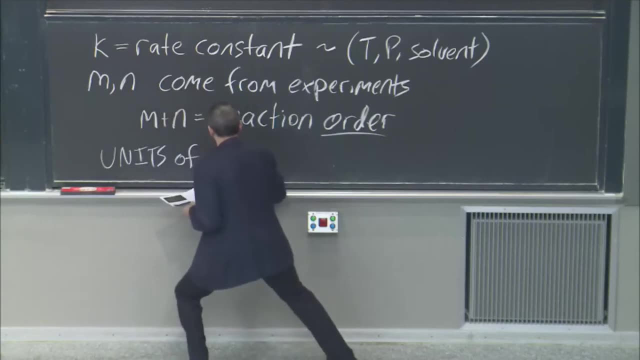 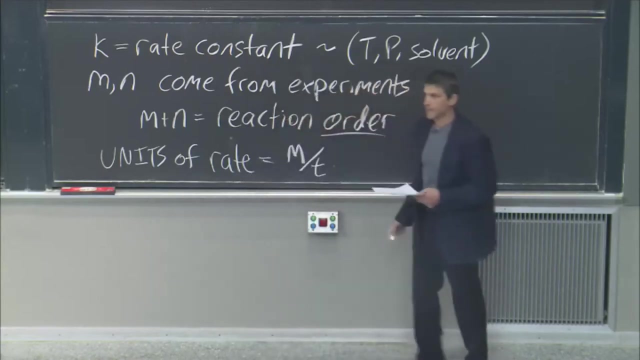 it's a change in concentration with time. So the units of rate, the units of rate are going to be molarity over time. That doesn't change Right, That doesn't change. Those are the units of rate. That's the definition of the rate. 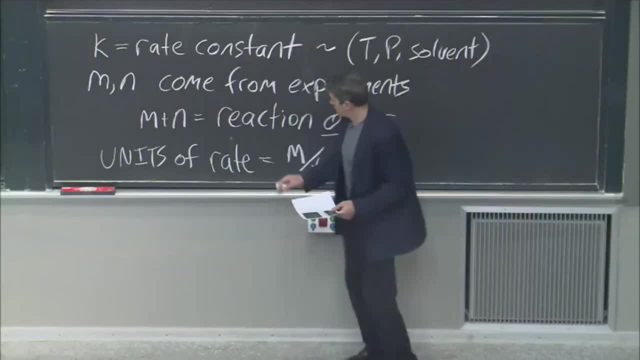 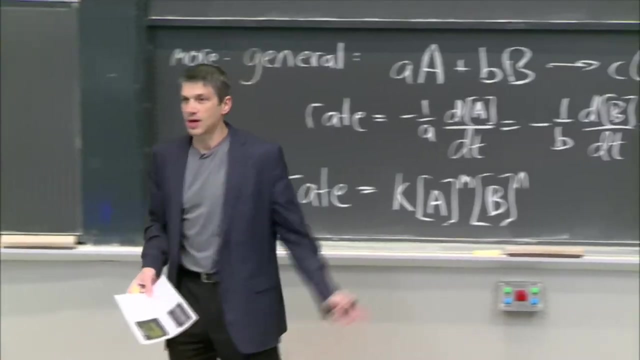 But you can see, and we will see, that if that has to always be true, then the units of k may vary, And we're going to see that as we go through examples. So the units of k could be different and will be depending on the reaction order which. 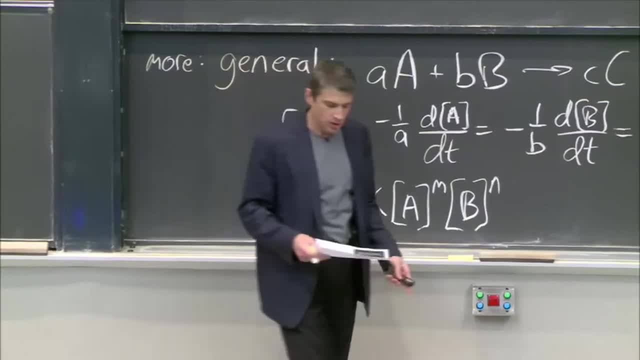 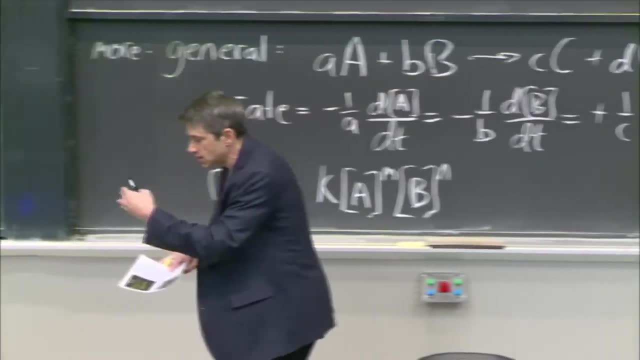 is basically saying it depends on the rate law. OK, Setting the stage. Now let's look at some examples, And we're going to go through this sequential. We're going to do a zeroth order reaction, then a first order reaction and then a second order reaction. 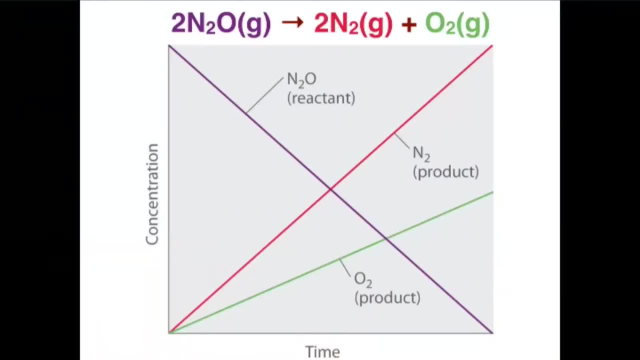 OK, So zeroth order. Well, zeroth order: reaction right in a zeroth. So this is nitrous oxide. So this is a reaction of nitrous oxide turning into N2 and O2.. Nitrous oxide is used in many, many applications. 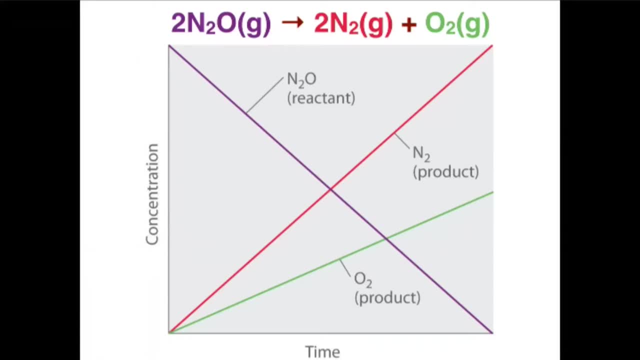 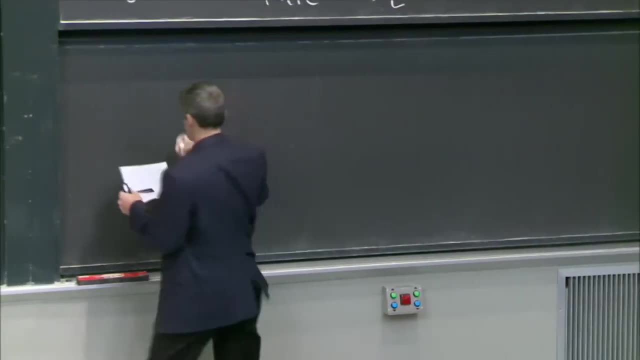 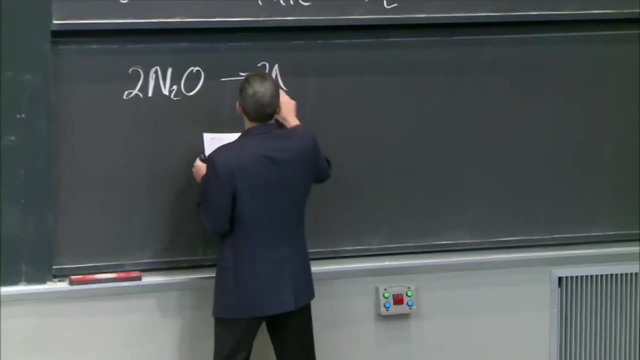 So it's not just laughing gas, And so if we sort of go with what we just wrote down, OK. so let's take this example. I'm going to write it down here: 2N2O goes to 2N2 plus O2.. 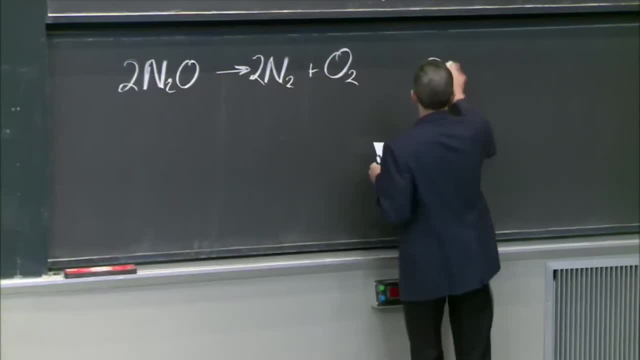 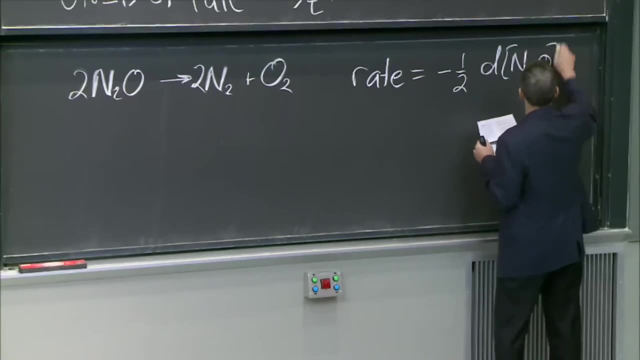 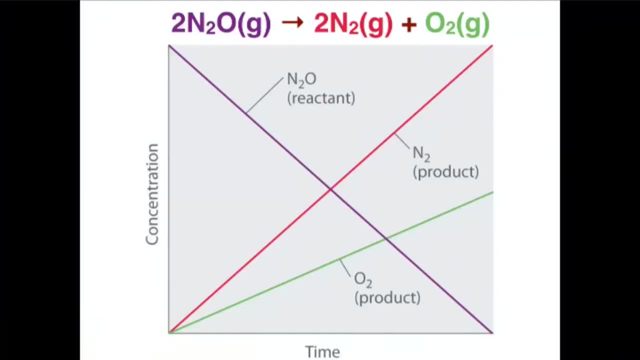 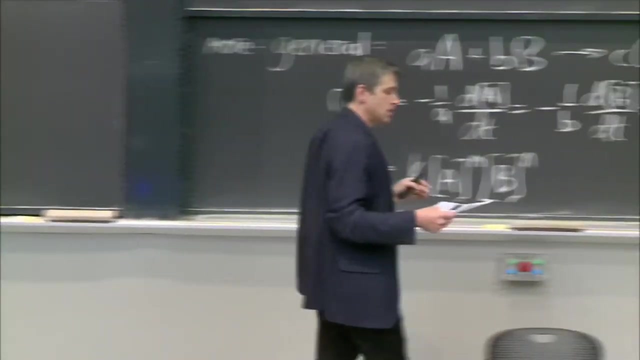 So, but see now, OK, so now I'm doing some measurements And I'm plotting some data here. So I'm plotting here the concentration of all three of these- the reactant and the two products- with time. And what you notice is, if I plot the concentration with time, 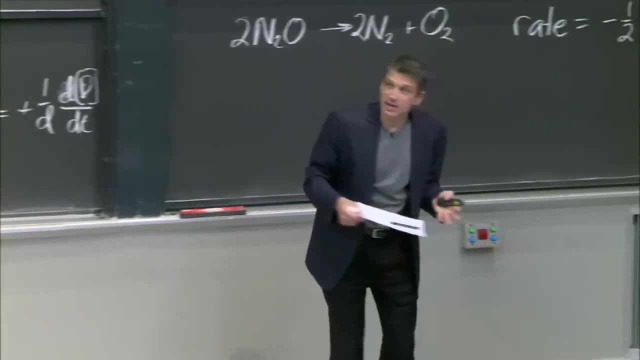 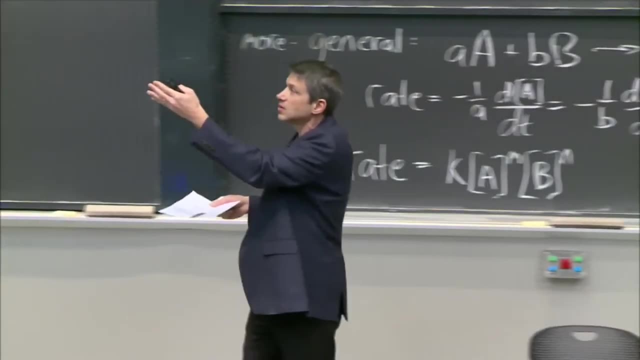 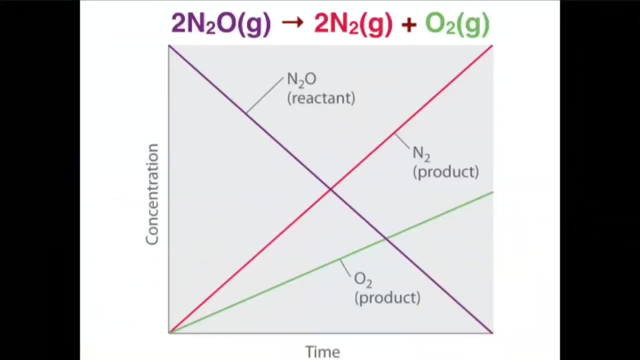 what does that mean? That means that they don't depend on concentration, Because the rate is the change, All right. the rate is the change in those with time, right, the change in the concentration of time. It's always the same because it's a straight line. 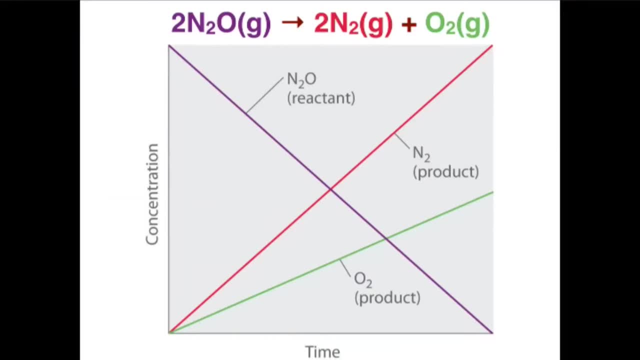 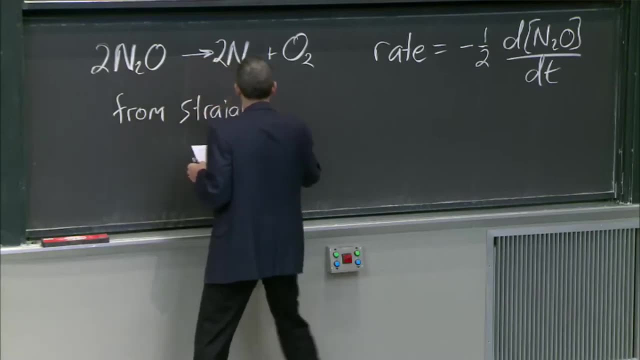 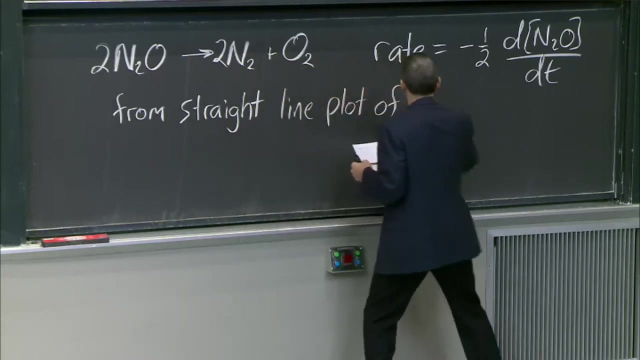 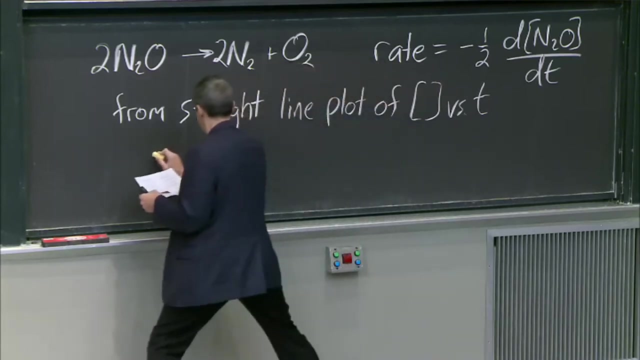 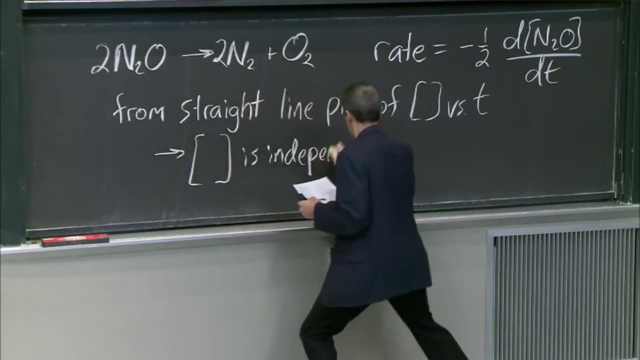 So if that's true, then the rate from, let's say, straight line, straight line. OK, we'll talk about plots as we go. straight line plot of concentration versus time, straight line plot, then we know that concentration is independent of time. 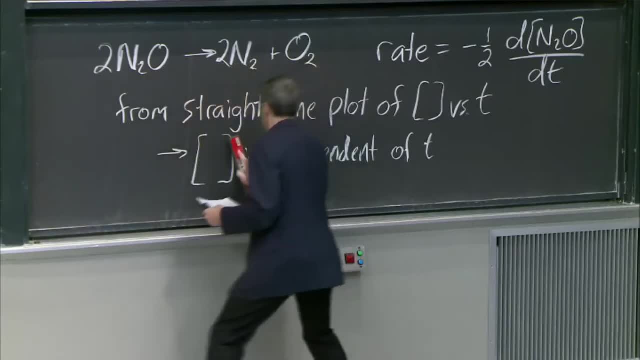 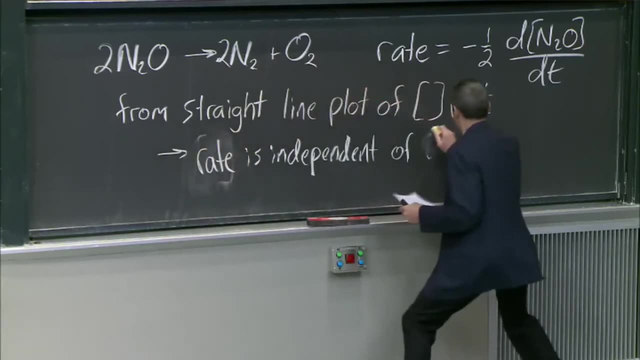 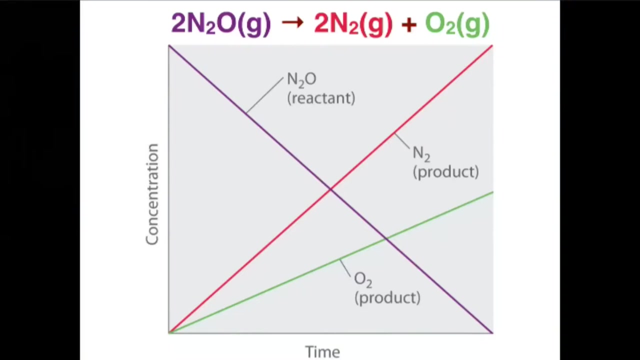 I'm sorry. rate is independent. Hold on. Rate is independent of concentration. The rate in the beginning is the change in concentration, The rate in the middle is the change in concentration with time, And it's a straight line, so it's always the same. 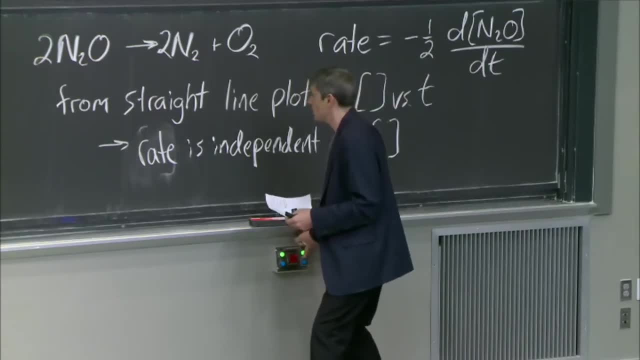 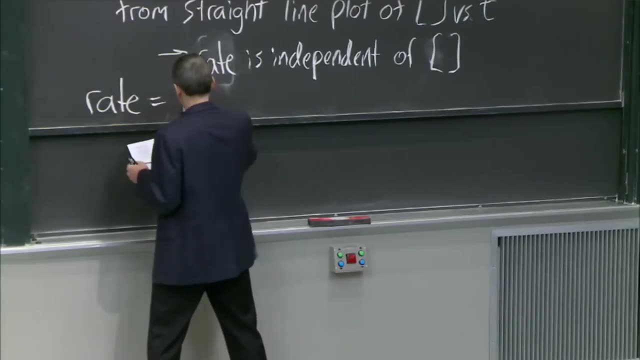 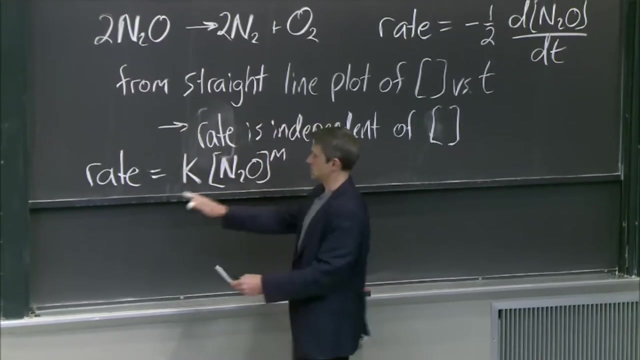 Well, that means something. It means something in terms of our rate law, Because now I know from my rate law that the rate is equal to k, the rate constant times n2o to the m. That's from here You take all the reactants and you put them down. 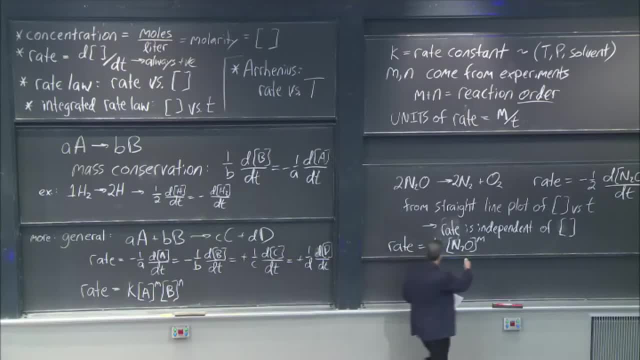 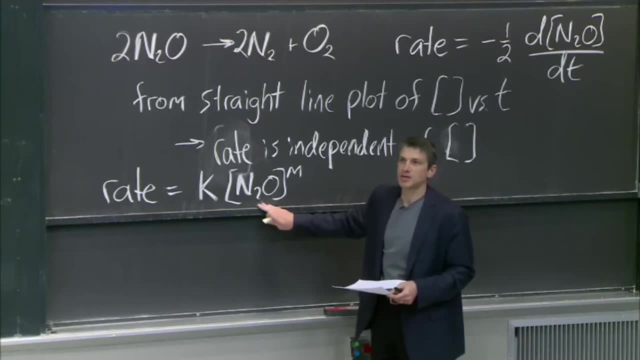 and you put exponents on them, And so I've just got 1, n2o and it's raised to the m. But I know there's no concentration dependence of this rate, So I know that m equals 0, and it's a 0th. 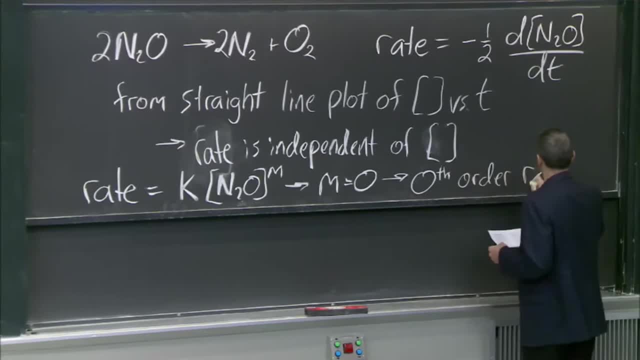 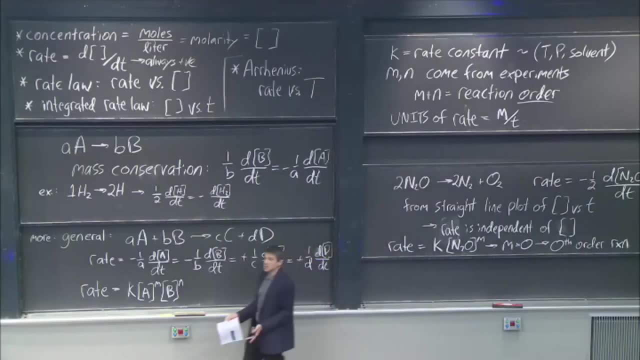 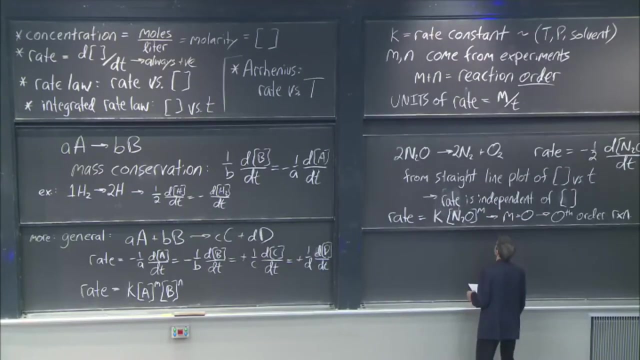 or a 1th. It's the order reaction: Rxn- ah, saves so much time. Rxn reaction, which means that the rate is simply equal to k. The rate must equal k, OK, So in this case, the rate, right. 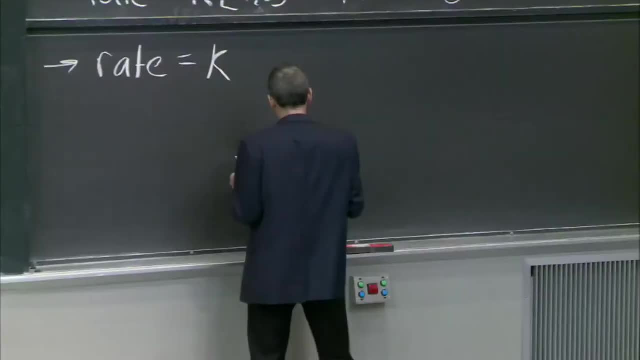 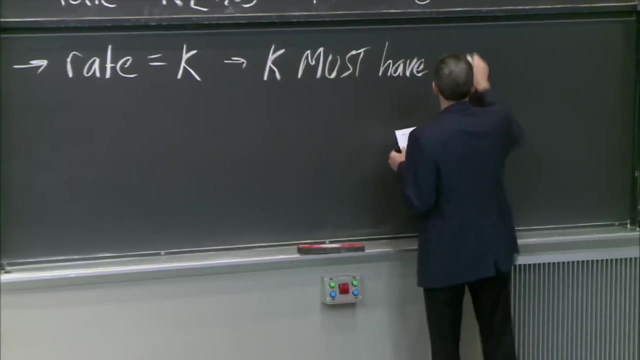 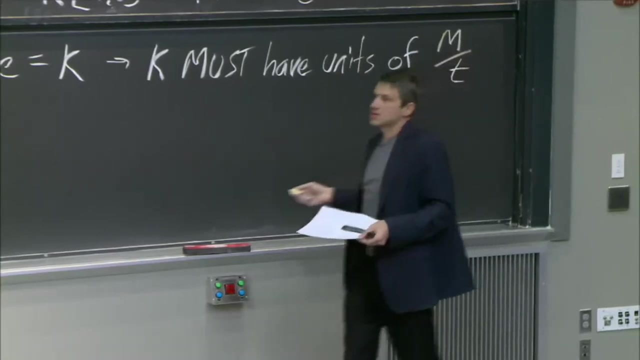 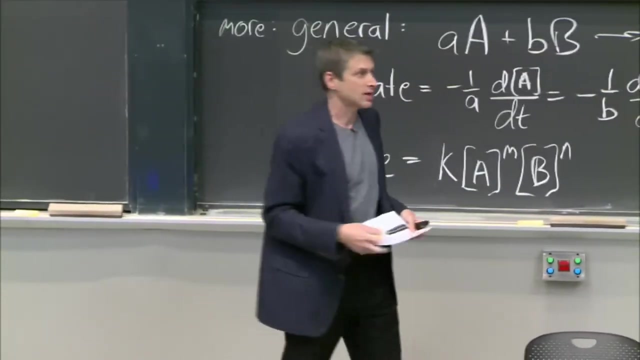 So we're continuing here. equals k, And that means that k must have units of molarity over time. Why? Because that's the units of rate. The units of rate don't change, The units of k will, But in a 0th order reaction, the units of k. 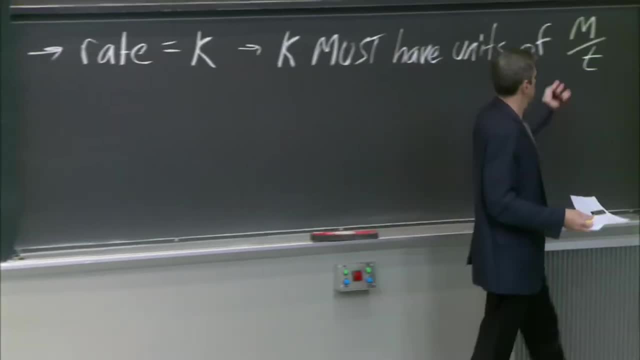 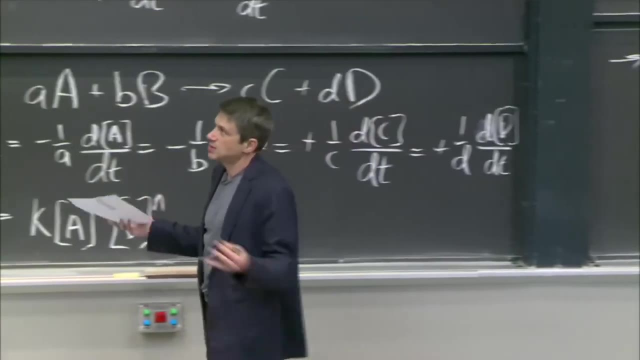 have to be equal to the units of rate. There's nothing else in there, OK. Again, I want to emphasize: there is no simple correlation between the stoichiometry- you know the coefficients of these things- and the rate law. 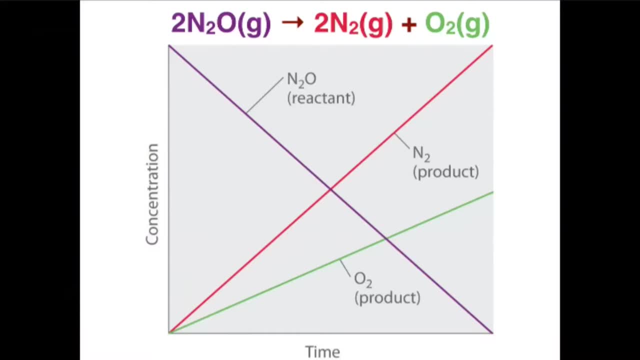 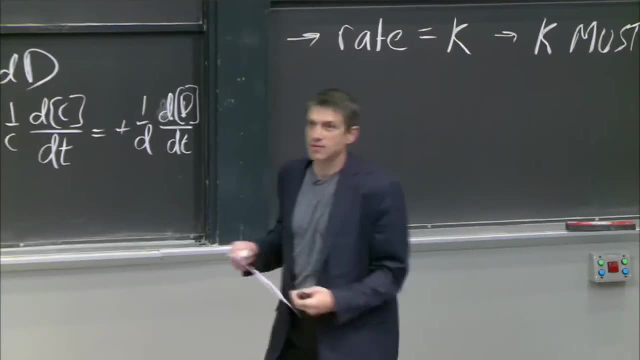 You've got to do experiments. This data comes from. oh, look at it, There is the mass conservation in action: O2, N2, right, You can see it, You can feel it. Slopes are different. They must be. 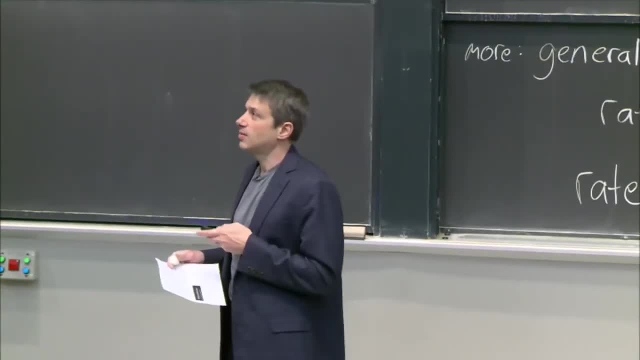 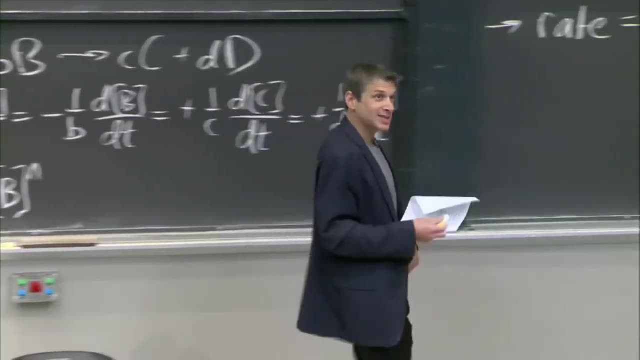 Now let's take a look. Now here's a reaction some of you may care about. So why does the 0th order reaction matter? Why does it matter? Because that's the reaction of beer. Maybe you do it. so ethanol- OK. 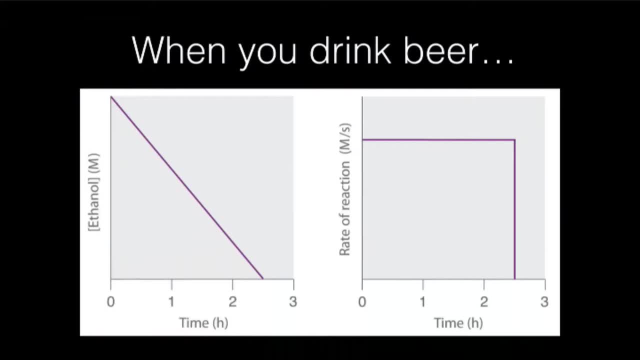 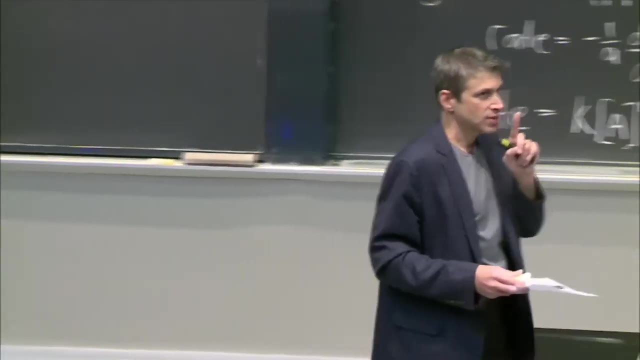 But we'll call it beer. So what does this mean If I consume beer? if I did, then the concentration of ethanol in it- there it is plotted versus time- is linear. That means- this is very important- it's a 0th order reaction. 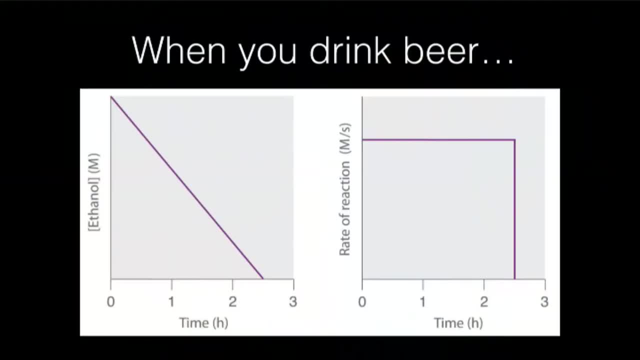 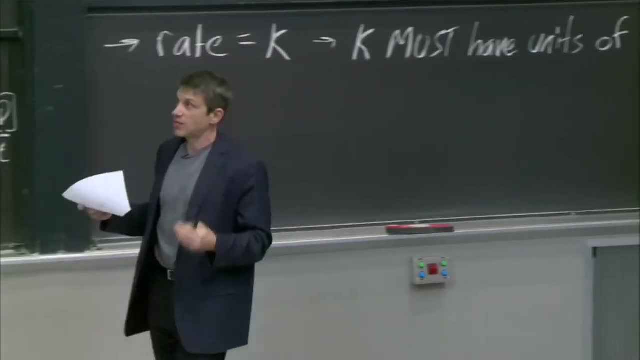 It means if I plot the rate of the reaction, you see it. There it is. It's a constant. It doesn't depend on the concentration. That really has a lot of ramifications, because if I drink a lot of beer, the average 70 kilogram person it. 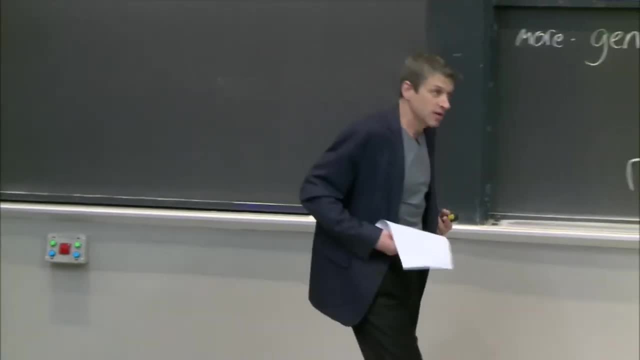 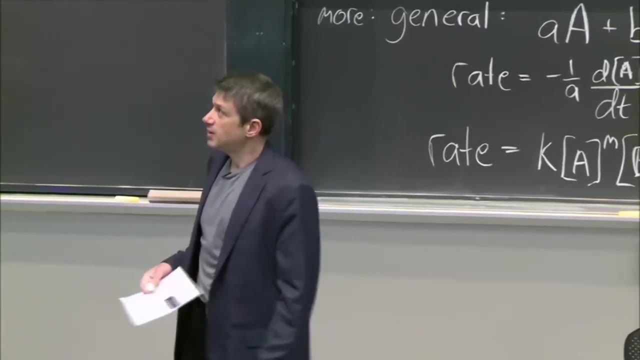 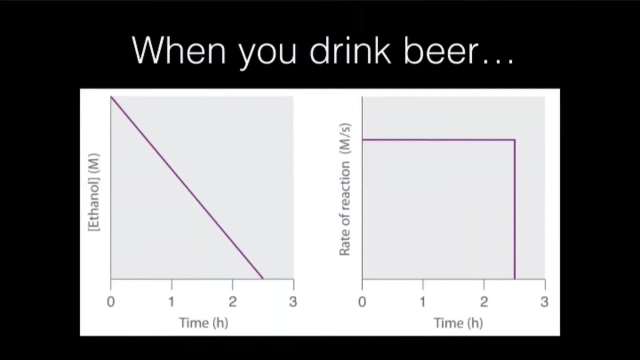 takes 2 and 1 half hours for the enzymes in their liver to decompose 50 milliliters of ethanol- one beer, But look at that. So that means that if I had more than that, you got to wait. The body can't. 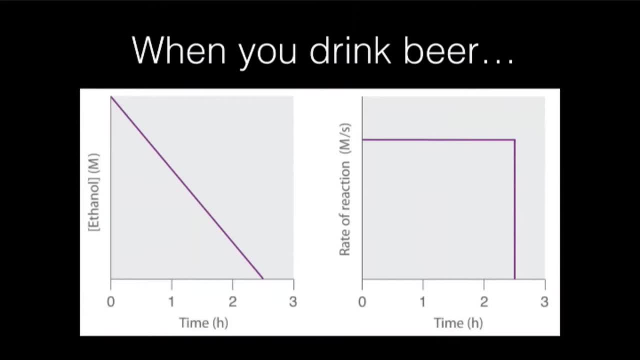 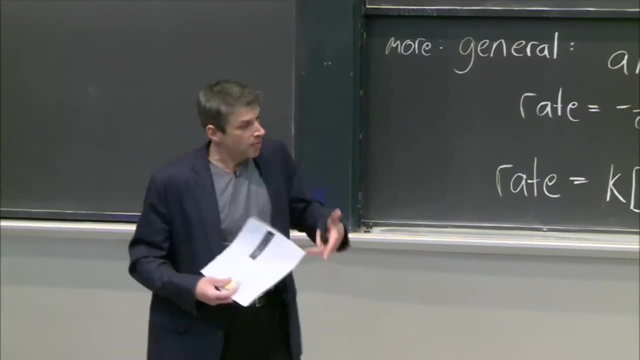 It's not dependent on how much I have. The reaction of the liver, the enzymes that are breaking this down, is not dependent on the concentration. So if I load up a lot more in there, it doesn't matter. There is a pipeline and there is a rate. 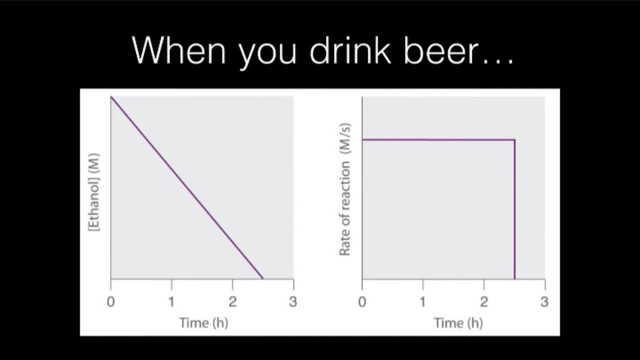 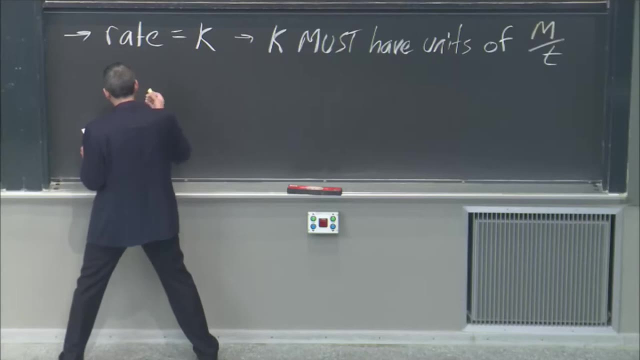 and it's not changing. Well, that leads to consequences to be thought about when you drink beer. But there's another thing we can do with beer, which is we can integrate it. Right, Yeah, Yeah, If we know that it, you know well, if we know that beer. 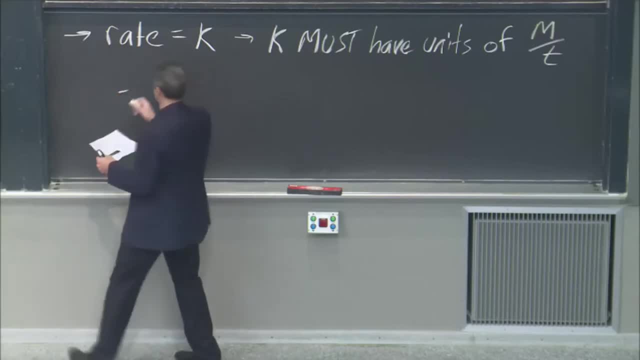 if we know that minus, I'm going to say there's some reaction that beer goes to something. So minus d beer, right, dt OK. well, assuming it has a coefficient of 1, is going to equal. that's the well, that's going to equal k. 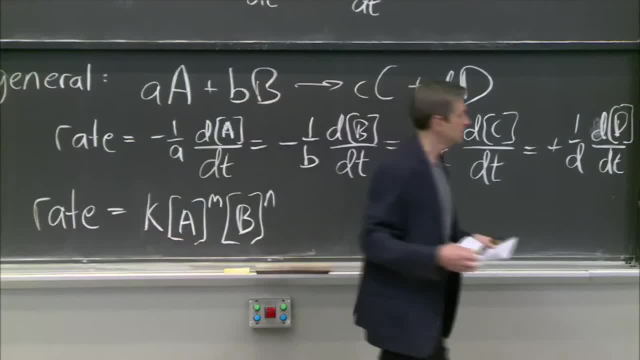 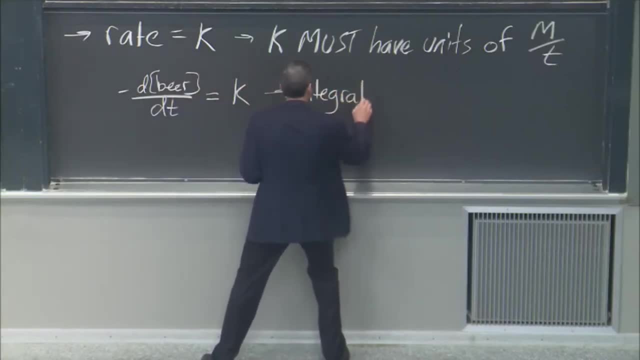 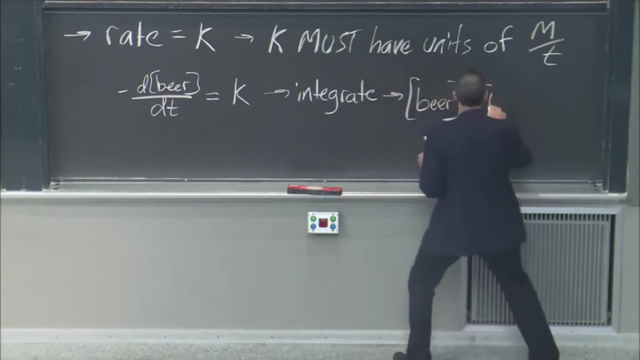 because it's a zeroth order reaction. right, It's a constant, And so OK, now I integrate both sides. If I integrate, then I've got the integrated rate law for beer, which is that the concentration of beer is equal to some initial concentration of beer, right? 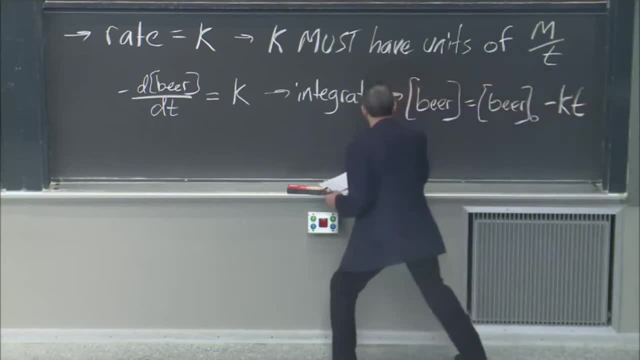 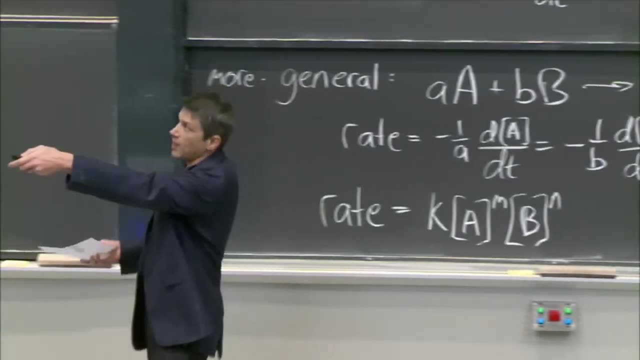 minus kt. This is the integrated rate law. That's the integrated rate law. Notice what I've done. I've gone from talking about the rate of the beer being, you know, the rate there, which is a constant, to a dependence. 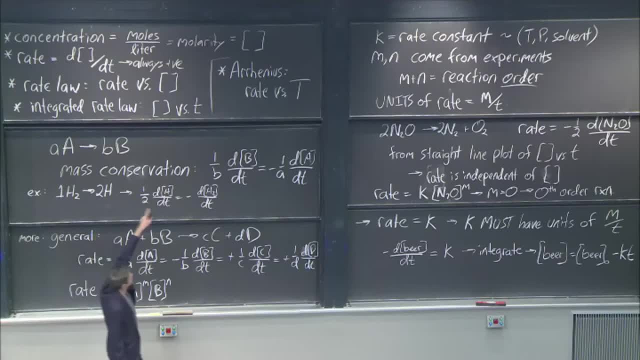 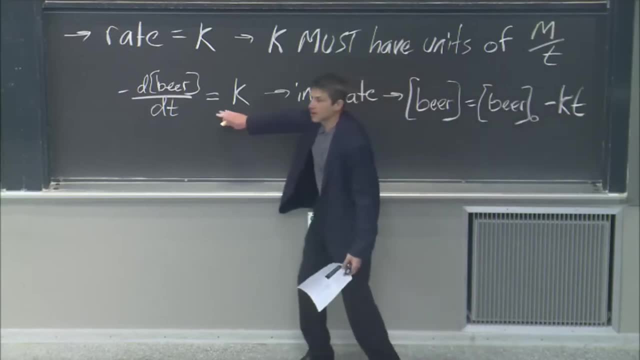 There it is: integrated rate law. The promise was that would get me a concentration versus time, and that's what it did: Concentration versus time. How did I get it? Well, I had a rate law and I integrated it. 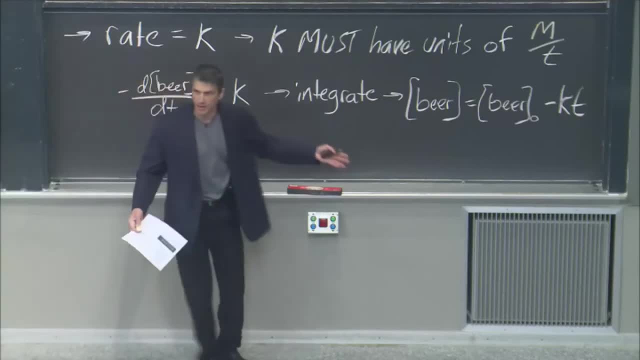 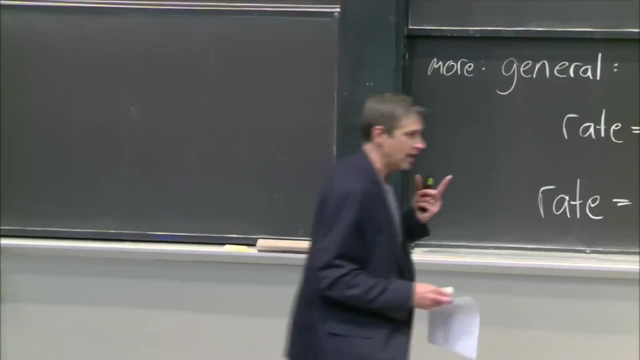 And I'm not going through the math, but you know, you put the dt over here and you integrate, OK. OK, so that's an integrated rate law. Well, let's go to the next order. If I had first order- and I looked at the data for that- 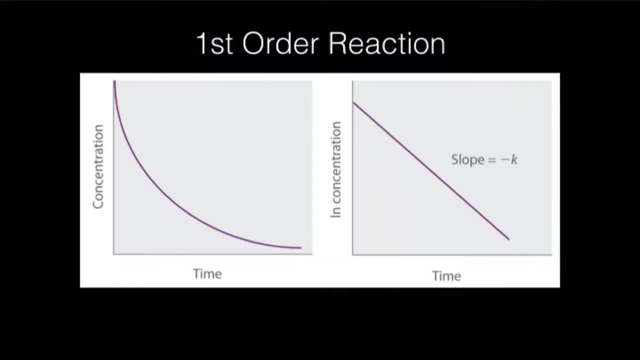 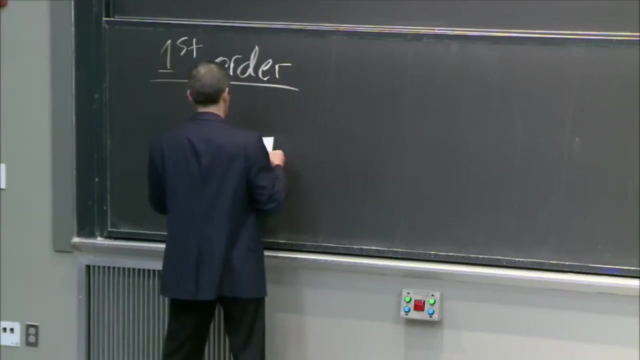 then you would see, if I plot the concentration versus time, it would not be a straight line. Why? Well, because for a first order reaction. so now we're in first order, right Then. so what that means is that the exponent here is a 1.. 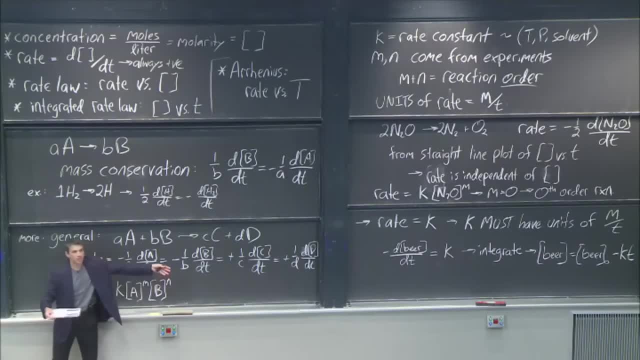 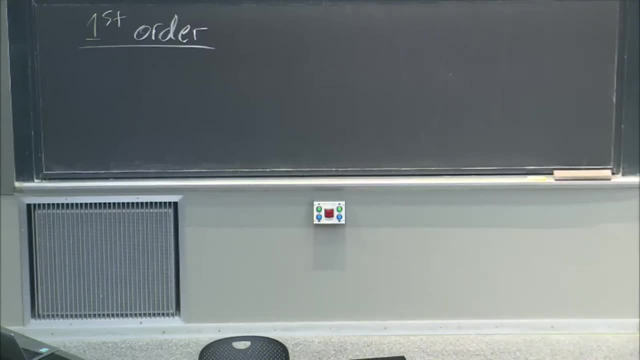 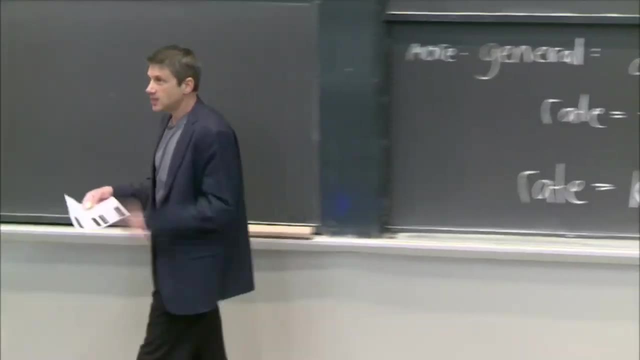 Or if I have two reactants, the addition of them is its first order total. Or it might be dependent on two reactants and its first order in each of them, but then second order overall because they're multiplied. But let's stay with the simpler case of just one reactant A. 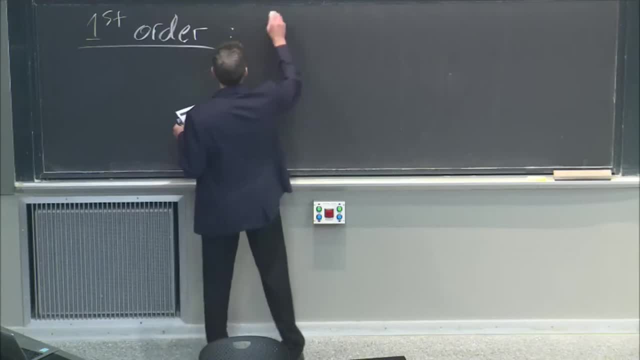 OK, so if it's one reactant and let's suppose A goes to some product, I'm not even going to write it out. You know that the rate is equal to minus the change in the concentration of A with time, right? 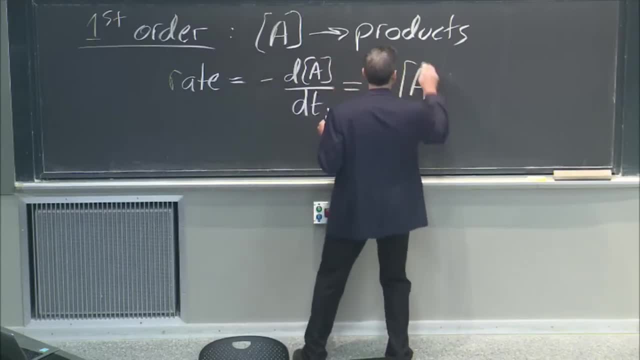 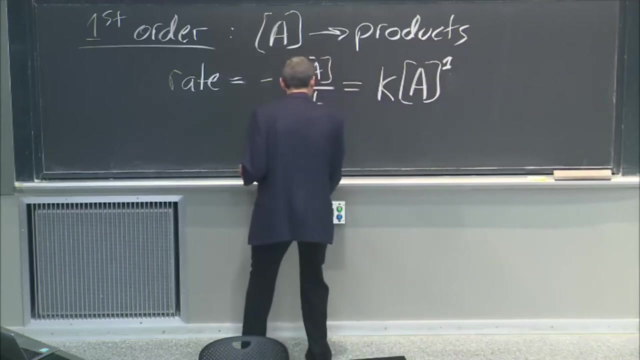 And that, because it's first order, it depends on the concentration raised to the first power. That's what we said. first order meant right? I'm telling you, this is first order now, OK, Well, you can see that if it's first order, 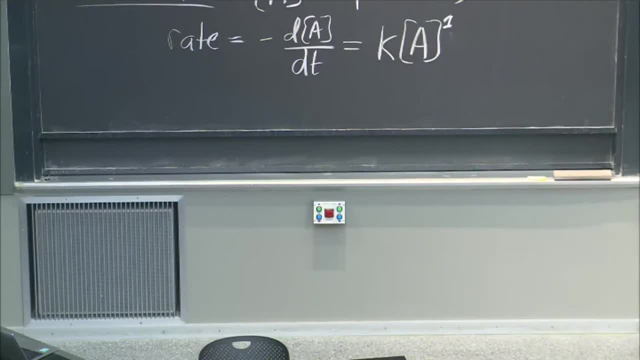 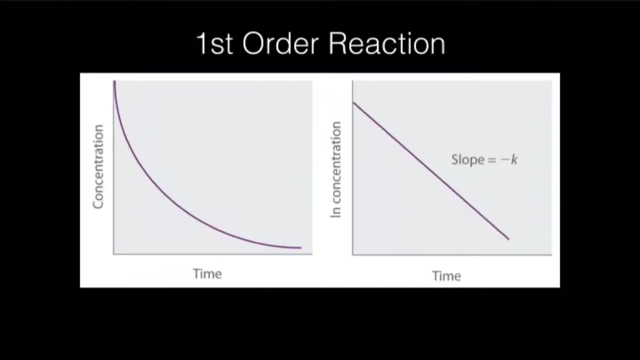 it depends on the concentration, And so that means that you know, you can see from that and you can see from the plot. If A, if the concentration of A, doubles, the rate doubles, The rate doubles. Why can't our livers do that? 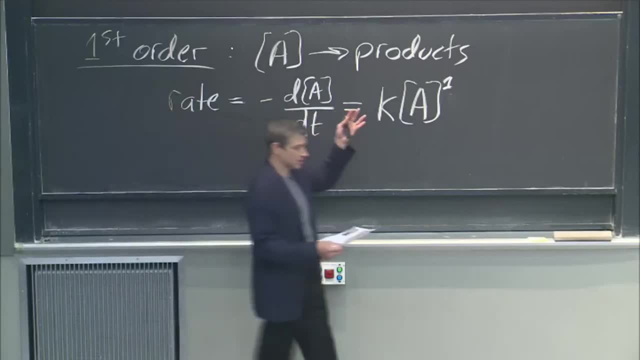 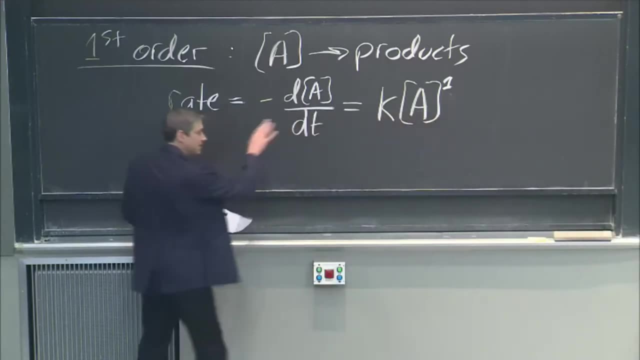 No, they're zeroth order, But there are lots of reactions that are first order, And so now, OK, here's the thing right Now, if this is, but the rate still has to have units of molarity change with time, right. 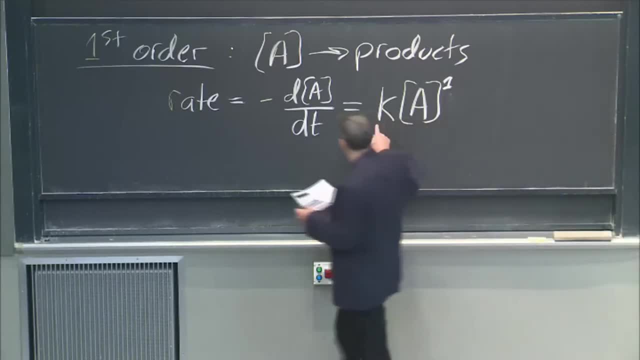 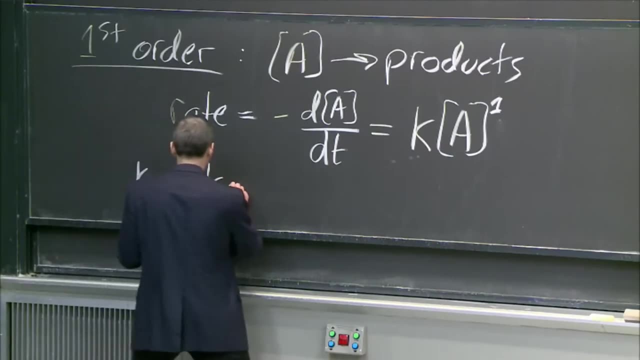 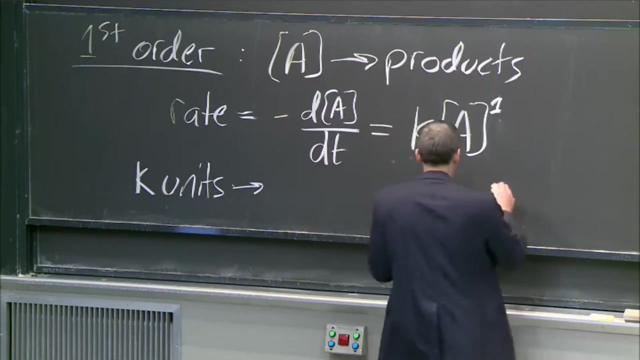 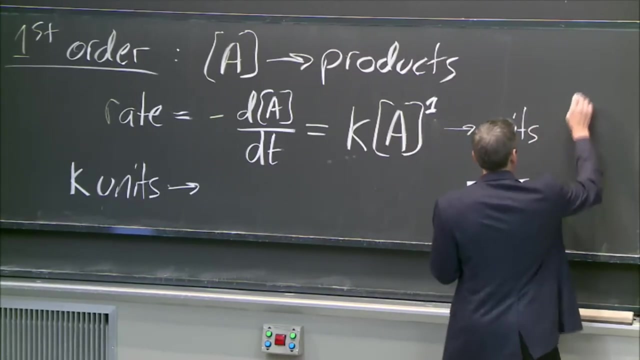 Molarity over time, And it can't have that unless k's units are. k units, in this case, are going to be. So let's see. Let me write down: OK, Rate has units. The overall units are molarity over time. 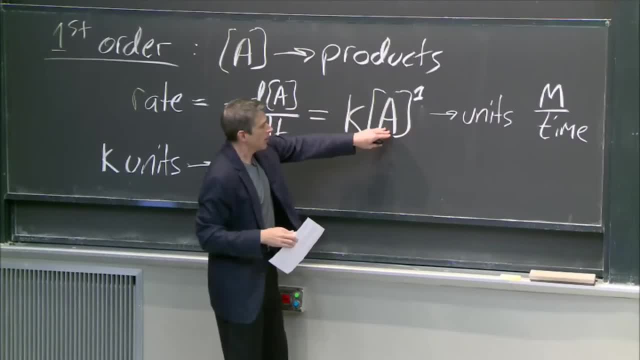 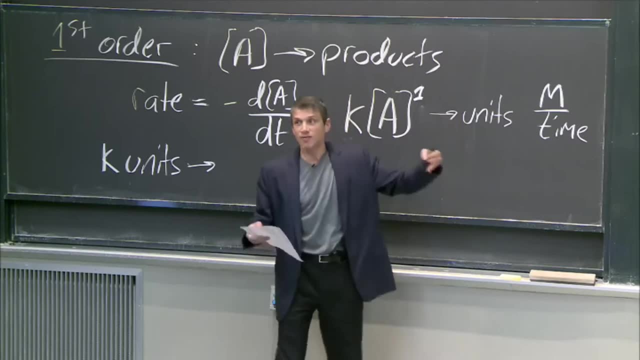 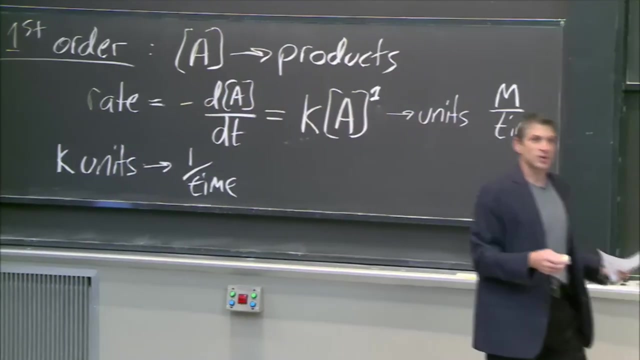 So now I've got k times molarity. That has to have units of molarity over time, all right, And so k must have units of 1 over time- 1 over time. But that tells us what to plot. It helps tell us things about like what: 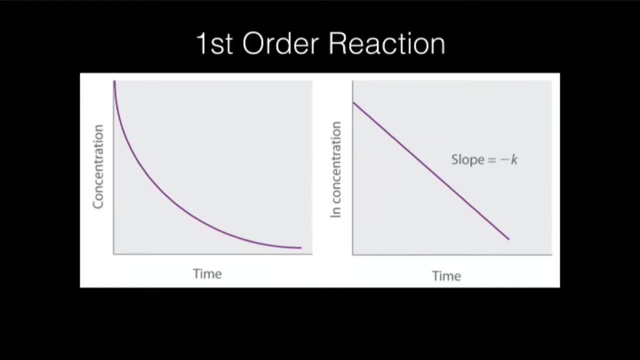 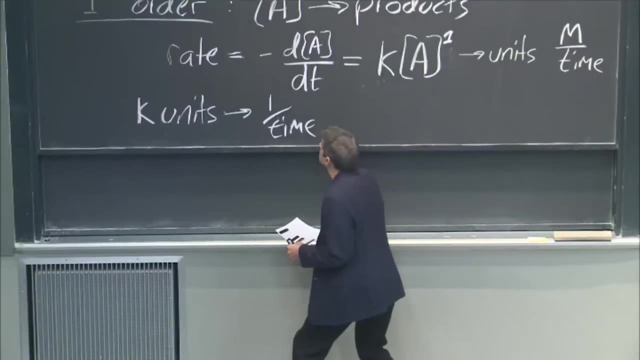 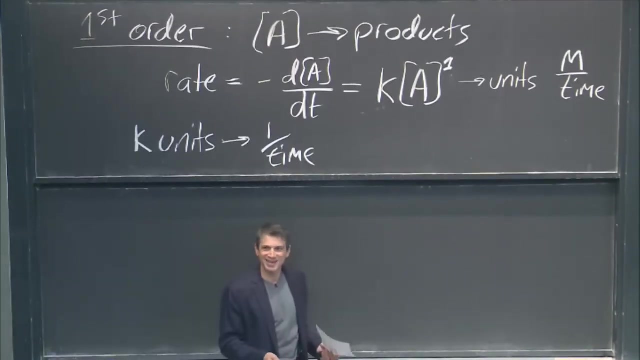 But the plots always come better when we integrate. If we think about the integrated rate law, then it leads to linearity, Which is something we always want in plots. Linear lines, Straight line, Linear lines- Really, I just said that. 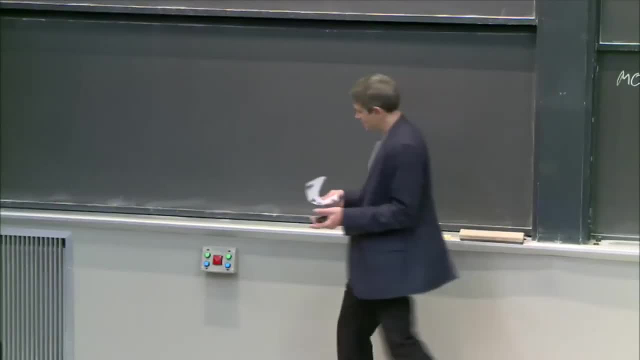 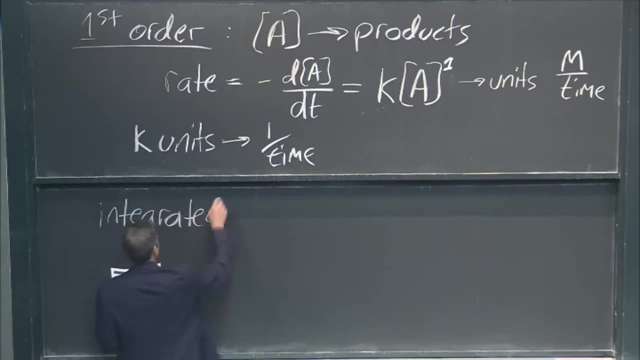 I did just say that I'm OK with it, Because it's true, But let's integrate this Integrated rate law. So now there's my rate law. Now I'm going to take the dt over and the concentration over And I'm going to integrate. 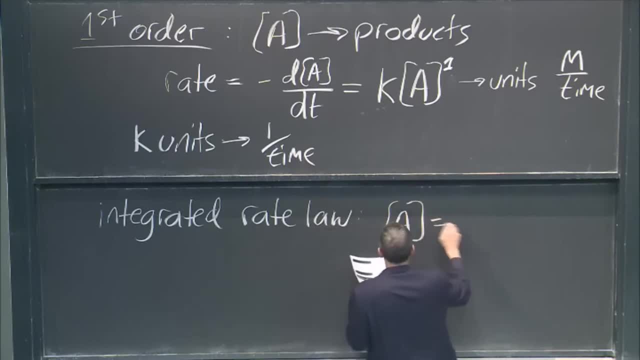 And I get this: A equals Some initial concentration times e to the minus kt. Notice the units right: 1 over time. That's good. Or, if you want, you could say that that's a log. a equals log a0 minus kt. 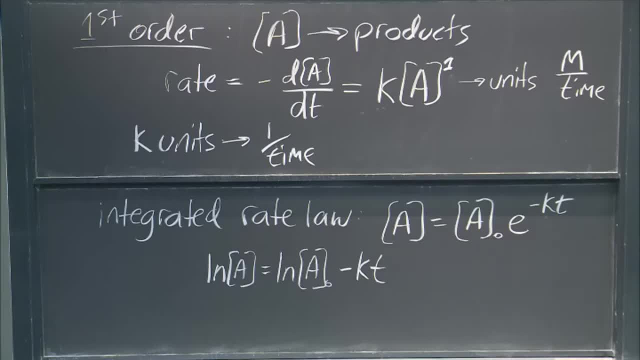 And this right now. this gave it to me, Because now you know that if you plot log versus time, if I have a plot of log versus time, if I have a plot of log versus time, then it's linear And we like linear. 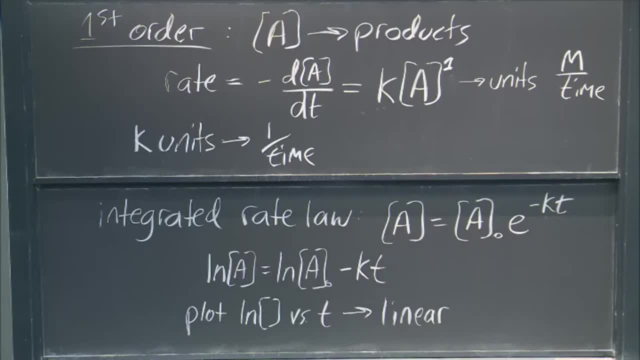 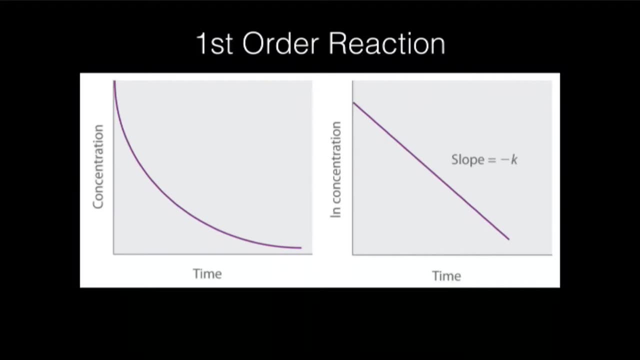 And that's what's plotted on the right. So that's a plot of log versus time, And so you can kind of go backwards and forth. It's like if I had a linear plot with concentration versus time. you know, it's zeroth order. 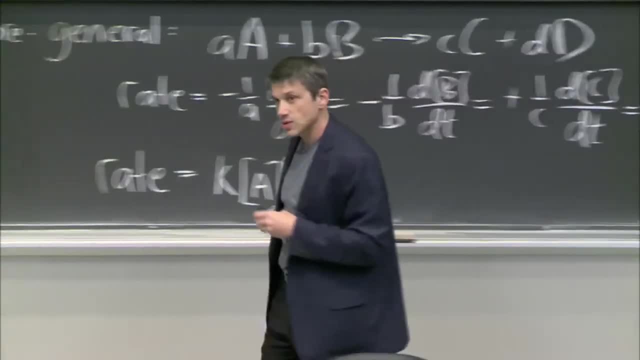 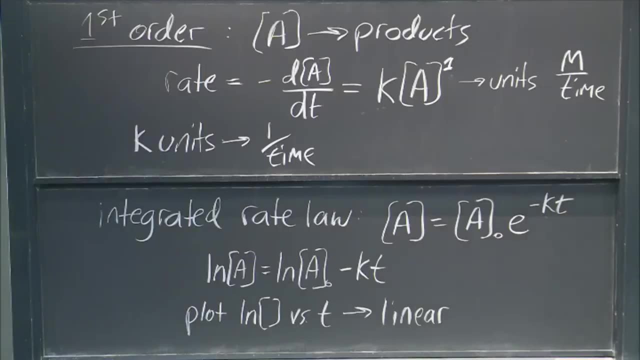 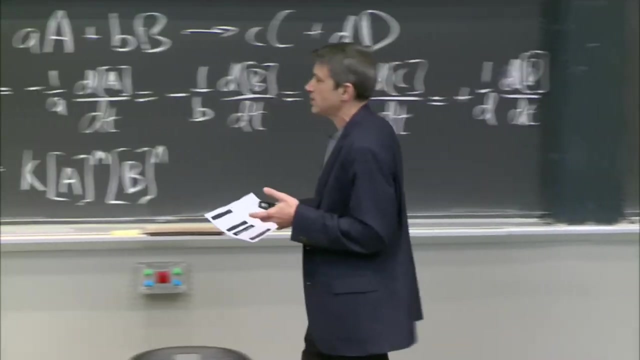 If I had a linear plot with log concentration versus time, you know it's first order, Right, And you know that from the integrated rate law. Now, if you have data, how do I know what the rate law- I'm sorry- what the reaction order is? 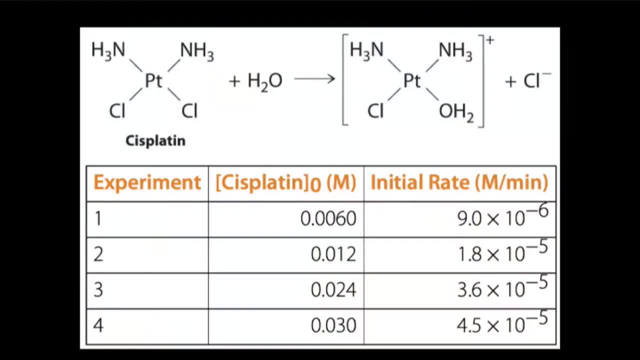 Often you'll just have data. You study a reaction and you get data. Here's a very important reaction. This molecule is called cisplatin. Now, cisplatin is maybe the most used and one of the Certainly very most important chemotherapy drugs. 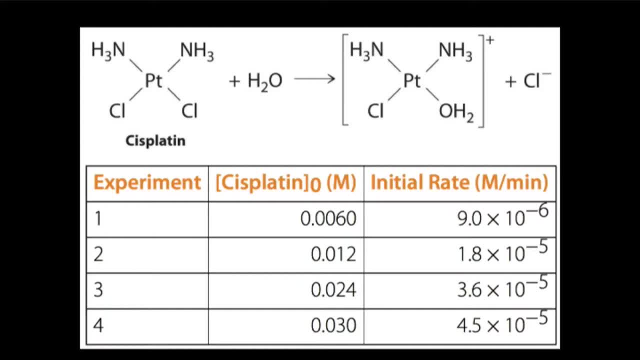 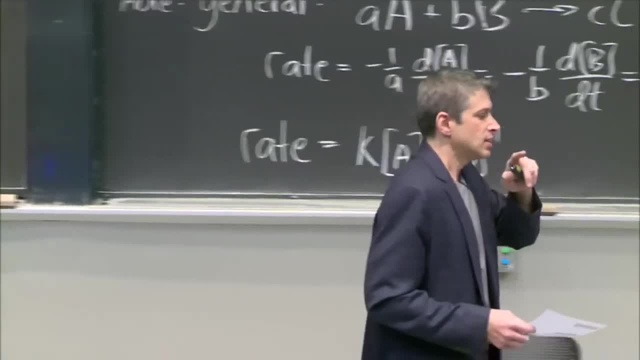 But it's not active in this state. with the two chlorines there, You've got to get one of them out and put a water molecule there so that with the water molecule it can go and damage the DNA of the tumor. That's the idea. 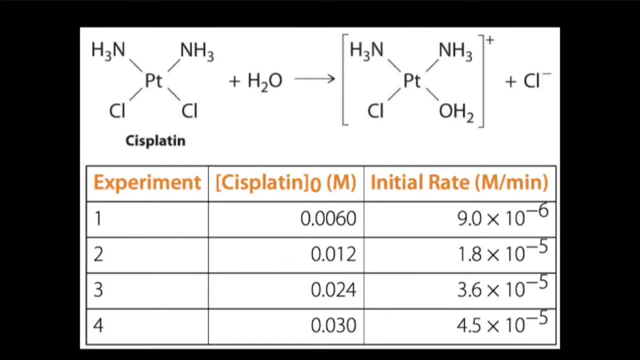 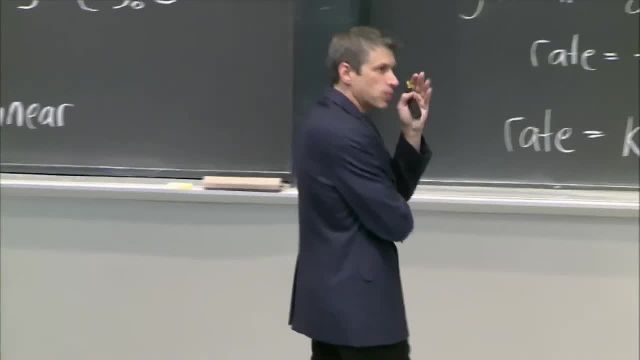 And it can't do that unless this reaction happens in the body, And so you can imagine that this kind of reaction is extremely important. What, And the rate is extremely important here. This has to happen in a time frame that we know very well. 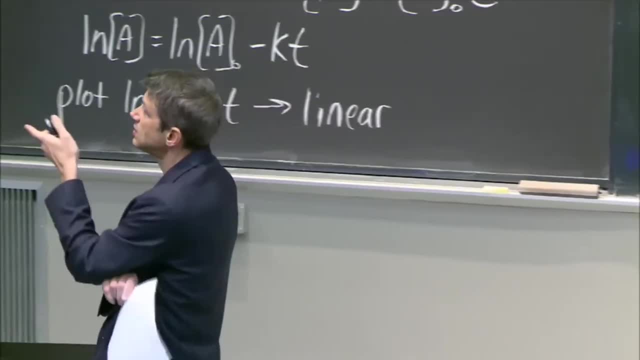 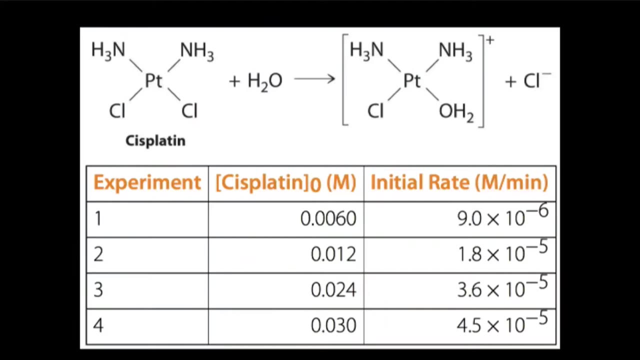 So this rate has been studied very carefully for this reaction And you can see- OK, you can write down numbers- How much did I start with and what was the rate. And I'm watching the rate change Right away. you know the rate changes. 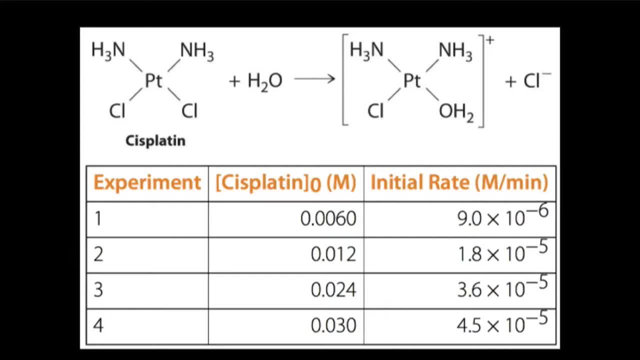 as the cisplatin concentration changes. It's not zeroth order, Right? And the second thing you know is well, if you take any two of those and you take ratios, then the ratios are the same. So it must be first order. 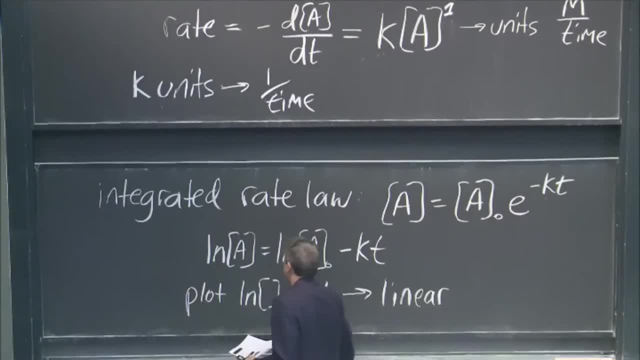 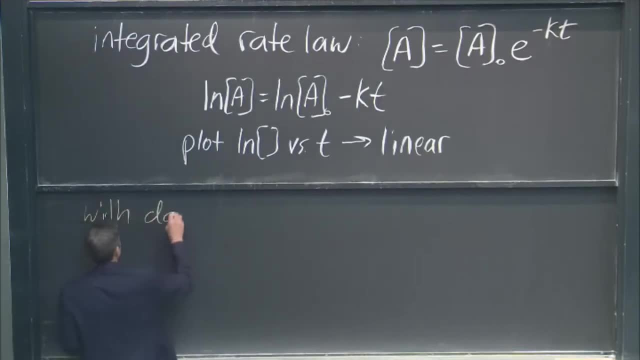 That's one way to know what order you have. So, if I have data. so with data like that, with data, you could do this. You could take ratios At two different times, And what does that get? It gets you the order. 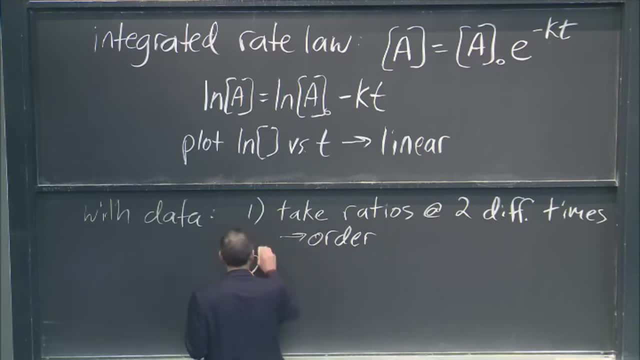 From that you can get the order, And we'll see another example. And then you can go further than that, because then I could plug in data from one of the times. Right, I could use data. Once I know the order, I could use data from one time. 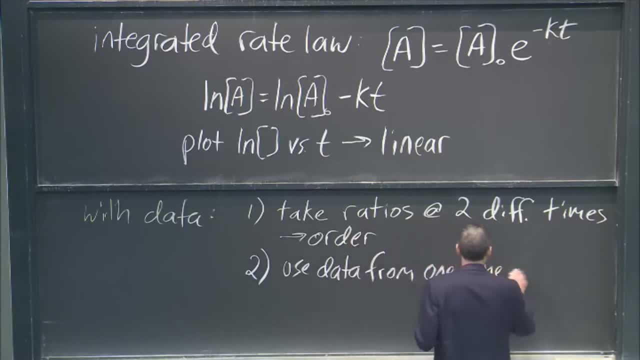 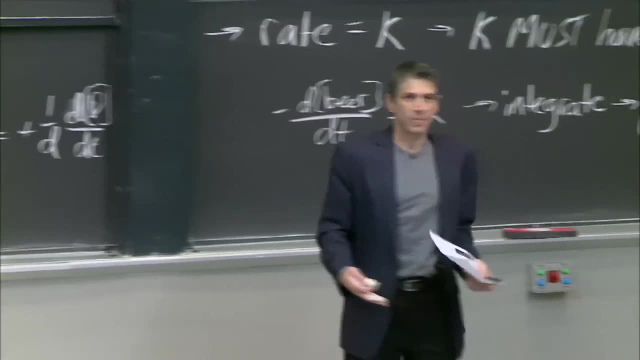 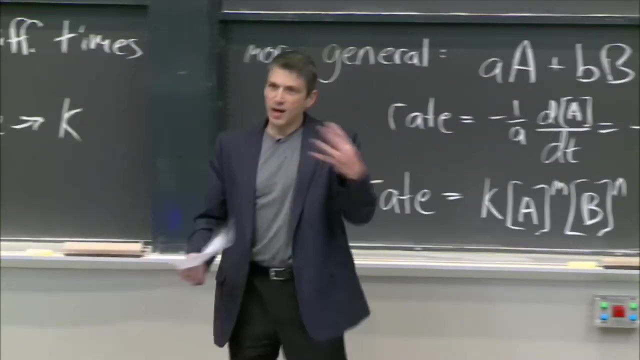 from one time, And then I could use any of these lines to get k Right, Because once I know the order, I know how to write down the rate law, And then I can use any of these lines to get k Right. 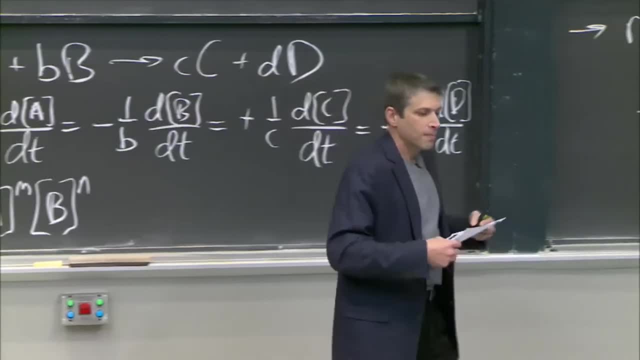 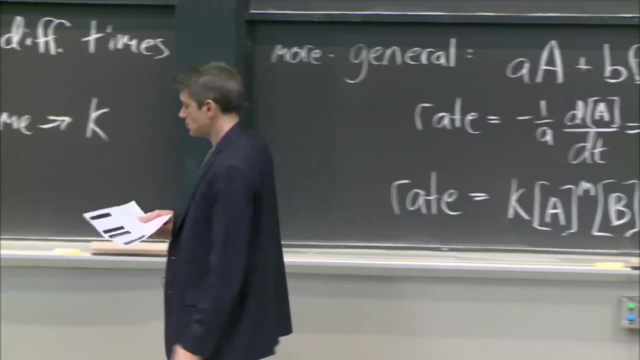 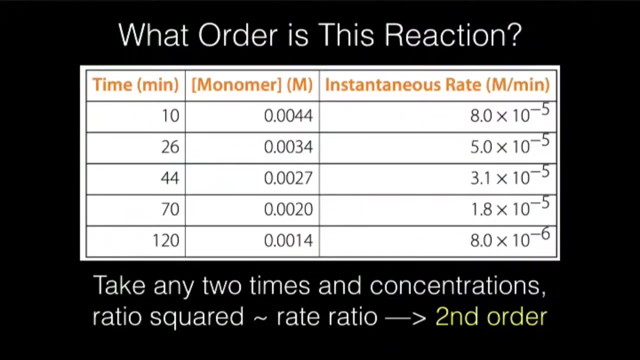 So we want to be comfortable with reactions, with rates going back and forth between order rate law, integrated rate law- plots Right. Integrated rate law- Plots Right. So if I had data that looked like this, I could do the same. 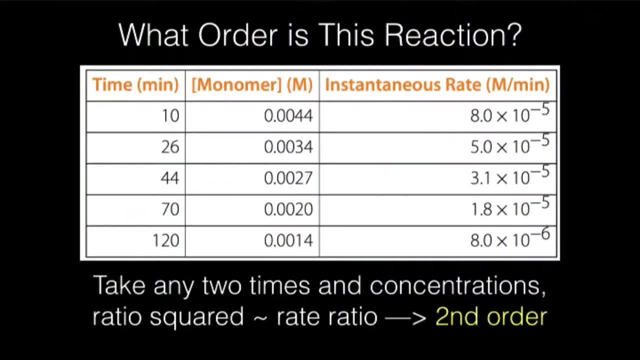 Here's another reaction. I could say: what order is it? Well, I'm not going to do it. So you take any two times in concentrations And what you have is that the ratio squared gives you the ratio of the rates. That means it must be a second order reaction. 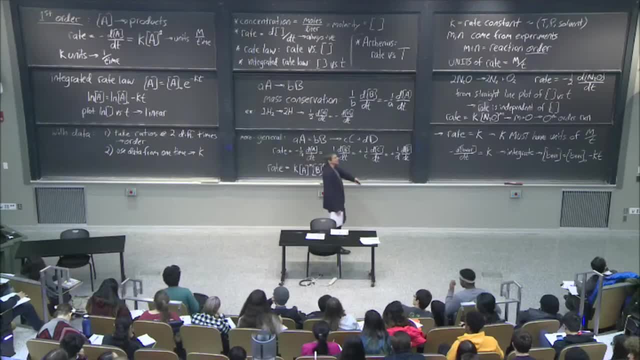 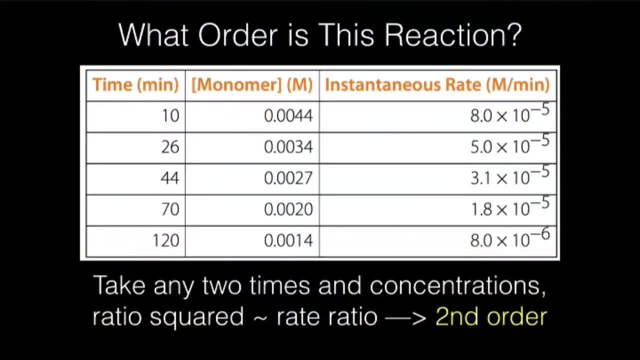 It means it must be Right. I had something that went into products and the dependence of the rate From this data. the dependence of the rate is that something's concentration squared. You can see it from the data. So let's see. 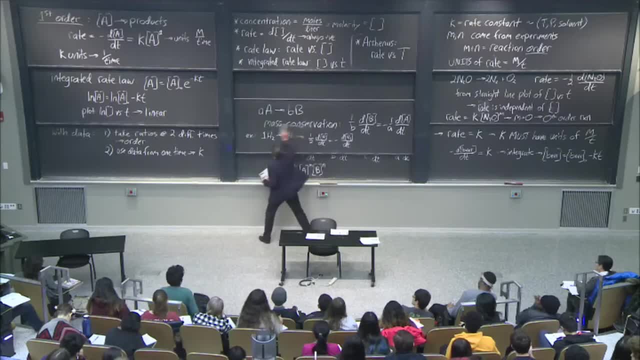 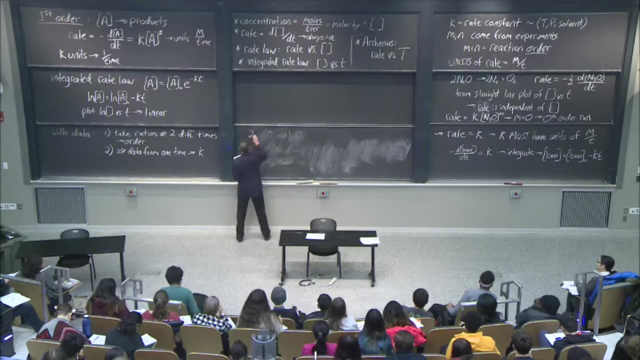 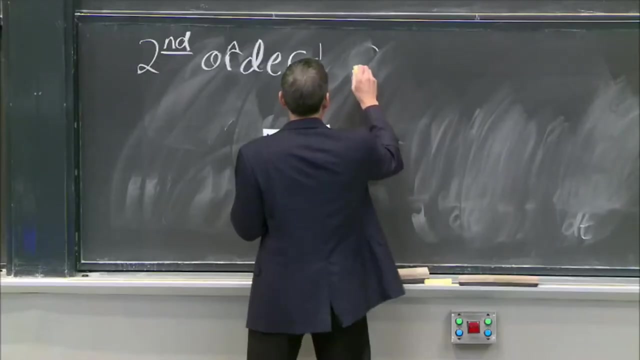 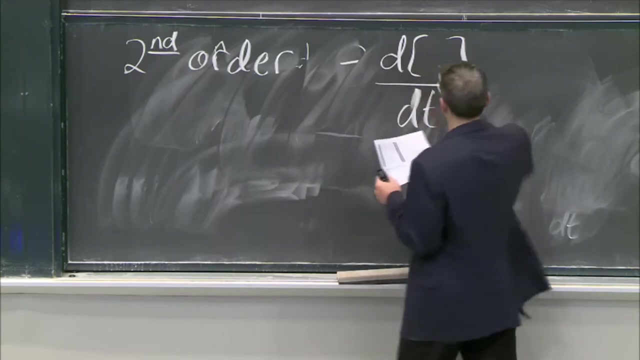 I'm going back to the middle here. OK, So now we just went to second order. So, for second order, what do you have? Well, you have that minus d of something, some reactant, And I just got one reactant here. 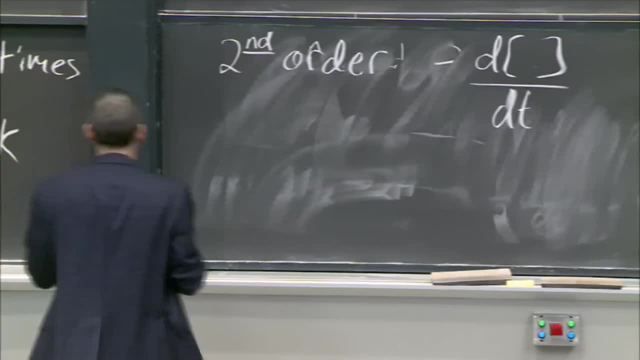 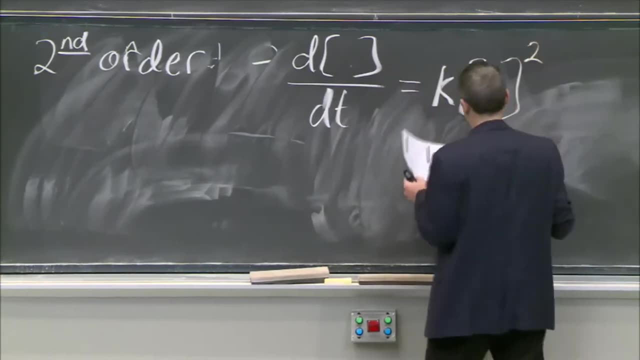 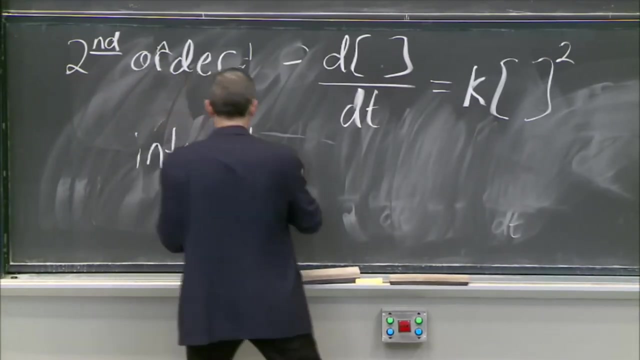 You think about it as A, So the same thing. A went to something. OK. So minus the change in concentration of that with time is dependent on k times the concentration of that squared. And if we integrate this one, integrate, then what do you get? 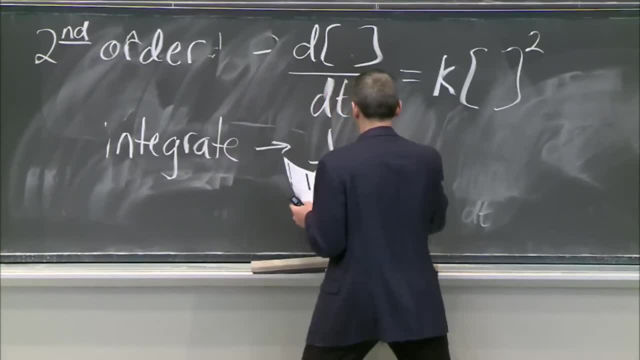 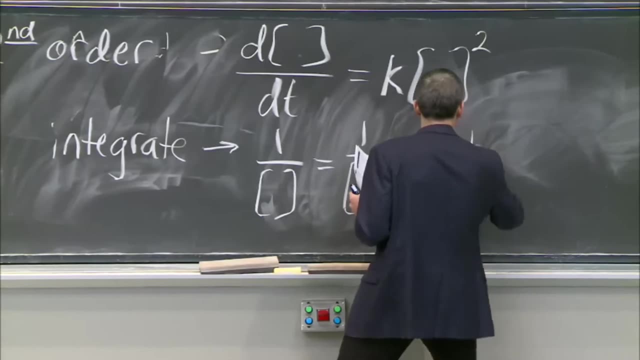 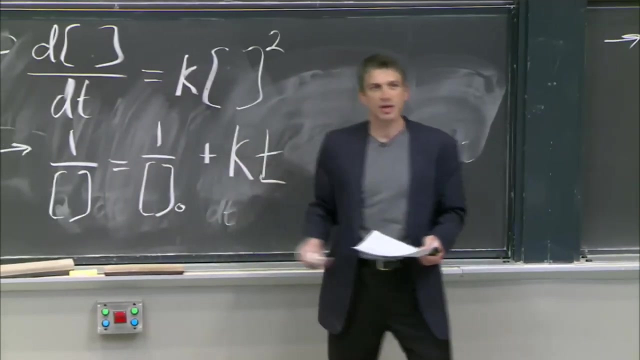 You get 1 over the concentration of the, something equals 1 over its initial value plus kt. Oh, you can see that. Take the t over here and take this over there, and then that's going to be the integrated rate law. 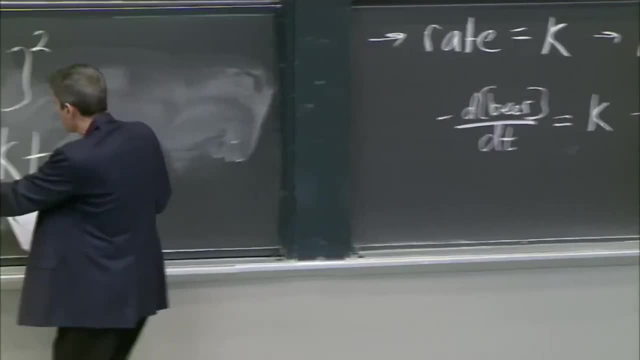 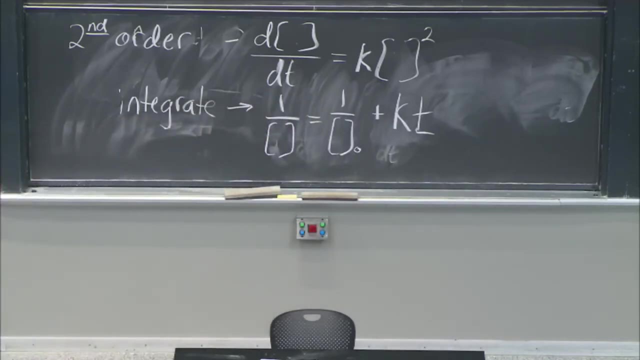 So now look at that. What do I plot? to get Linear? I've got to get to linear. I don't like curves in reaction rate plots. I like linear lines because the linear line will tell me something about the reaction order. 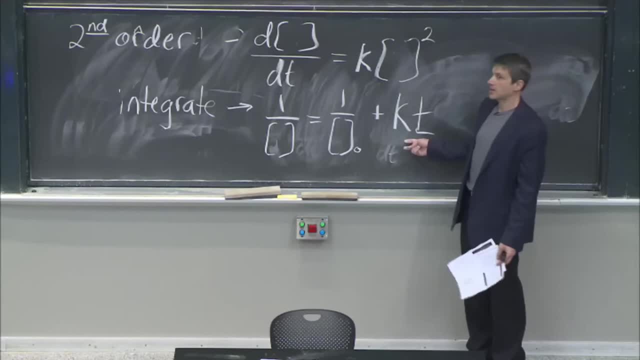 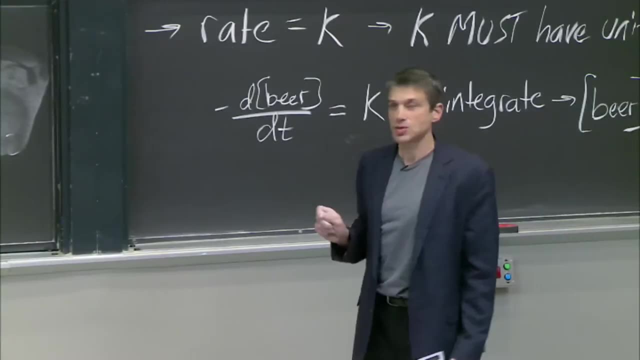 And, by the way, the slope could tell me something about the rate constant, And so if it's second order, the plot that gives you a linear line is 1 over concentration versus time. So let's say I had this data and I tried to plot it. 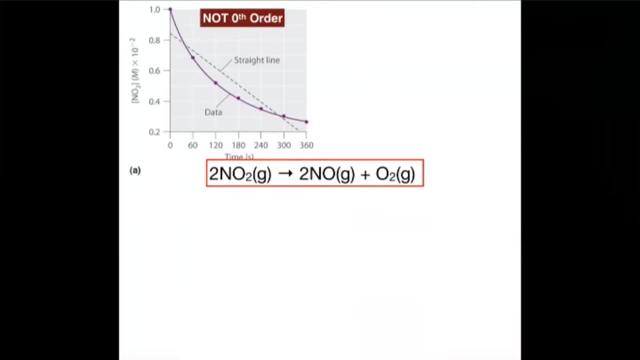 The first thing I do is I say, well, OK, hold on. If I plot the concentration versus time, that's what it looks like, Not linear. That means it's not zeroth order. Well then I plot: OK, I'm going to take the same data. 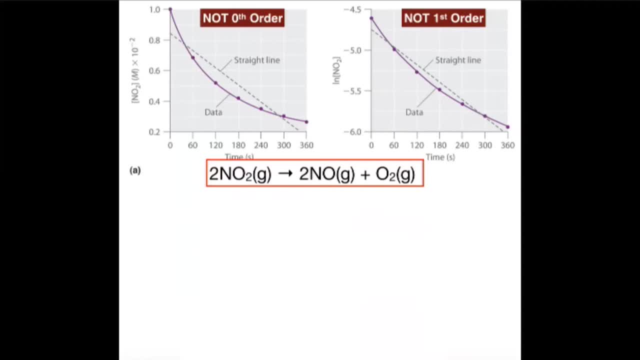 and I'm going to plot the log of it versus time. Not linear, Not first order. But if I plot 1 over that concentration versus time, it gives me a perfect linear fit. So it must be second order. Plots order. 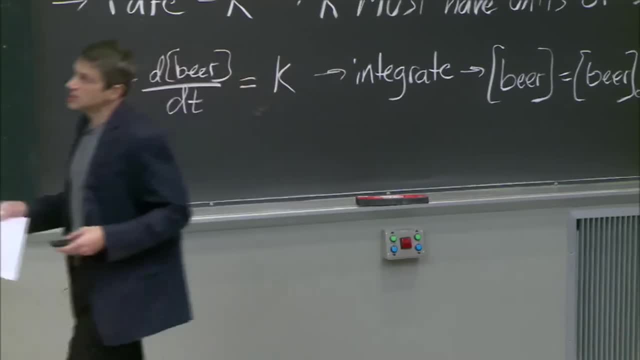 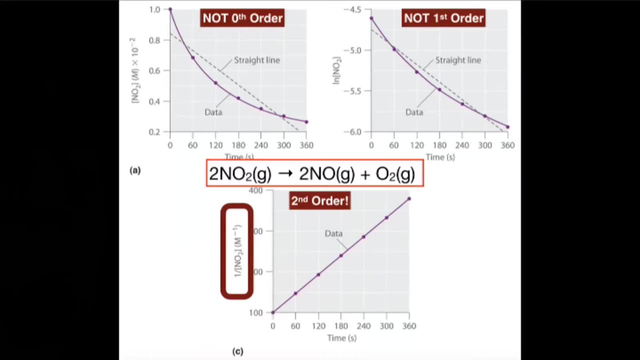 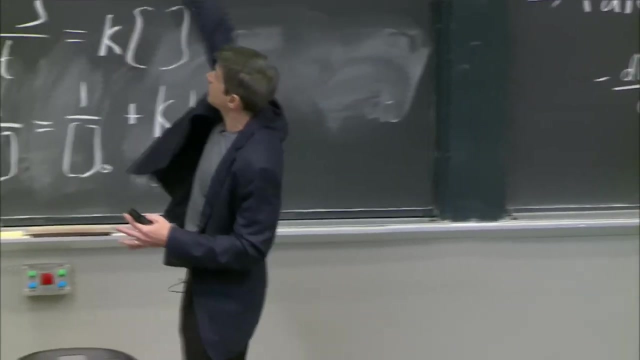 Linear, And so we're not going to go beyond zeroth, first and second order, because what I want is for you to feel your oneness with reaction rates and kinetics through these three orders- zeroth, 1 and 2, and through these different concepts that are up there. 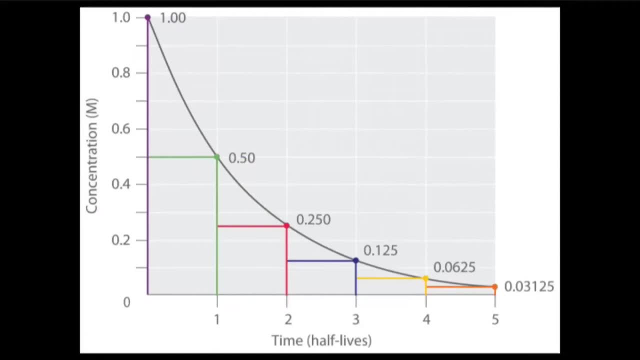 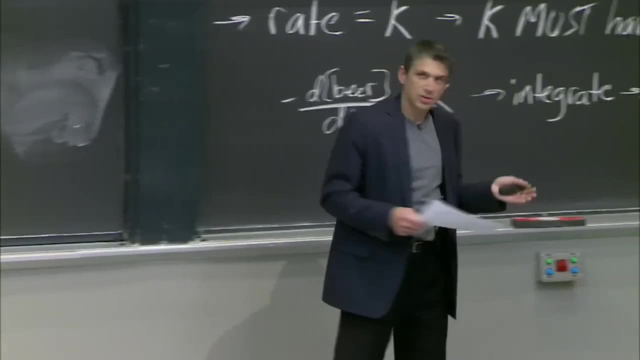 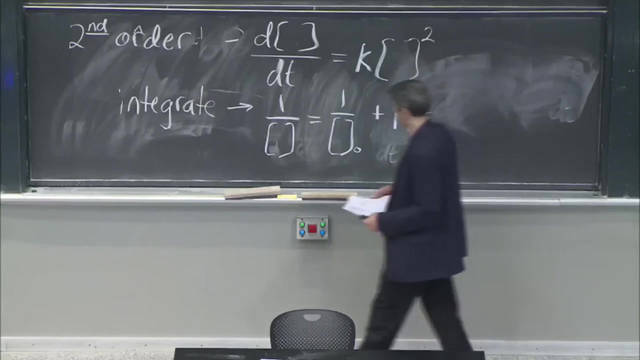 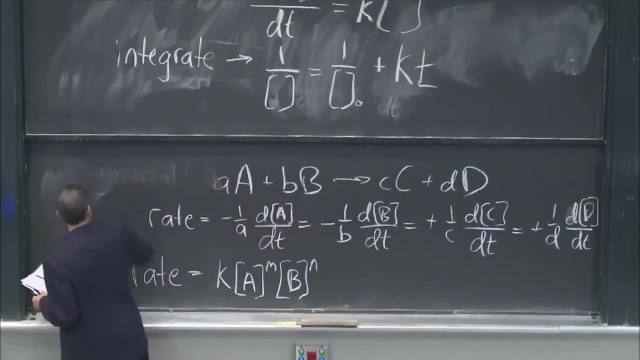 So one more thing you can do before I turn to temperature. One more thing you can do with, once you know the rate law, is you can calculate how long it takes for the concentration to be cut in half. If I know the rate law, then I can calculate the half-life. 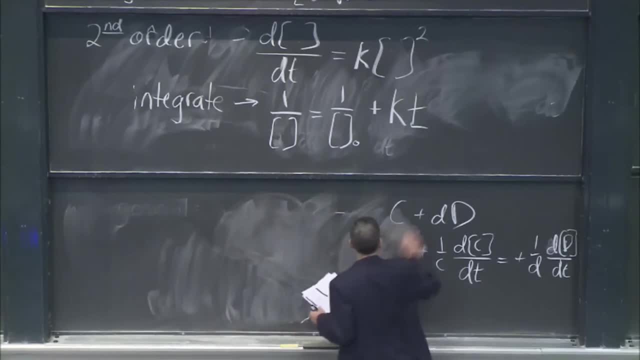 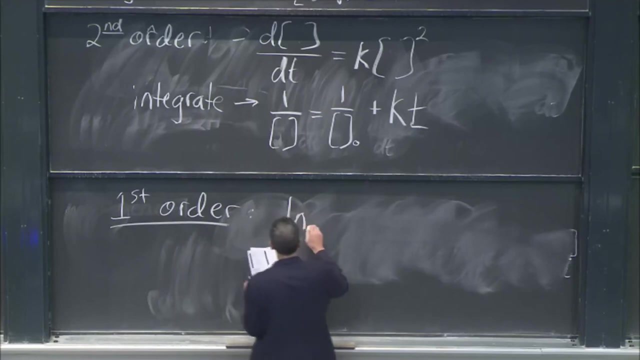 That's what that's called. So for example, if it's first order, let's suppose it's first order, Then the integrated rate law. I'm just going to put the two concentrations on the same side here: A over A0.. 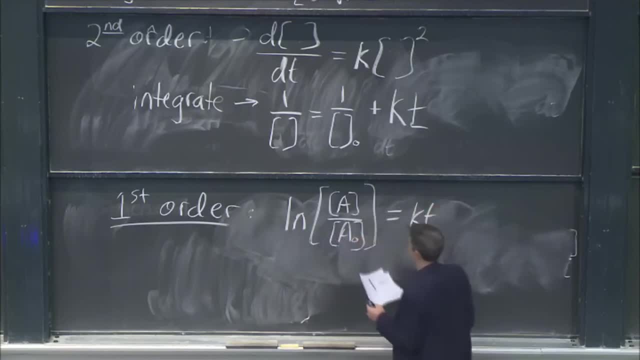 So the integrated rate law gives me this. It's just what I had before somewhere. But you can see well, what if A? what if the concentration of A is exactly half of the beginning concentration? So when A equals 1 half, 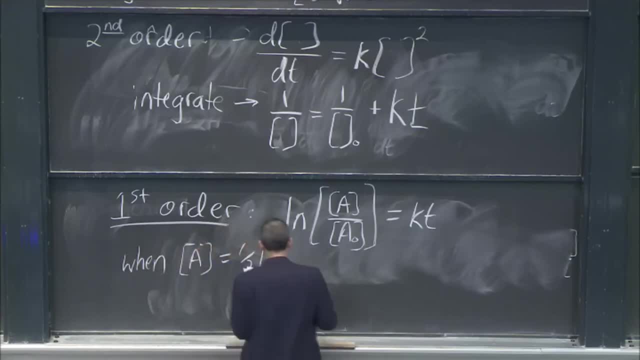 The initial concentration, but then this becomes a half right. So if I want to know how much time it takes to get to half, that's a good thing to know. just in general. How long do I have until half of this is left? 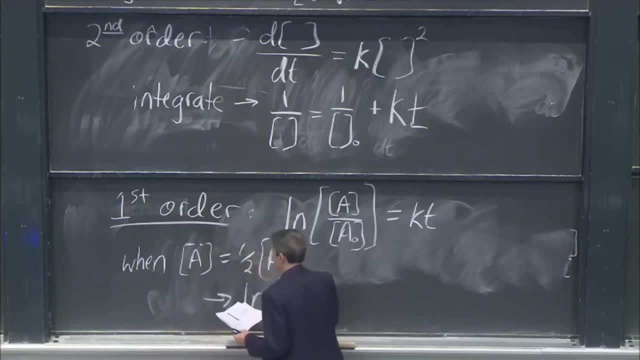 Well then you know that this is going to give you log 2, right, When A equals 1, half A0, then log 2 equals K0. T, and we're going to call that an important. it's not just any time it's called the half-life. 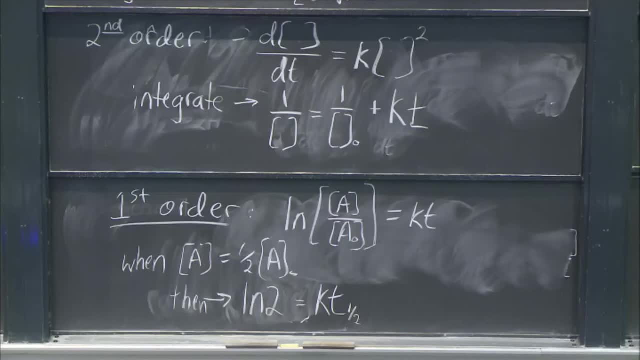 It's the time that it took to get to A being 1 half of the initial And the half-life. so I've got it right, I've got it. I've got the half-life. The half-life is a very powerful tool. 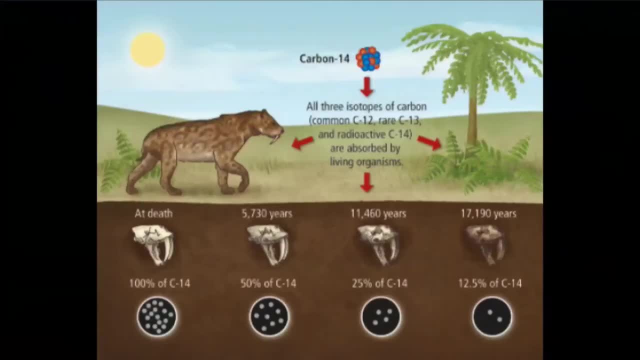 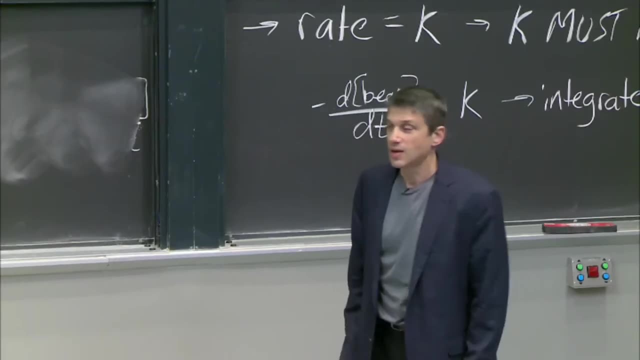 A number of you may have heard of carbon dating. This is just a picture of wild animals, But see but what happens. Those wild animals breathe in oxygen and other stuff from the air, Including stuff that contains a spread of carbon atoms. 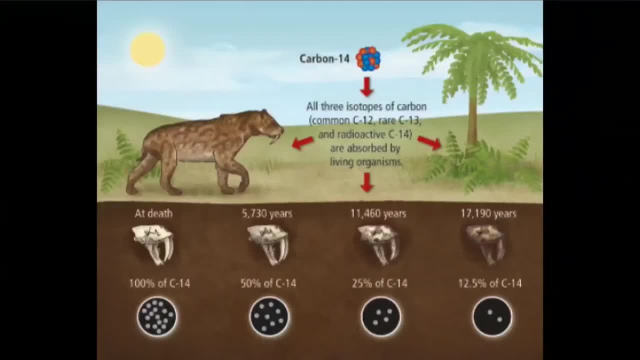 And we know carbon has isotopes. We know about carbon's isotopes. We've already talked about them: C12, C13, C14.. C14 has this wonderful thing about it that it radioactively decays, And it turns out that there's a certain concentration. 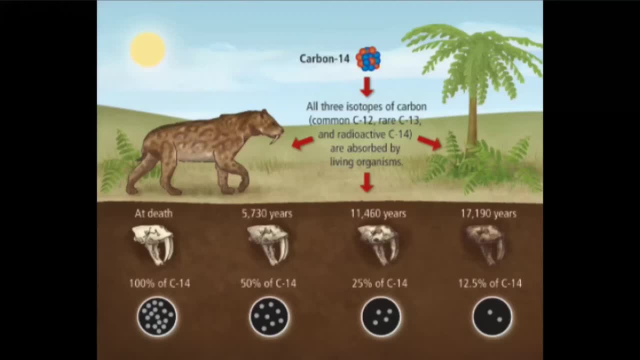 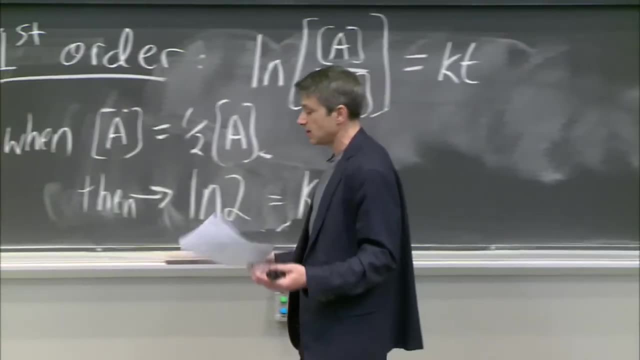 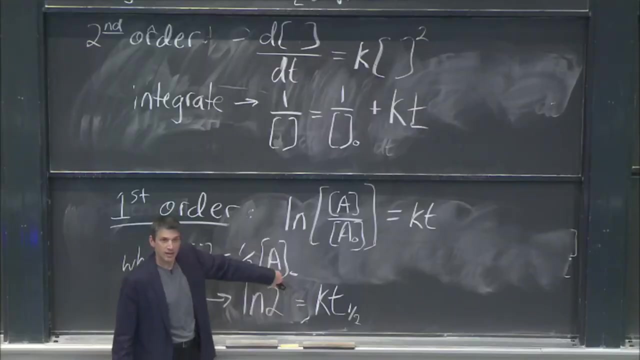 of that in the atmosphere at any given time And we can go back in history and know how much concentration there was in the atmosphere And we know if these animals are breathing it in. we know that they should have that concentration at A0.. 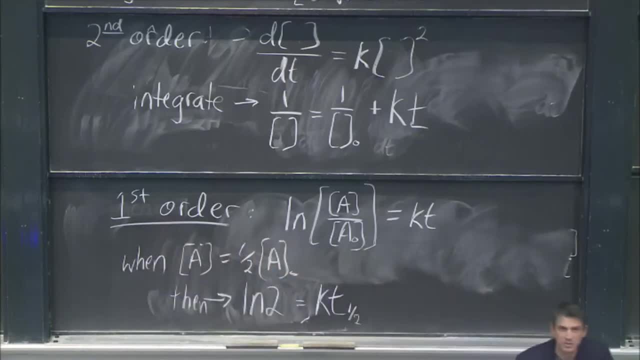 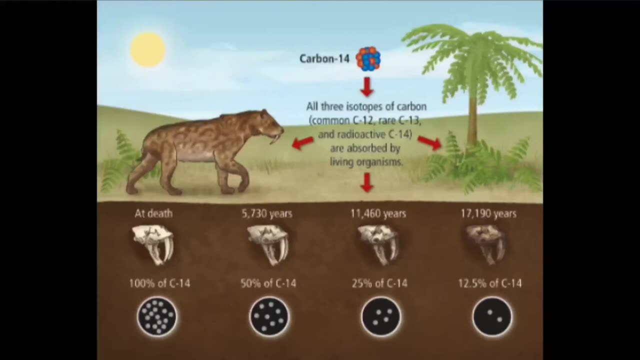 Except this isn't a concentration. This is a number of atoms, But it's OK, It still is a first-order process. The radioactive decay of C14 is a first-order process, And so because of that, we can date things using carbon dating very accurately. 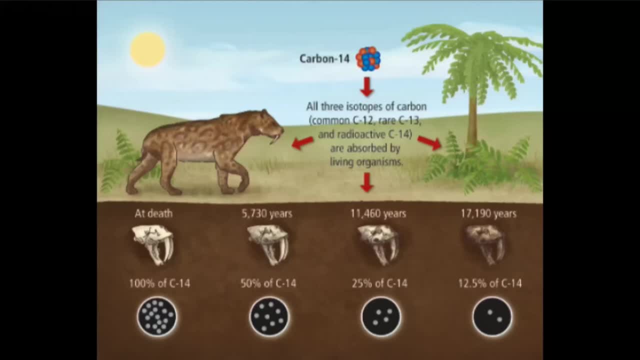 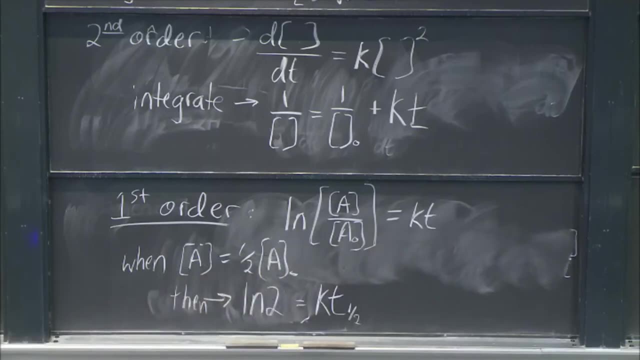 So this is a really awesome thing. OK, Thank you, Have a great day. Thank you, See you. awesome tool that relies simply on the half-life, on knowing the half-life. All right, Here's a summary that I thought would be useful. 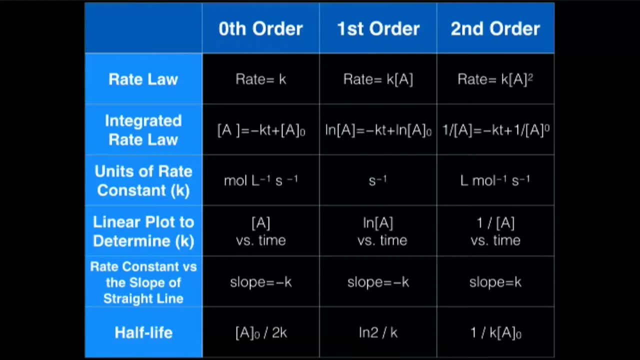 This is it. This is everything we just talked about before we switched to temperature Rate law. zeroth order, first order. And you're all like: why did I write this all down? It's all on this page. No, it's good to write down. 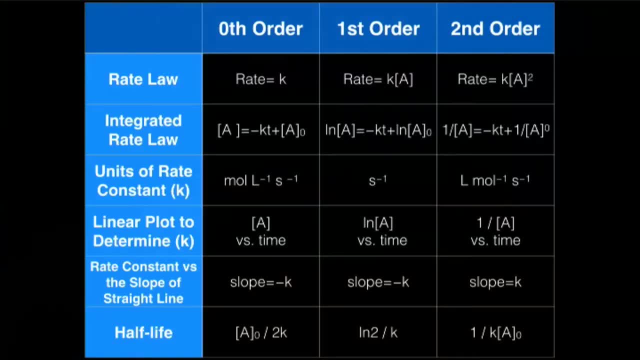 It helps you think about things. But here it all is. There is the zeroth order, first order, second order, Integrated rate law- that comes from that. The units of the rate constant, The linear plot to determine the rate constant. What gives you what the slope of that line is? 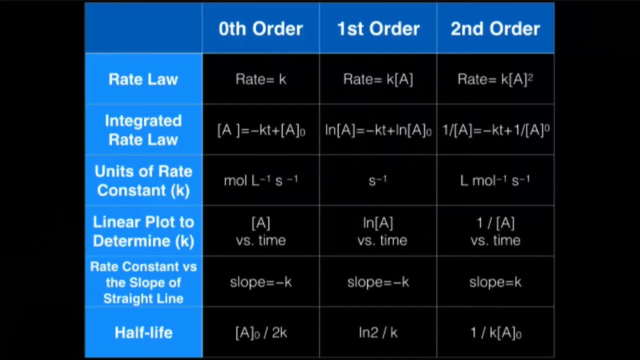 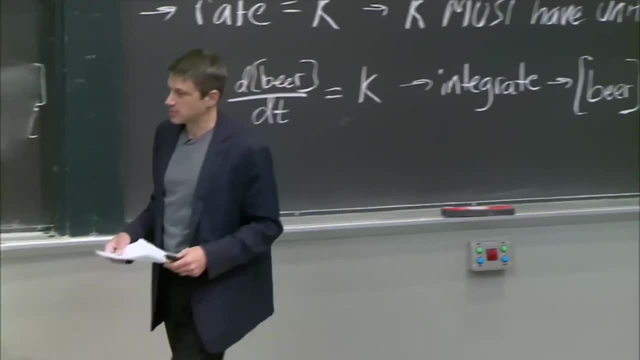 And then what the half-life would be if you just follow this for the other two orders. So this is all that we just talked about, And the best way to fill your oneness with this is to do some practice problems more than what we've just done. 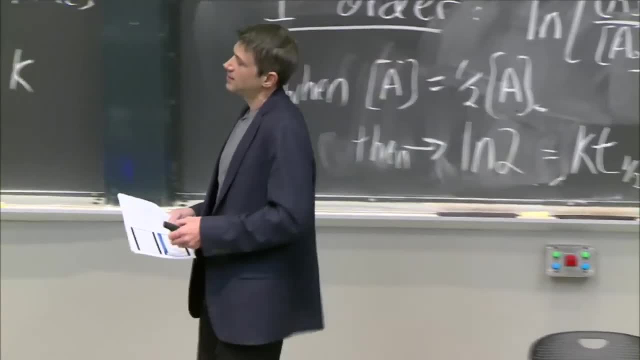 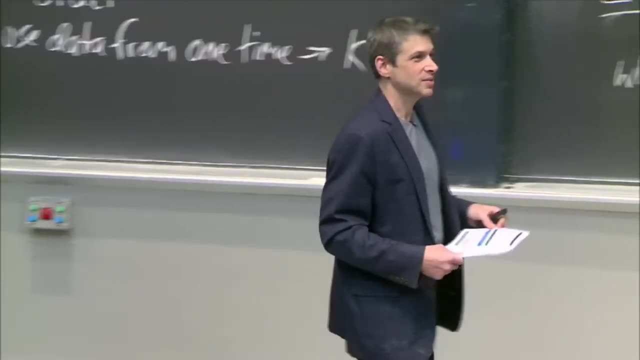 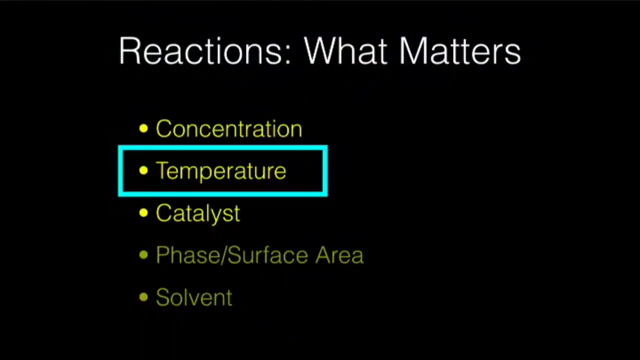 The next topic. I'm not going to spend the same amount of time on temperature and catalysts, obviously, But I want to mention how these impact reaction rates. We're talking about how fast the concentrations change- And to do that, what we're going to do, 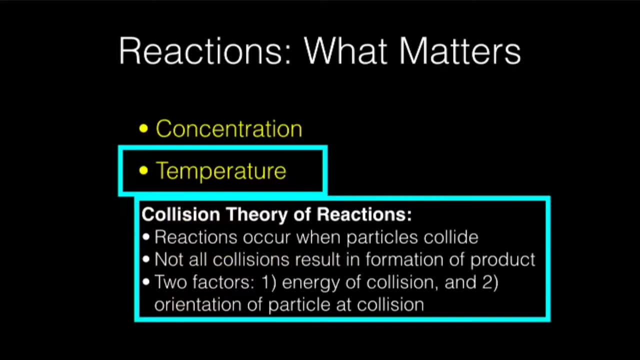 is. we're going to use the collision theory of reactions And I've just written it down here what it is. What is the collision theory? What is the collision theory of reactions? What it is is it says that they occur when particles collide. 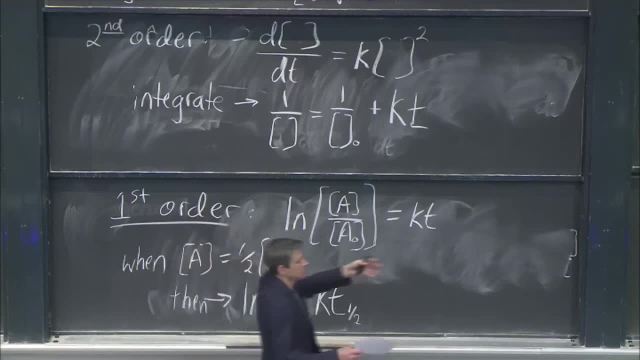 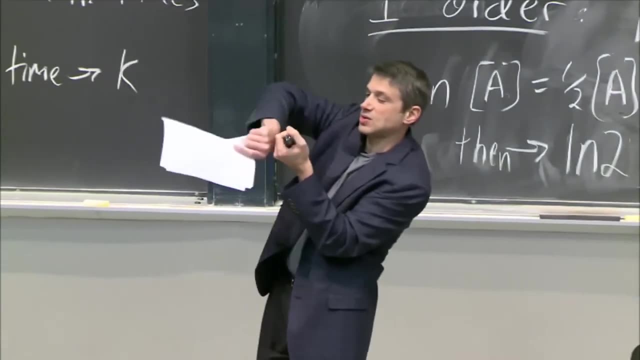 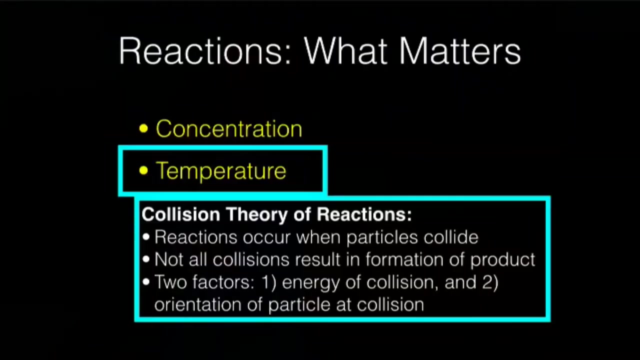 Why does A plus B go to C? Well, because things collided into each other and they got close enough, Or they maybe had the right orientation so that new bonds could form or others could break. And the theory also says that not all collisions result. 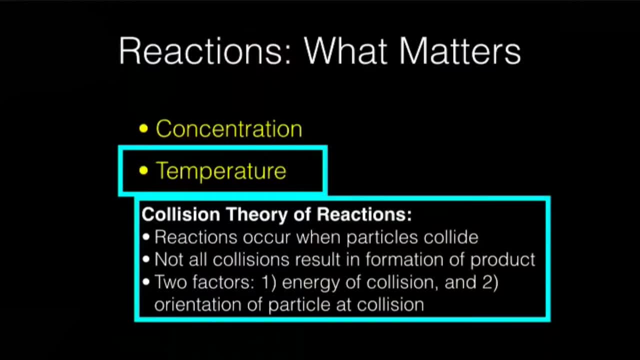 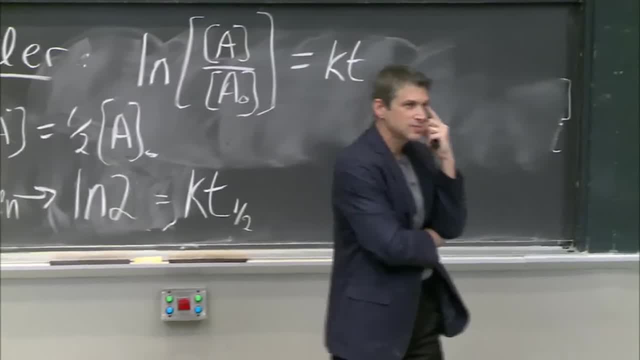 in the formation of product and that there are two factors that matter: The energy of the collision and the orientation of the particles. So I want to highlight those two factors. So, energy of the collision: We're going to start with the energy of the collision. 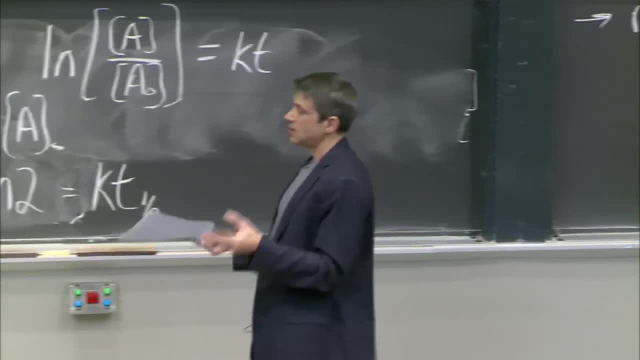 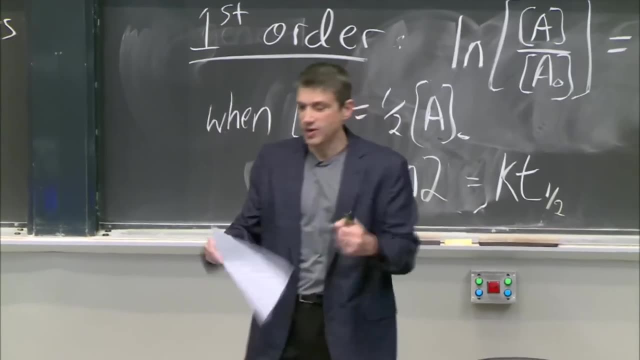 And we're going to talk about that in terms of where do you get that energy? You get it from heat. You get it from thermal energy, which means these things are vibrating and moving. Maybe, if it's a gas, they're bouncing off. 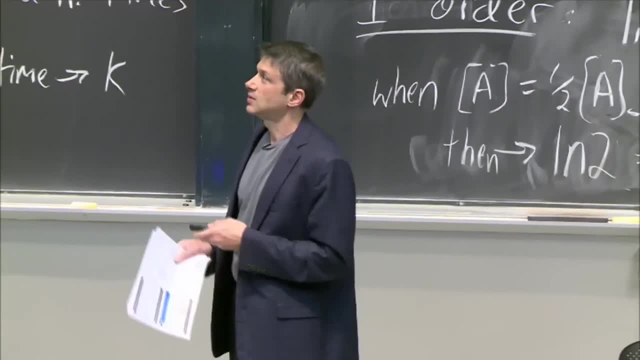 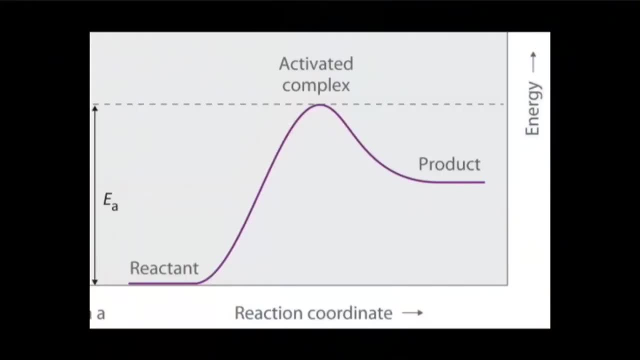 of the walls of the container, That's temperature. How does that matter? Well, in order to understand how that matters, we have to think about This, and this is what collision theory for reactions tells us to do, is to think about a reaction in terms. 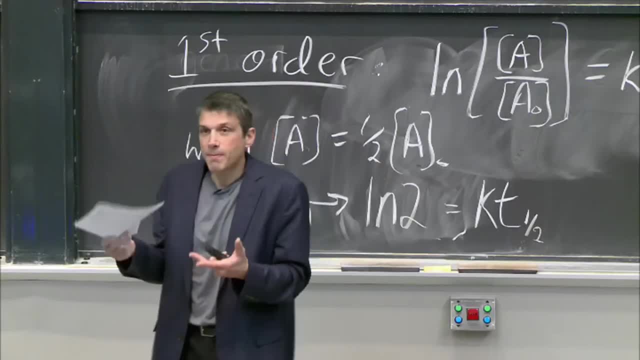 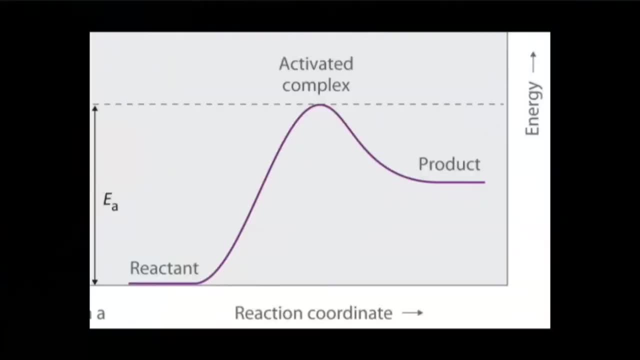 of an energy landscape and an energy barrier that you have to overcome. So here I have this Ea, which is the energy that it's going to take. I need to put that energy in for the collision to be strong enough. Think about it as like, well, I just kind of didn't collide. 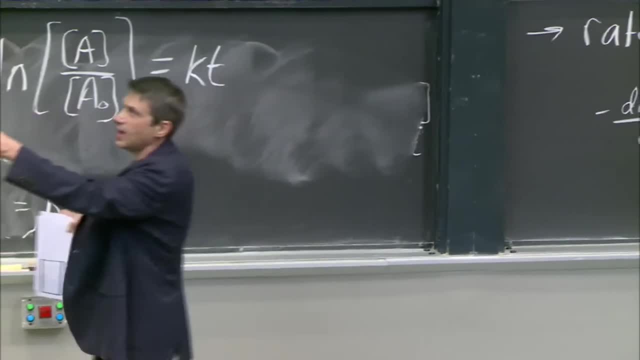 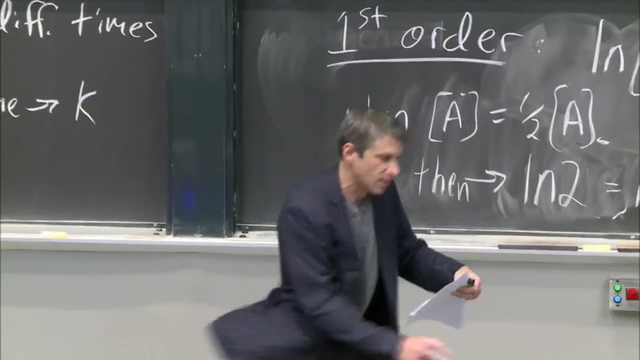 I had a very low energy, So I'm below Ea And I can't get over this hill. It really is, think about it, like pushing a car. Did I push it hard enough so it can go over the hill, Or is it just pushed a little bit? 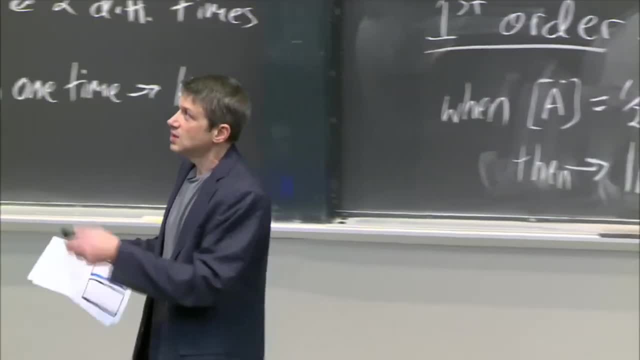 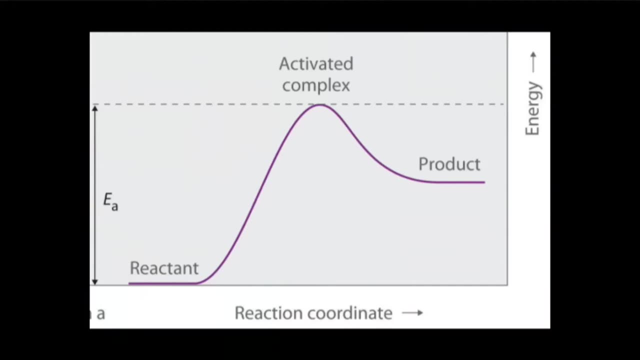 That's the kinetic energy we're talking about. Could it get over that hill? Because what we're saying is that for this reaction to happen, there's some amount of energy that's needed. That's the activation energy. That's the activation energy. 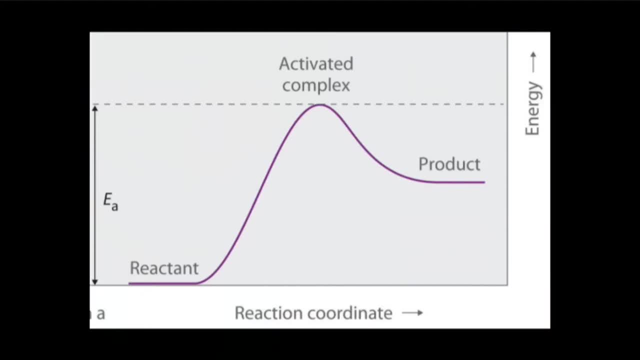 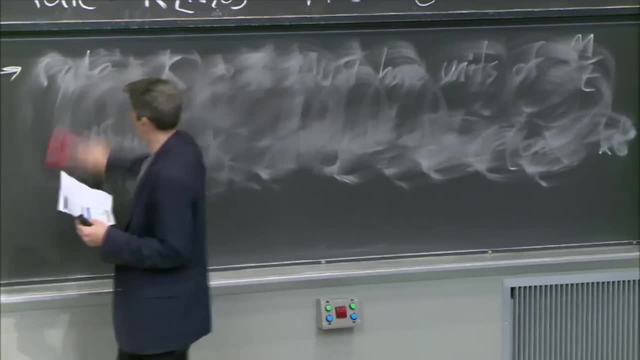 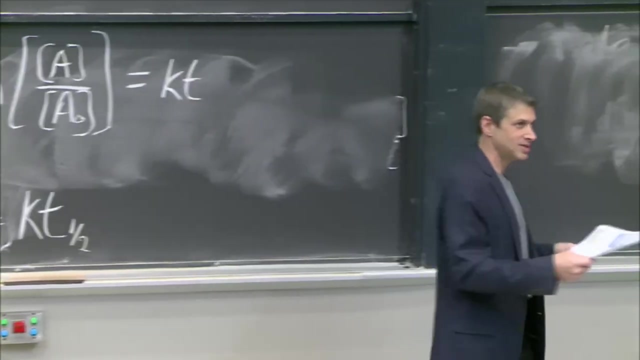 OK. So what does that mean? Well, first of all, you should all be feeling something right now, And you know what I'm talking about. I'm talking about Svante, Svante Arrhenius, right, Somebody said it. 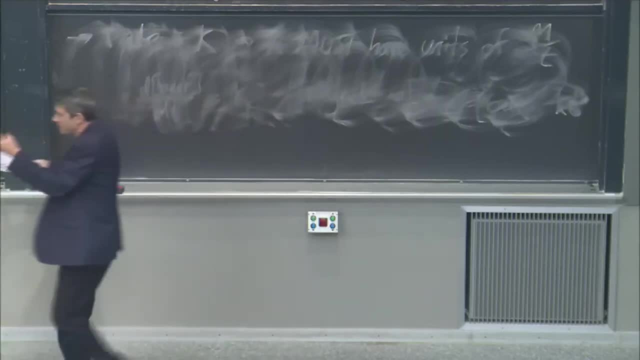 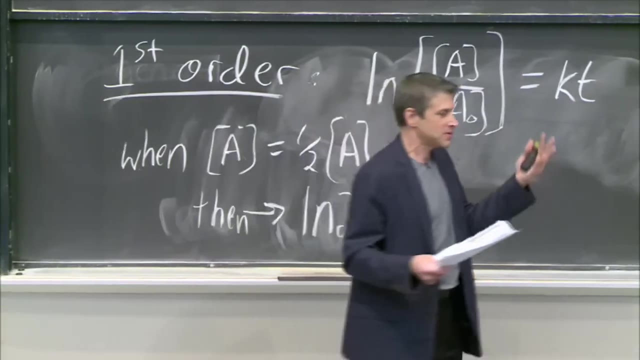 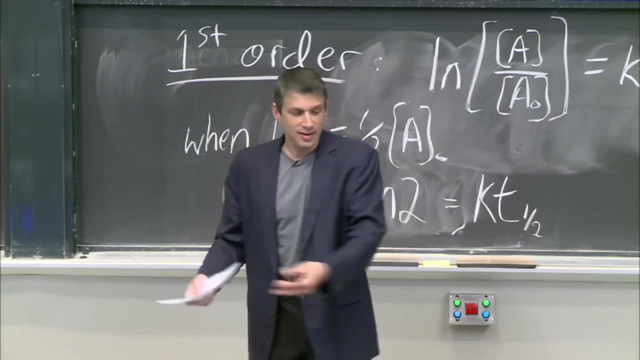 You were feeling it. Why? Because I'm talking about a process that has a barrier that is thermally activated. a process that has a barrier that is thermally activated, Svante Arrhenius: crickets, crickets and then. 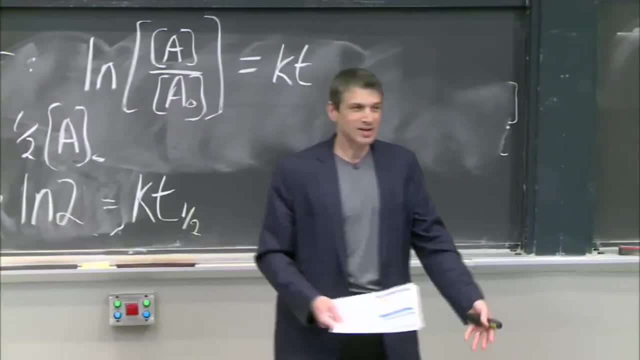 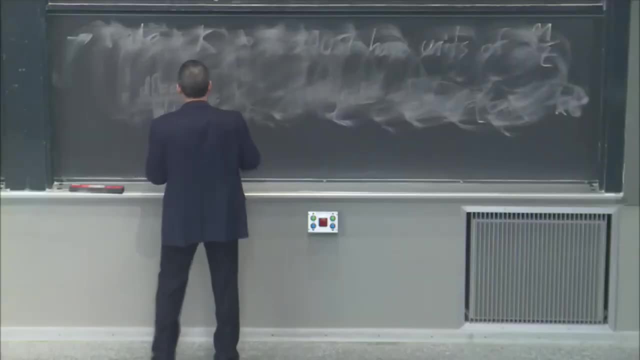 intrinsic carriers: activated processes, reactions- They have a barrier, They have a barrier. Now here's the thing, though: Ea is typically maybe an electron volt, And we know that KBT is 025 electron volts. We've talked about this before. 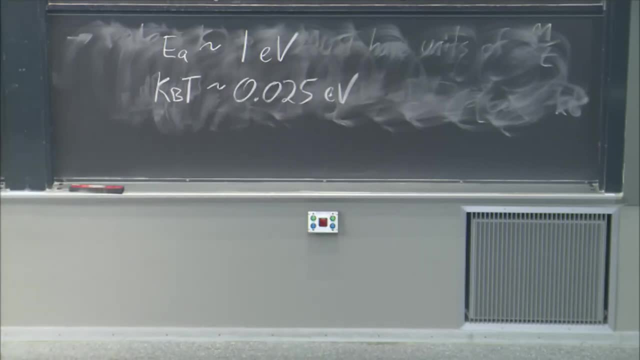 And how is that possible? It's the same as what we talked about before, because this comes: this is an average energy If you put the Boltzmann constant in to room temperature. this is at room temperature If you put the Boltzmann constant in at room temperature. 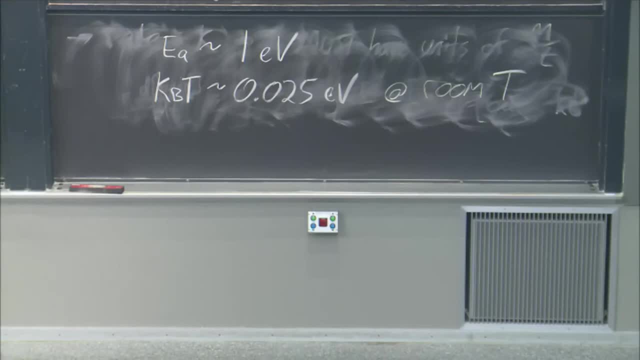 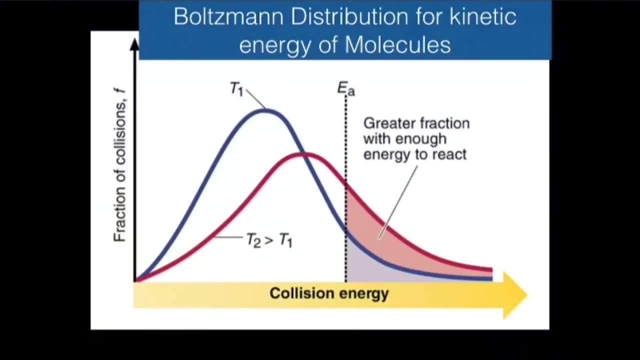 you're going to get that small energy, But we know that thermal energy is a distribution. This is something we've talked about, So here it is again. So this is the Boltzmann distribution. This is the Boltzmann distribution. This is the Boltzmann distribution. 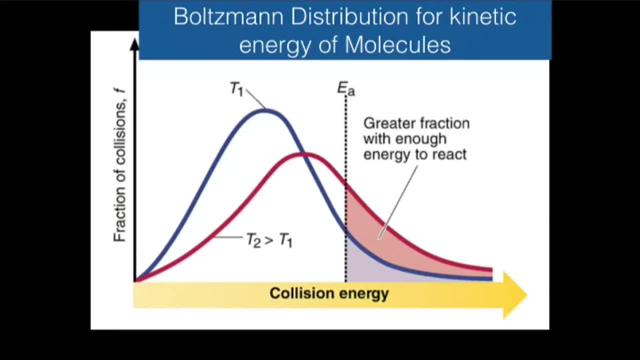 This is what this distribution is called, And if I have my energy for activating a reaction, my barrier for the reaction to happen, shown there with the vertical line. basically, I have two temperatures. So, yeah, KT may be small, but there's some tail out there. 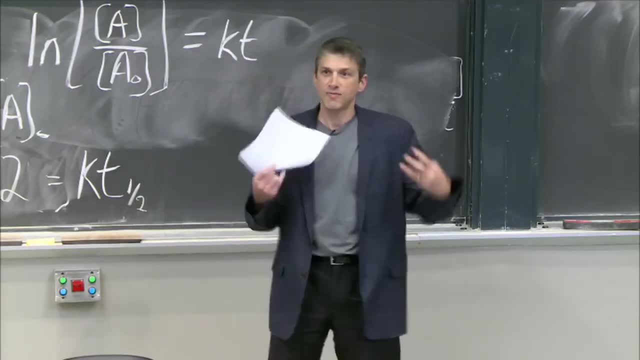 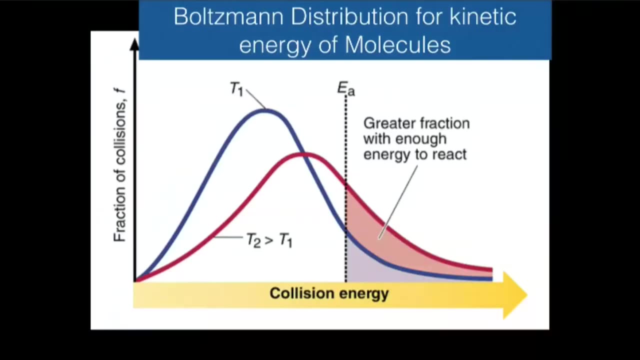 where there is enough thermal energy, there's enough kinetic energy for this collision to lead to the reaction. So those tails, They grow larger and larger. The amount of molecules that have enough energy grows larger as you increase the temperature. That is Arrhenius. 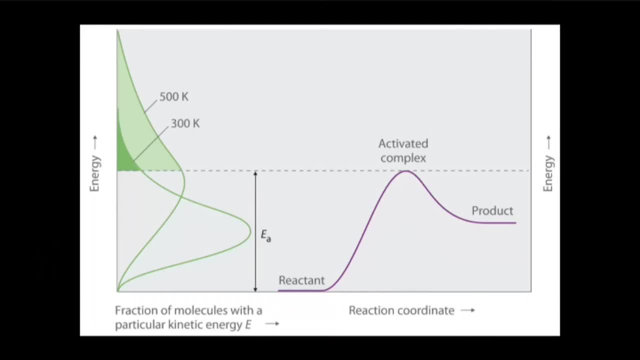 The probability for this to happen grows. That is what Arrhenius gives us, And so here it is mapped. This is something that is in the textbook. that is a nice diagram because it maps the two together. You've got the reactant going to the products. 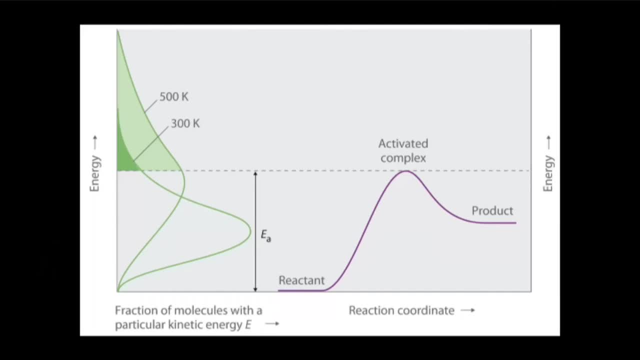 There's an activated complex, It needs that activation energy. and over there we've turned on the side these kinetic energy distribution plots. So you can see, when do I have enough? Well, when I'm over that activation energy, there's going to be some fraction of molecules. 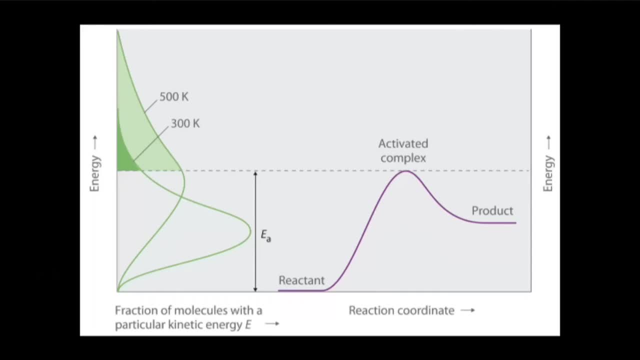 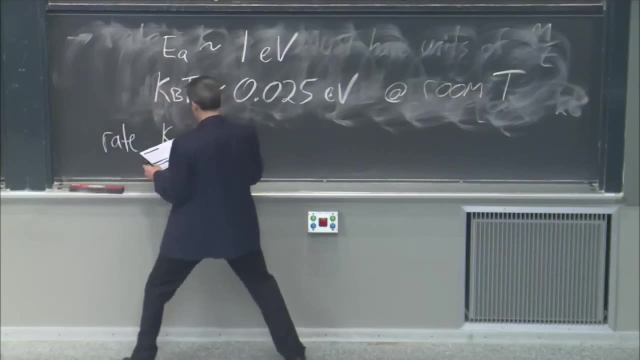 that have enough, and that fraction depends on temperature and that is Arrhenius. And so what we get is that the rate, the rate K, the rate is equal to some constant A times e, to the minus Ea, So that's the rate K over Kbt. 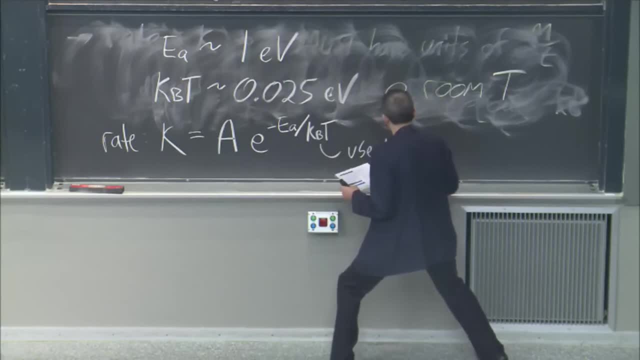 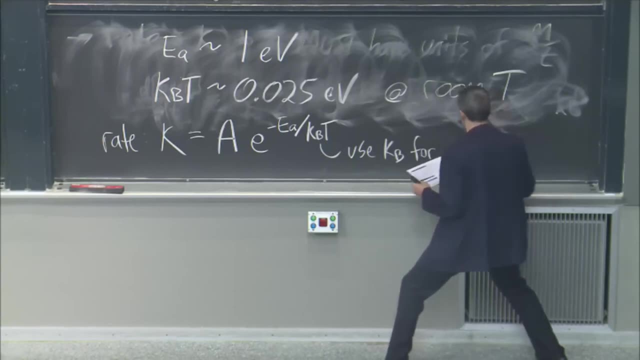 And remember, we use Kb for one collision for a molecule or an atom, And we would use R or R for a mole. Here I'm talking about a single event, one molecule colliding with another to make the reaction happen. Now this is called the frequency factor. 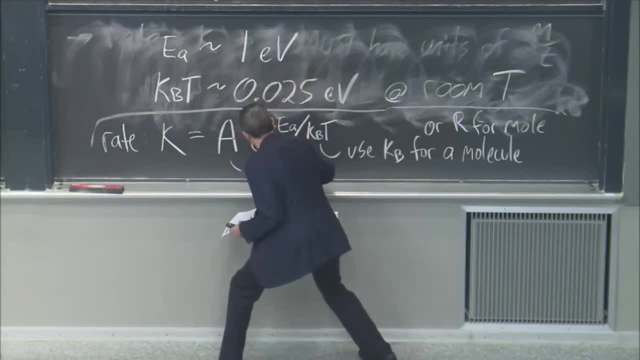 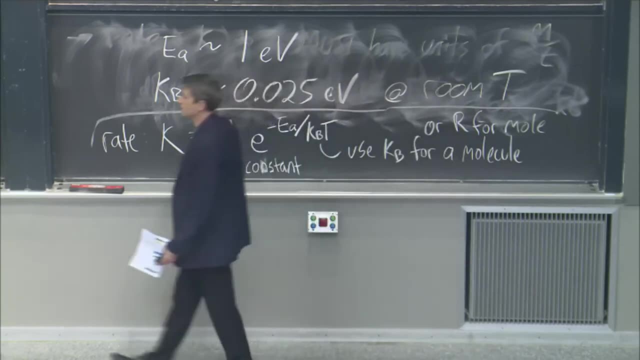 and it's a constant, Constant, constant, And that's something that you could understand. how this might depend on a combination of things, But it's assumed incorrectly, but it's a good enough approximation for us, But it's assumed to be independent of temperature. 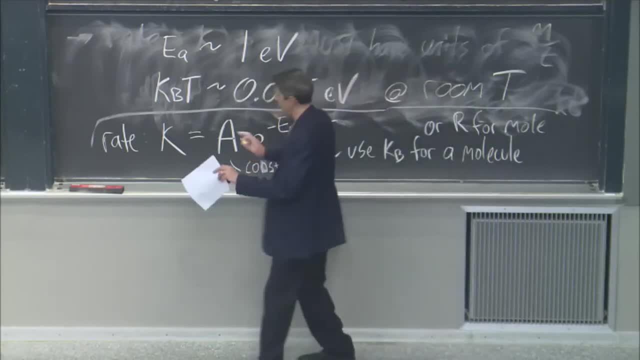 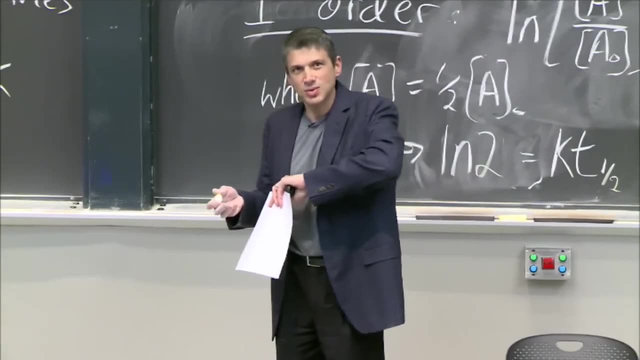 So we pull it out and call it a frequency factor, And it has. It has in it information about whether these things really made the right collision or not. That's what A has in it This exponent, Arrhenius, is telling us. 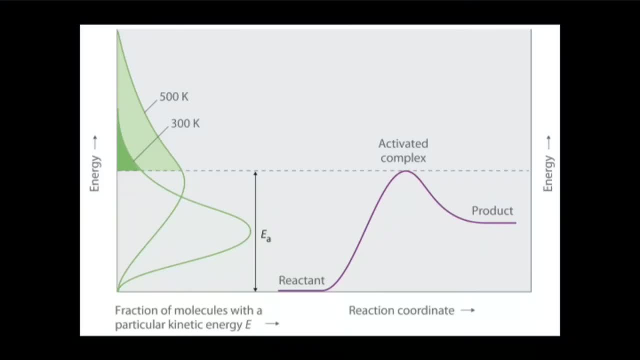 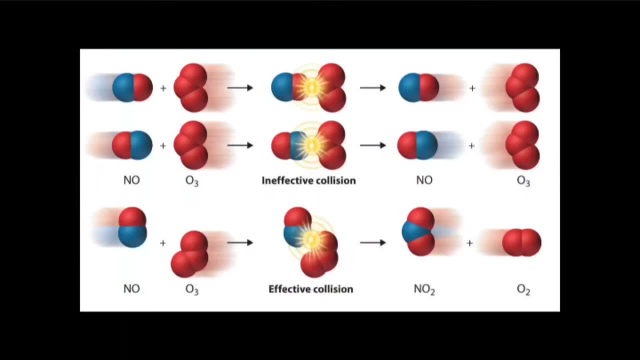 this exponent tells me about that fraction, That fraction, But A tells me about orientation. So here's an example. Here's No plus O3.. And on the top line you can see the No. so the Os are red and the N is blue. 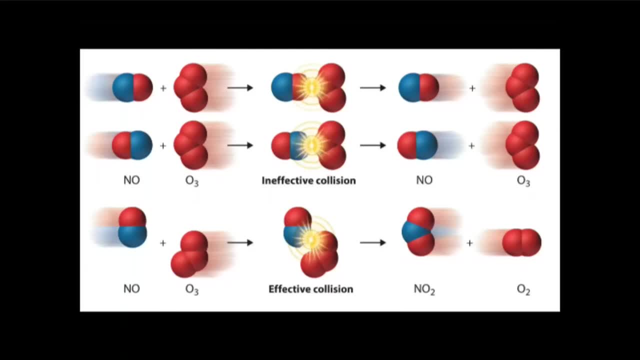 And the No is coming in. but it's coming in either way, whether It's N or whether it's O, it's coming into the wrong oxygen, It's hitting that wrong oxygen And so it doesn't do anything, because the one in the middle 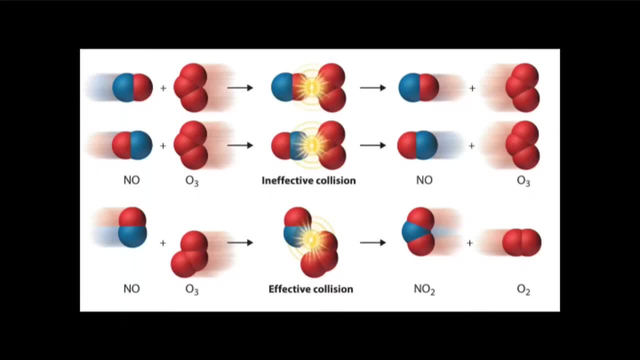 isn't going to be very reactive, not at least at this temperature. But then you've got a different case where it comes in a little differently And in fact the nitrogen is what's coming in and leading the way to that oxygen on the end. 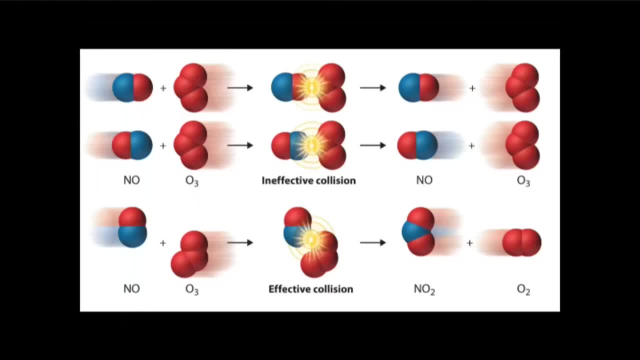 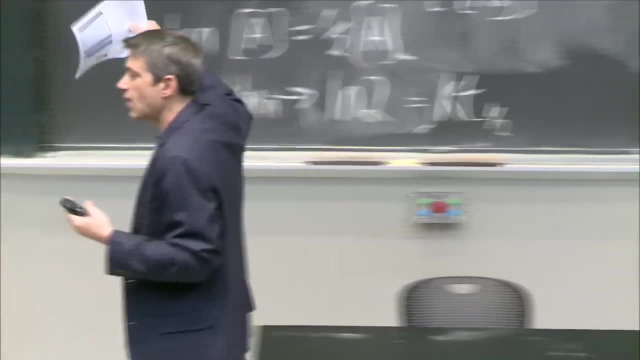 And that leads to the reaction. So you can imagine now. it's not just how fast they're moving, It's how fast they're moving, Which is what the exponent tells us. It's more complicated, And this is called the frequency factor. 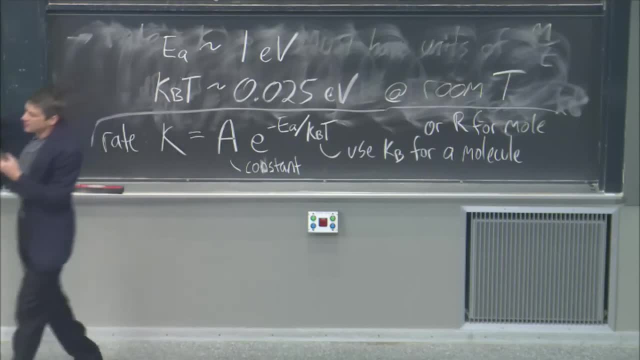 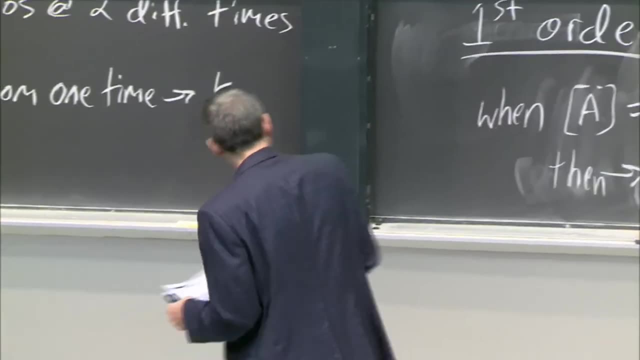 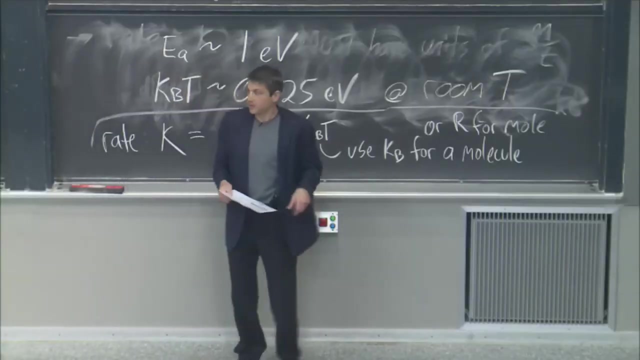 because it's sort of all these complicated effects rolled into the frequency of the collision being right, not just the temperature, And so this gives us the temperature dependence of the rate constant. This gives us the temperature dependence of the rate constant, which is very important. 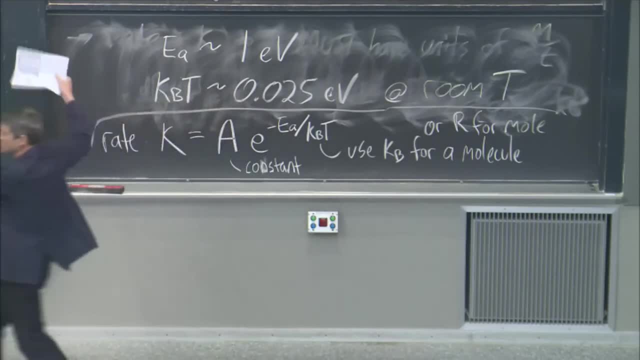 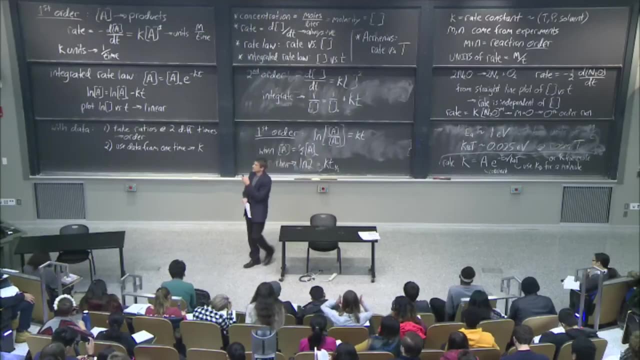 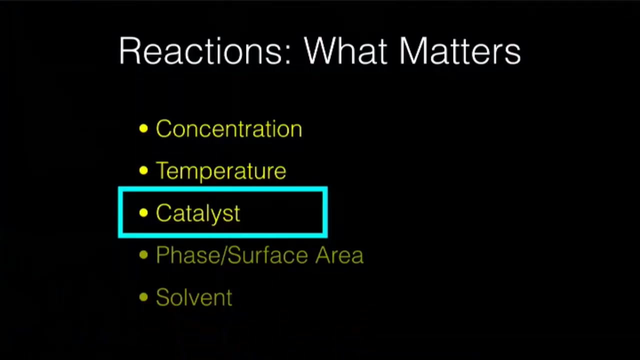 This is not time, This is temperature. This is a different thing than everything else we talked about here, which involved time dependence. That's temperature dependence. OK, And finally, the last thing- and just to show you this is my very last point- is that, just like before, 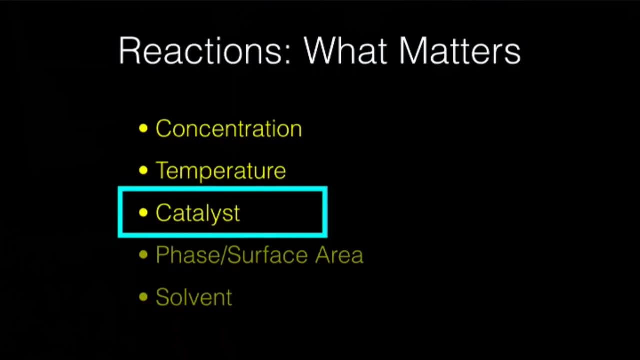 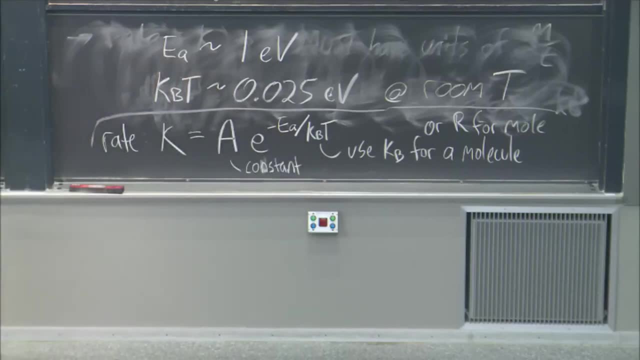 if I wanted to run a reaction and make it go faster one way, just like with semiconductors, I would increase the temperature, But I don't want to run my phone at 600 Kelvin. So what do we do? We use chemistry. 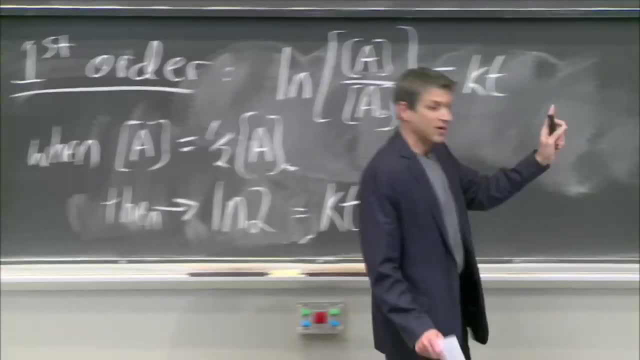 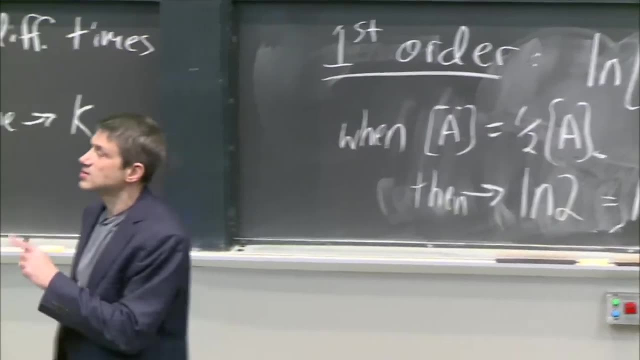 I may have reactions that I want to run a lot faster. In fact I very often do. And what do I do? I use chemistry, And those are called catalysts. What a catalyst does, and this picture shows it in the context of collision theory. 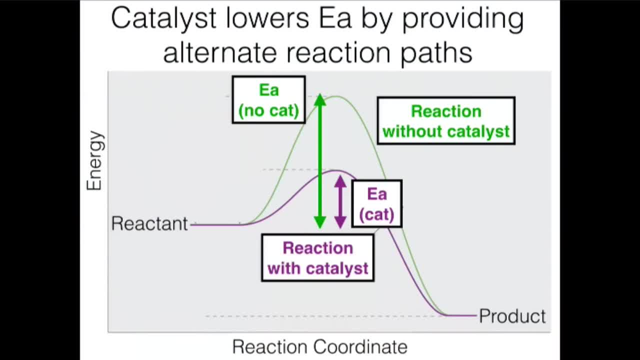 I've got these barriers I'm trying to get over Here. it's flipped, It doesn't matter. There's a barrier, So the reactant is higher than the product, It's OK. There's still a barrier that I have to overcome.